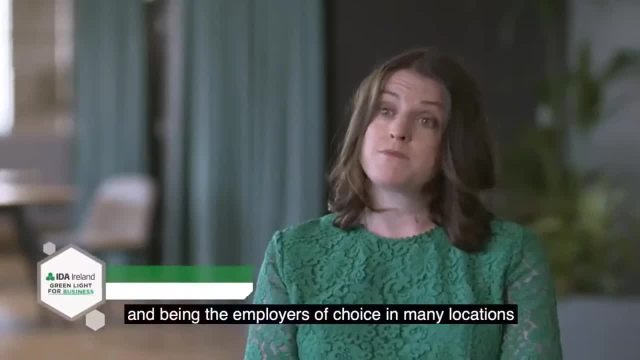 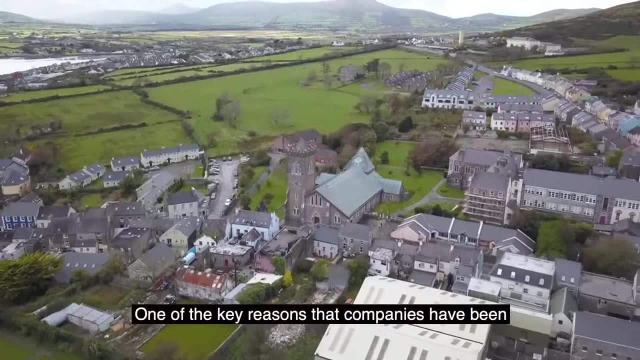 So they make a major contribution, both in terms of jobs and being the employers of choice in many locations around the country, but also the local contribution to the communities in which they're based, One of the key reasons that companies have been so successful in regional locations around the country. 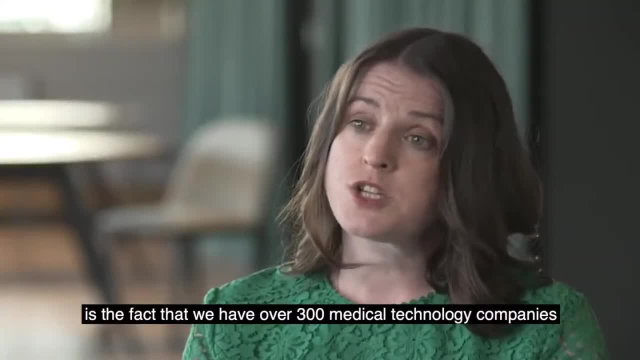 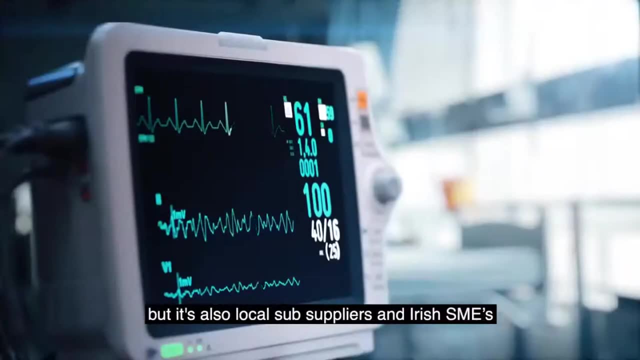 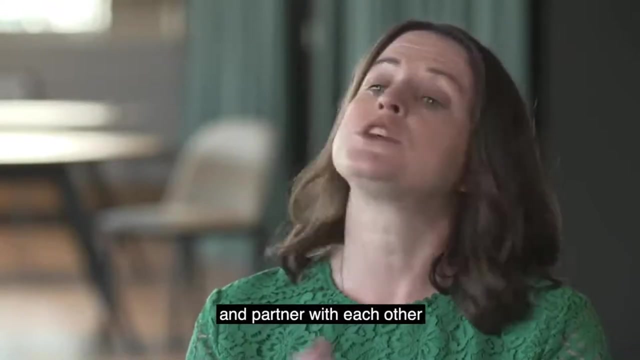 is the fact that we've over 300 medical technology companies here in Ireland and it's a very close-knit. It's not just major OEMs and manufacturing products here, but it's also local sub-suppliers and Irish SMEs, And it's the way those companies collaborate and partner with each other, to everything from supply of materials. 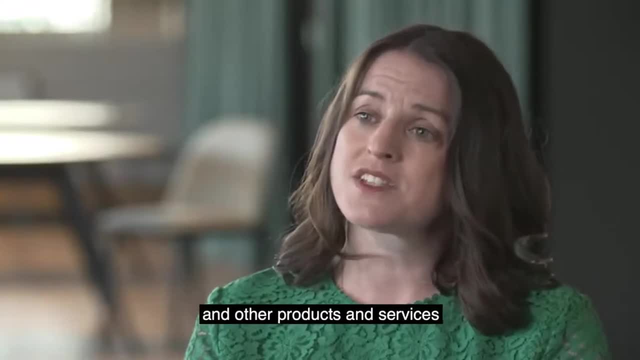 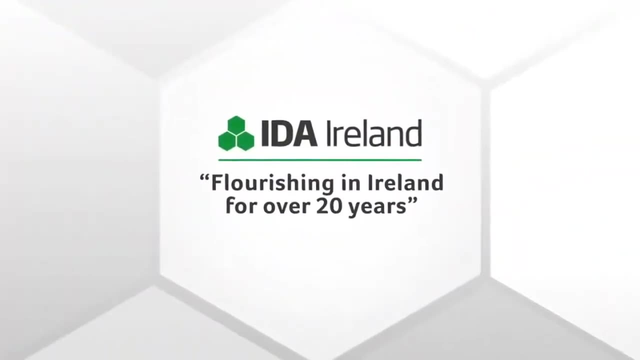 engineering services and other products and services. that really helps the medical technology sector to thrive here. What is the role of Striker in the future? What is the role of Striker in the future? If you look at Striker in Ireland, it's a very close-knit sector. 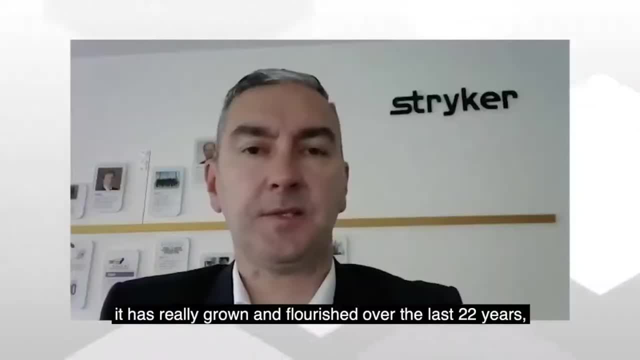 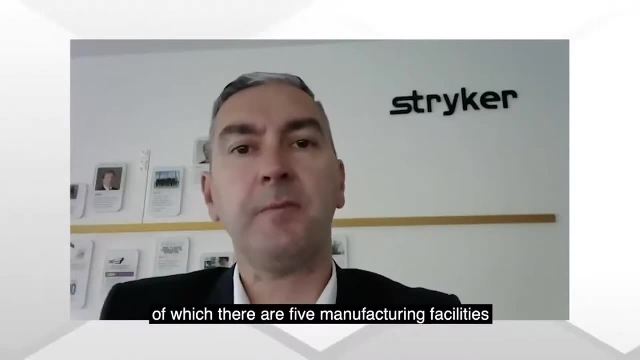 If you look at Striker in Ireland, it's a very close-knit sector And it has really grown and flourished over the last 22 years since we opened our first facility in 1998.. And our facilities in Ireland, of which there are five manufacturing facilities and one global innovation centre. 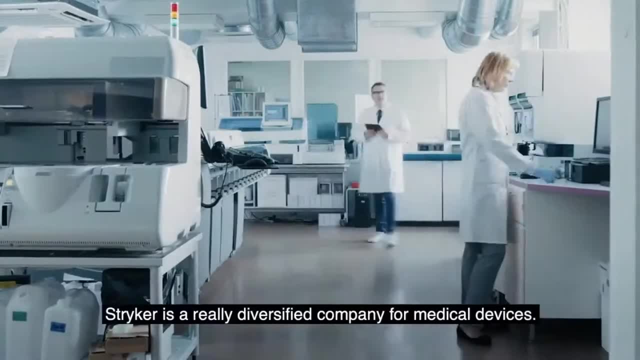 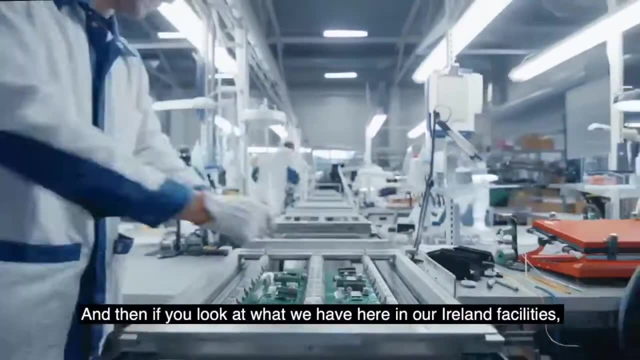 are somewhat a microcosm of Striker. Striker is a really diversified company for medical devices. We have a very wide portfolio And if you look at what we have here in our Ireland facilities, we make things from knee implants or knee prosthetics. 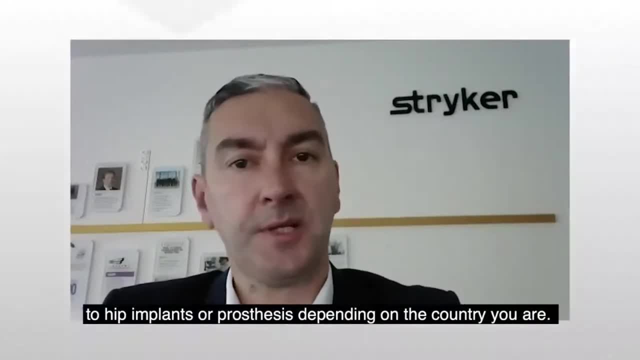 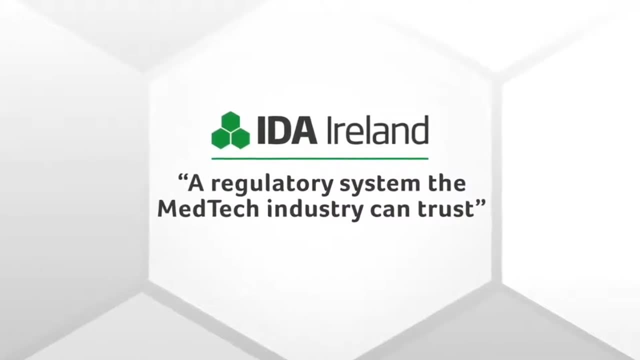 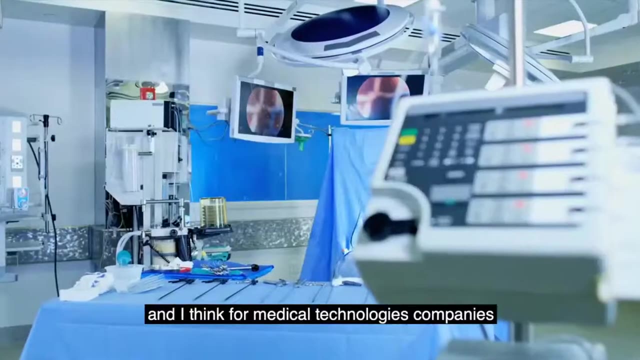 knee prostheses to hip implants or prostheses, depending on the country you are. Why does Ireland have such a massive training time? Well, Ireland has a great reputation in terms of its regulatory regime here and, I think, for medical technology companies. 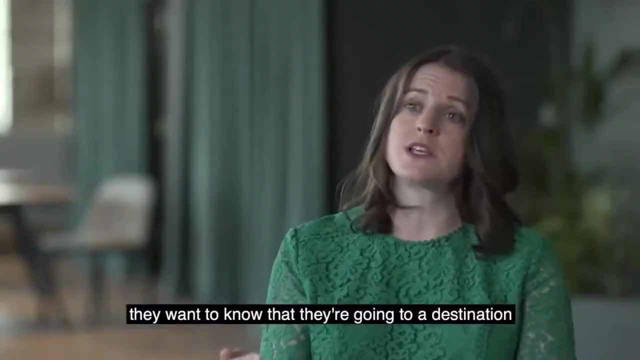 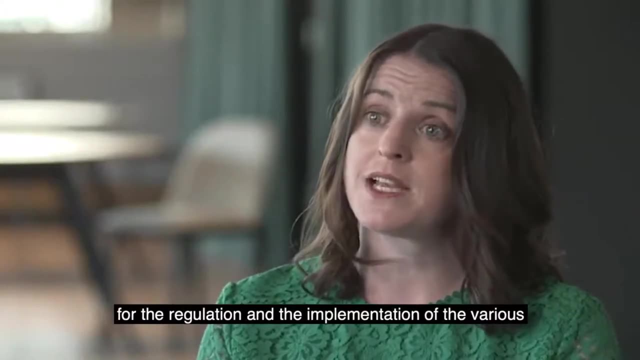 in such a highly regulated environment. they want to know that they are going to a destination that has an exemplary track record in this space. So the Health Products Regulatory Authority here is responsible for the regulation, the implementation of the various EU directives around medical devices, and it takes a very 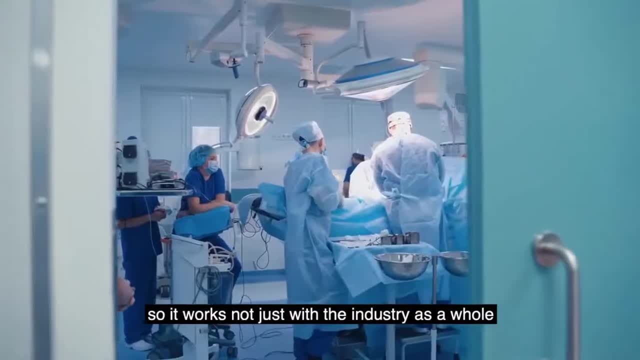 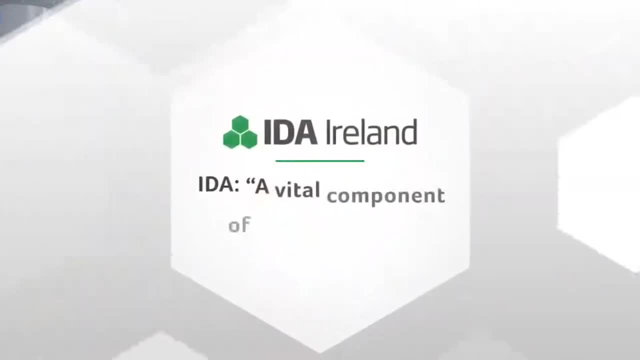 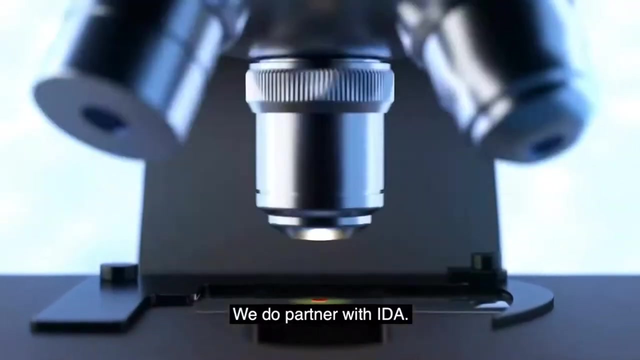 pragmatic approach to doing that. so it works not just with the industry as a whole but with individual companies around, helping them when they get set up to ensure that they've all of their systems placed to be compliant. we do partner with IDA. they are another vital component of that. 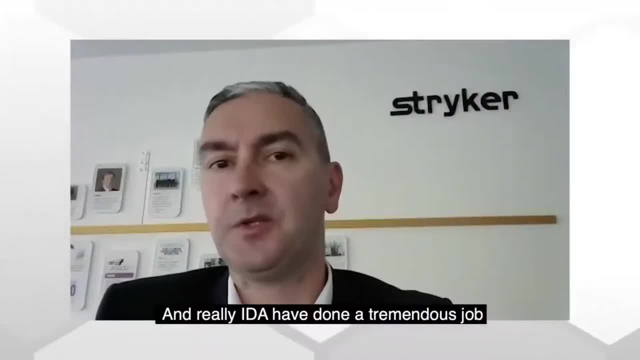 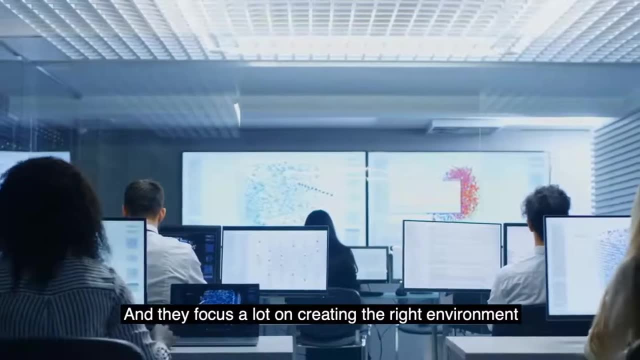 ecosystem and that partnership and really IDA have done a tremendous job in helping create that ecosystem- that word I keep using- and they focus a lot on creating the right environment for companies like Stryker to flourish and also are very interested and cognizant of what are the things we 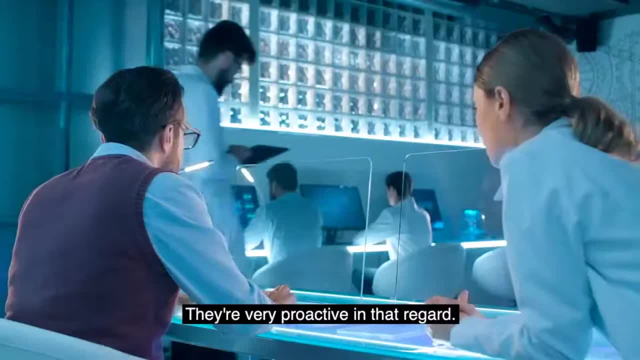 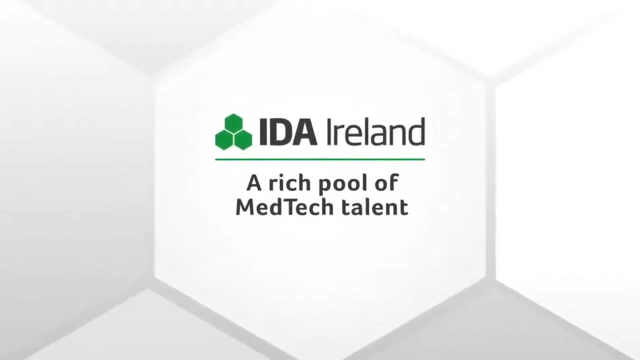 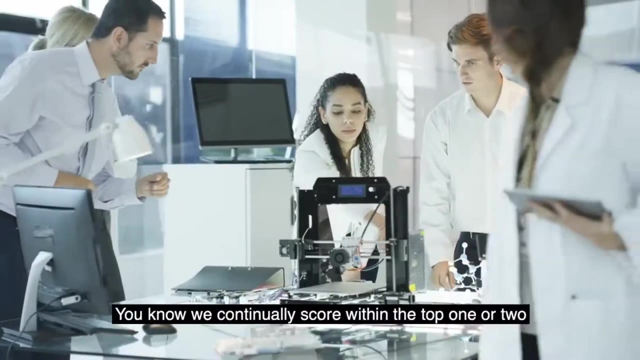 need, or what are the supports, to continue to be successful. you know they're very proactive in that regard. so the Irish workforce has a great reputation for flexibility and adaptability. you know we continually score within the top one or two countries in the world for how we adapt. 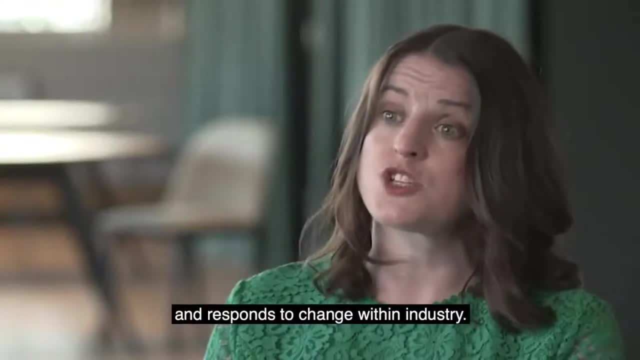 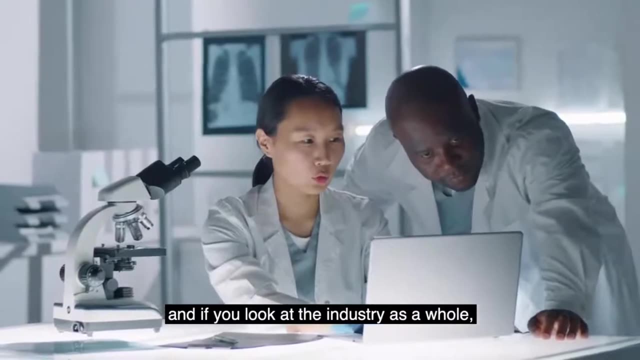 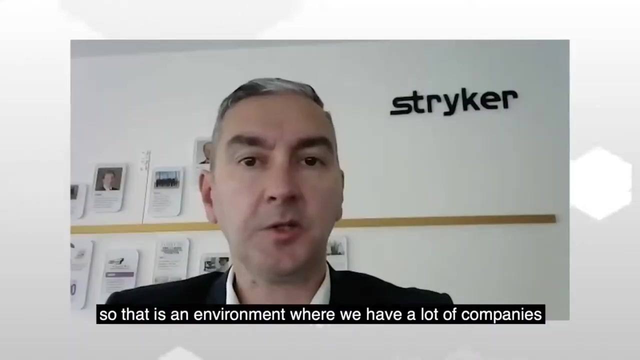 as a nation and how our workforce adapts and responds to change within industry. we're part of a very powerful ecosystem in Ireland at the moment and if you look at the industry as a whole, there are nine of the top 10 medical devices located in Ireland, or 17 of the top 20. so that is. 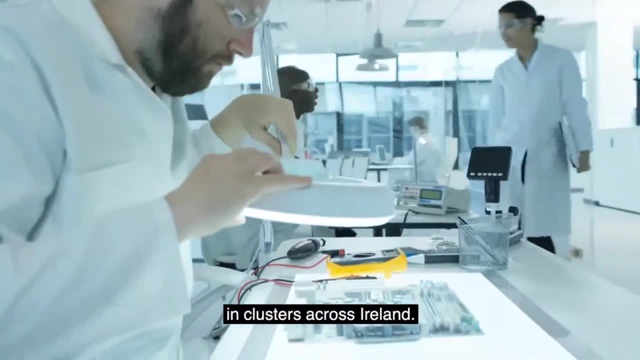 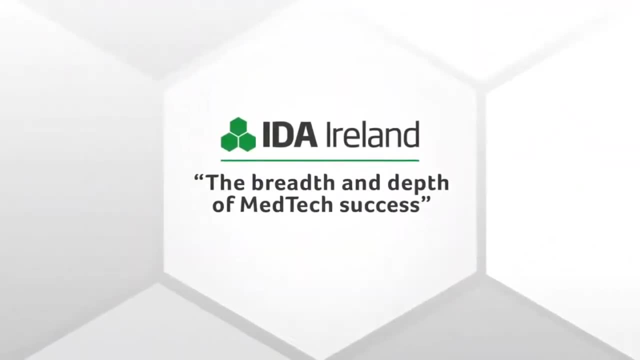 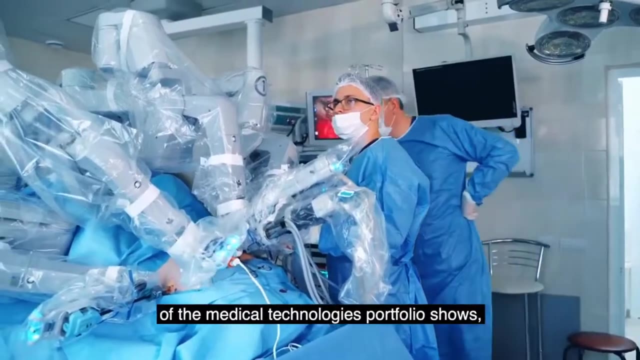 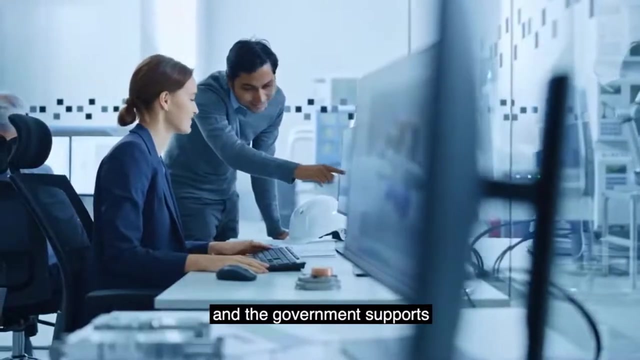 an environment where we have a lot of companies in clusters across Ireland, so really we have a rich pool of talent to really work with. as the breadth and depth of the medical technologies portfolio shows, Ireland has the talent pool, the ecosystem, the business and regulatory environment and the government supports. 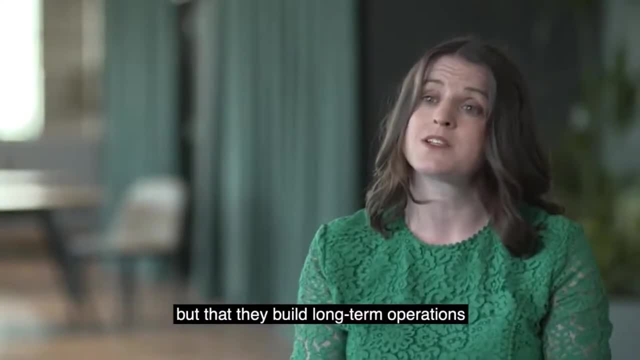 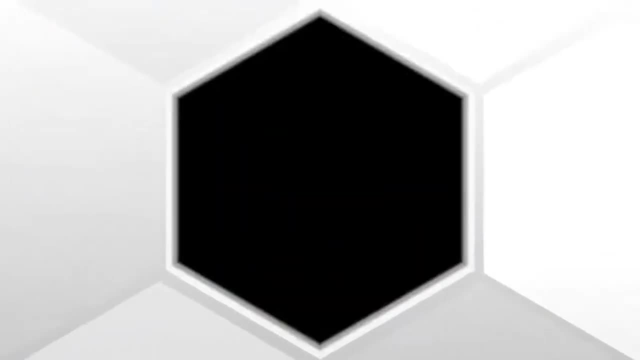 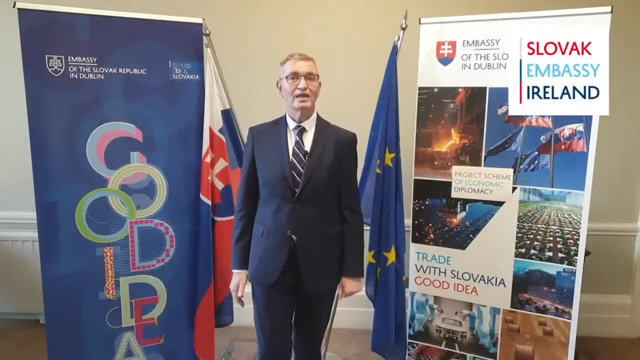 to ensure the companies not just have a successful start here, but that they build long-term operations that add value for their businesses. good morning, ladies and gentlemen. I am more than happy to welcome all of you at the launch of the Slovak Island Health Pitch organized by the embassy of the Slovak Republic in Dublin. 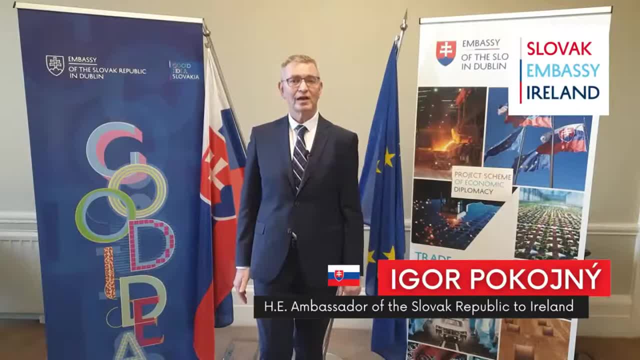 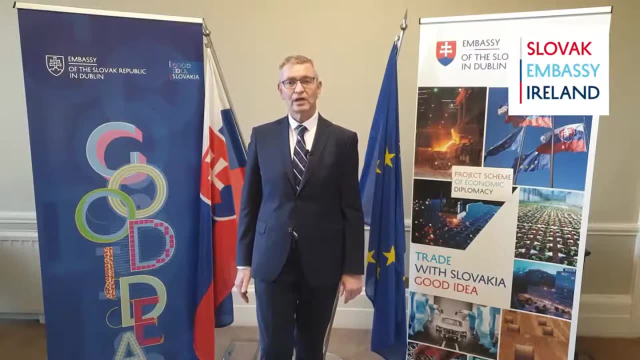 Slovak Honorary Council in Galway and the Slovak Investment and Trade Development Agency. I am delighted to see so many companies joining us from Slovakia and Ireland. until now, trade between Slovakia and Ireland has been almost entirely represented by multinational corporations. however, we are witnessing a dynamic change of narrative regarding the very foundation of our 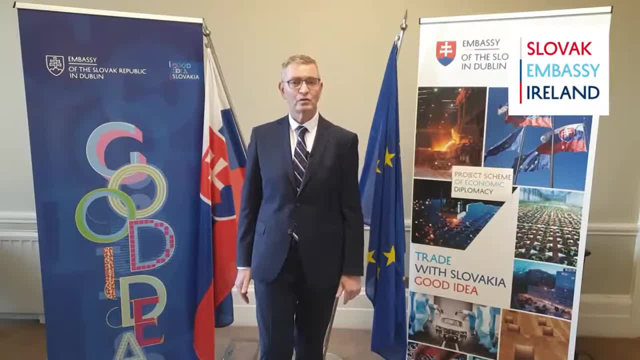 economies as they pivot from traditional industries to innovative medical solutions. therefore, it is the ambition of the health pitch to project small and medium enterprises on a pan-European stage. that will advance their chances of finding new markets to network, connect and succeed in the future. I am delighted to welcome state secretary. 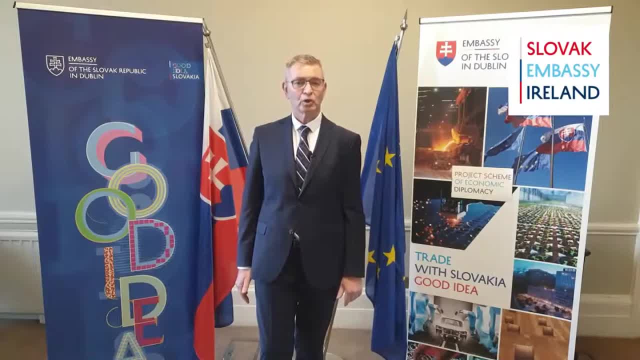 of the Ministry of Foreign and European Affairs of the Slovak Republic, Ingrid Brodsková, state minister of the health department of Ireland and rabbi and director general of the Slovak Investment and Trade Development Agency, Robert Cimoncic, state secretary. the floor is yours. 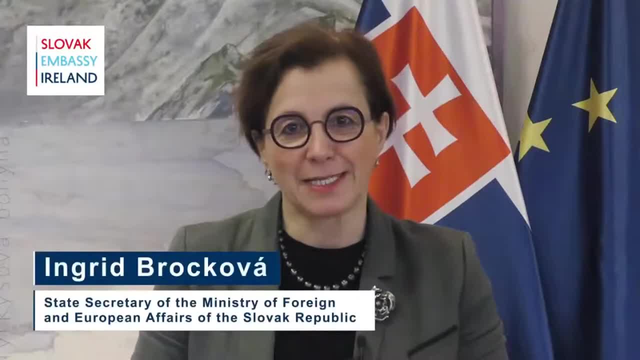 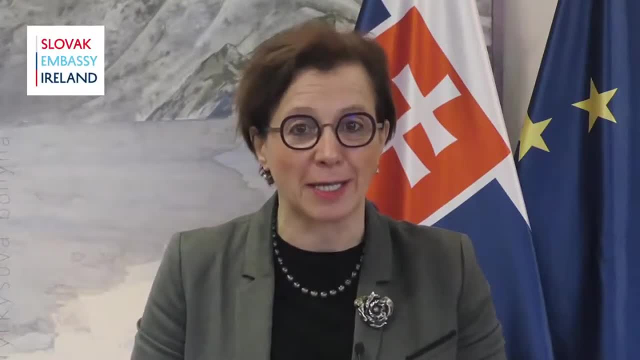 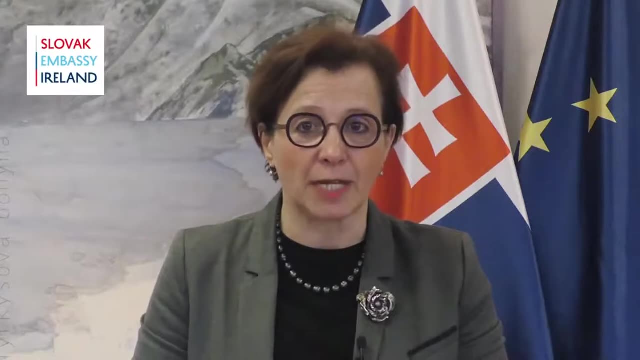 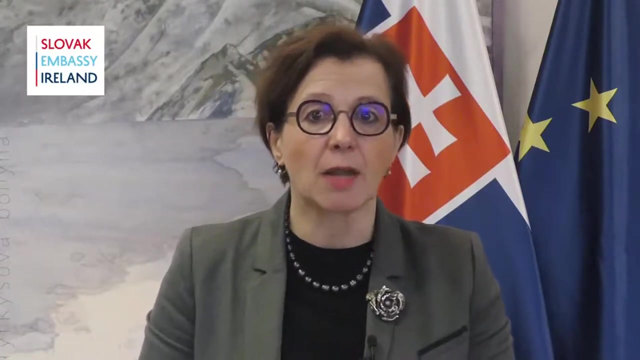 ladies and gentlemen, good morning to all of you. it is actually the second pitch day in a row, so let me welcoming you on the traditional Slovak Ireland health pitch. as you know, we are in the middle of dynamic change regarding the very foundations of our economies, from traditional industries to innovative ecosystems. Slovakia has been among. 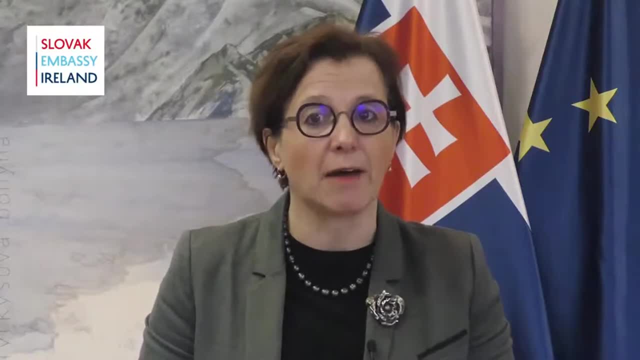 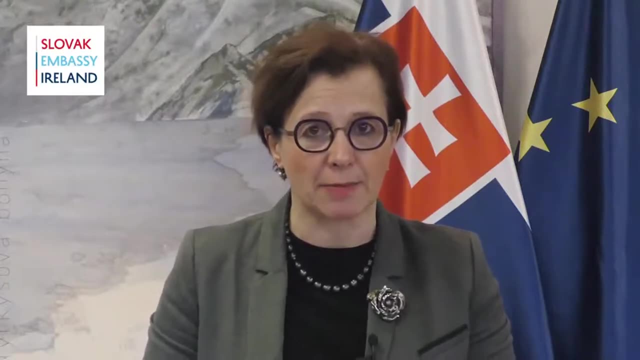 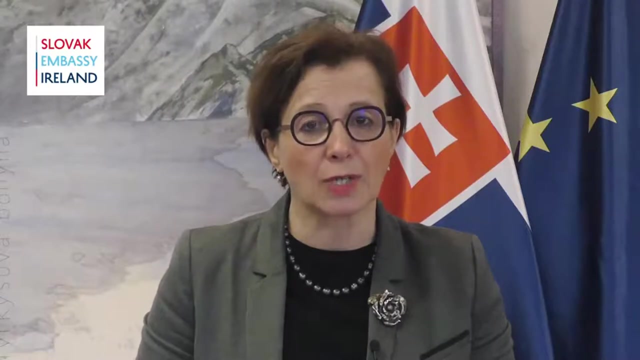 the fastest growing EU economies in recent years. however, we need to maximize our innovation potential and translate ideas into practical steps. I firmly believe that innovation is not just a key driver of competitiveness, but also critical to solve the pressing global challenges like pandemics. it has to be the private and public sector working together on one common goal. 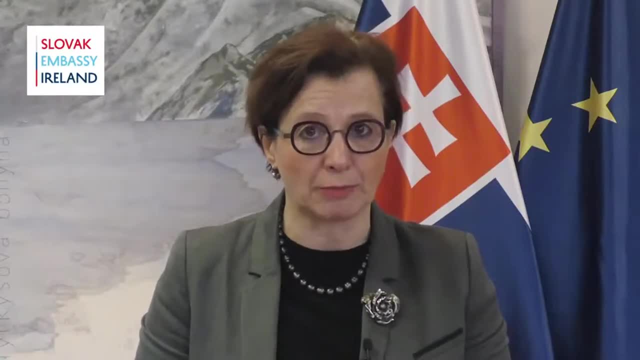 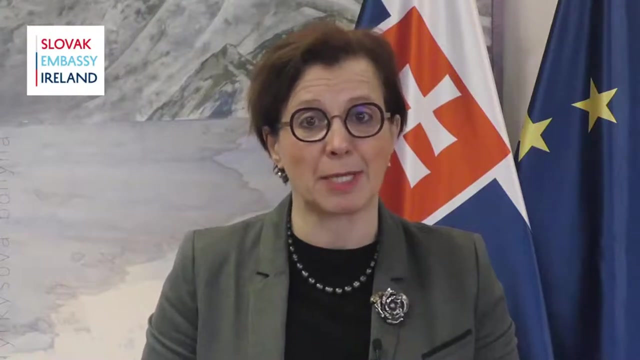 to unlock the innovation potential through collaboration. we at the ministry of foreign and European affairs take this job seriously. economic diplomacy acts as an accelerator for the Slovak companies with export potential. thus all these initiatives that have been carried out in this year. All the participants of today's event were carefully chosen and will surely introduce 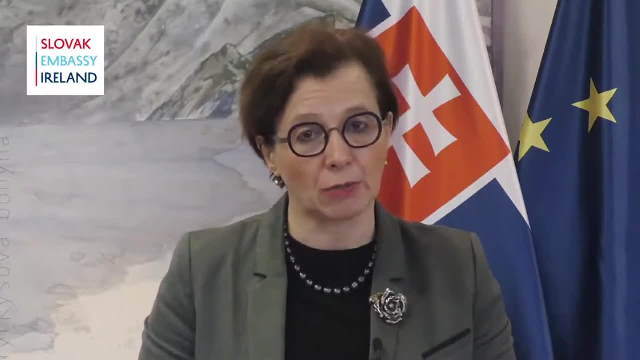 you the most valuable content focused on their unique solutions. Slovakia and Ireland have many things in common: Desire for the invention and the hard work are definitely part of them. So let's use this opportunity and boost the Slovak Irish economic cooperation in a very topical sector of today. 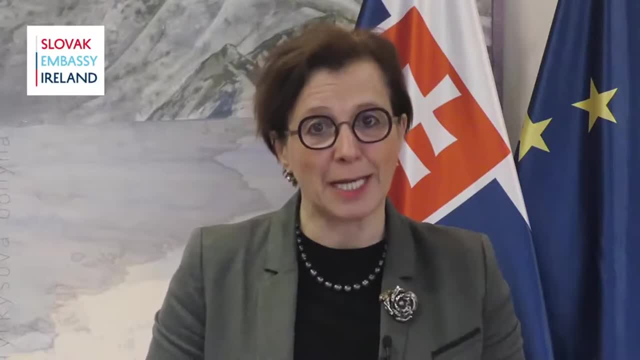 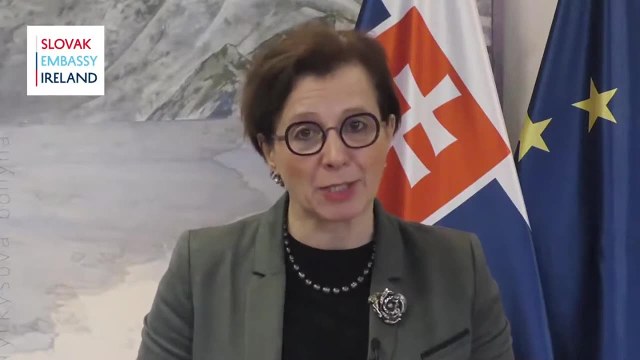 Let me say thank you to our embassy in Dublin and our Honorary Consul in Galway, Mrs Lorraine Higgins, for organizing today's event. I really appreciate the support and the presence of the Minister of State, Mrs Mary Butler. 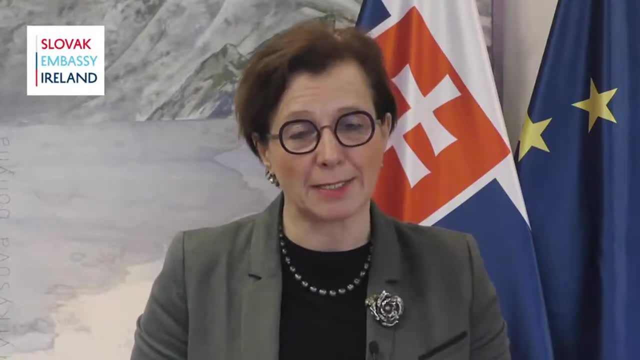 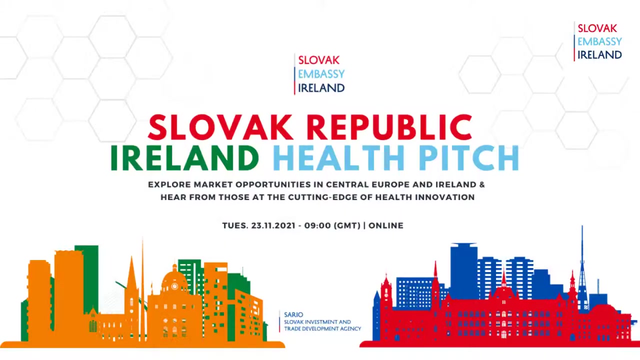 Although business travel is still quite demanding at this moment. let's hope that the return to normalcy will resume soon and you will be able to follow up on your expansion plans in person. I wish you constructive meetings and good luck. Good morning everyone. 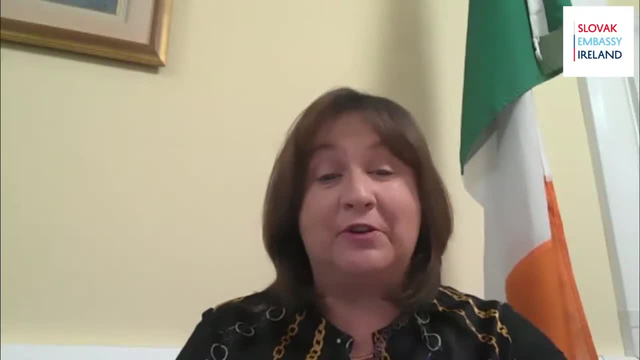 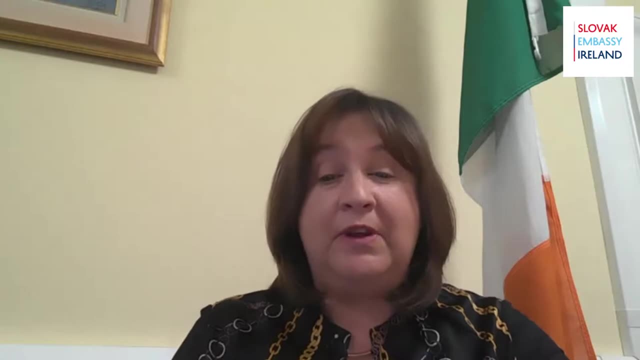 Firstly, I want to thank you for inviting me to be part of the inaugural Slovak Ireland Health Pitch event this morning, particularly the Ambassador and State Secretary, whom we just heard from. It's fantastic to be able to say that Ireland has developed a rich landscape of life sciences. 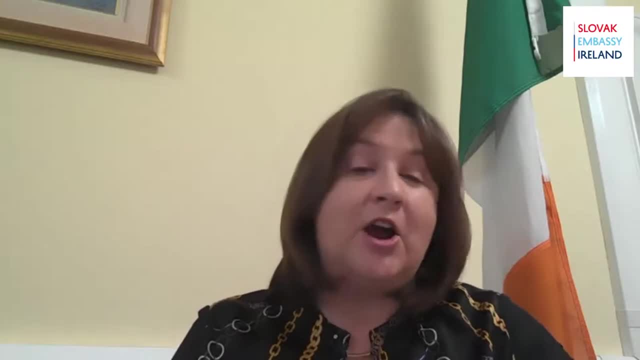 business and healthcare. We have a large network of highly innovative indigenous companies, large well established FDI multinationals, a continually developing world-class research base and a strong industry focused clinical community. In this context, Ireland's event is a timely one, as well as highlighting potential new 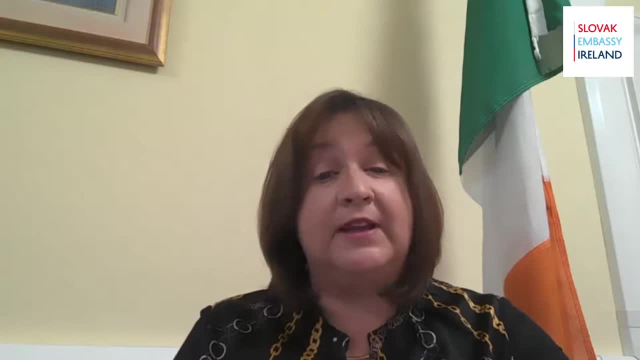 market opportunities. Today's pitch event brings to the fore some of the in-depth knowledge and expertise across key sectors of medtech, pharma and healthcare. Thank you very much. pharma, biopharma and technology in both Slovak and Irish companies. 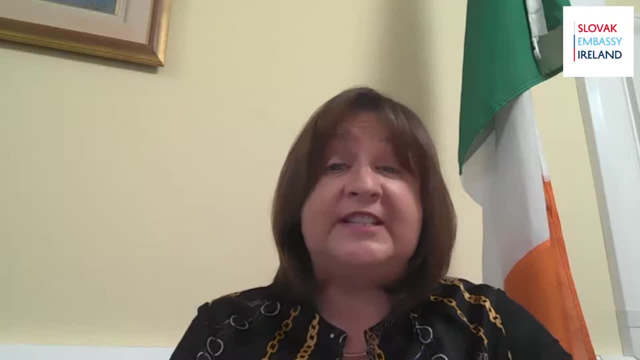 The life sciences industry in Ireland employs over 78,000 people in activities ranging from manufacturing, R&D, supply change and a variety of EMEA and global services. The sector accounts for 83.7 billion in exports from Ireland. In the last 10 years there has been a significant ramp up in biologics. 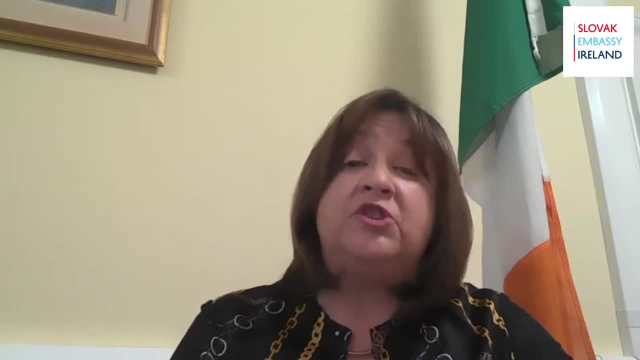 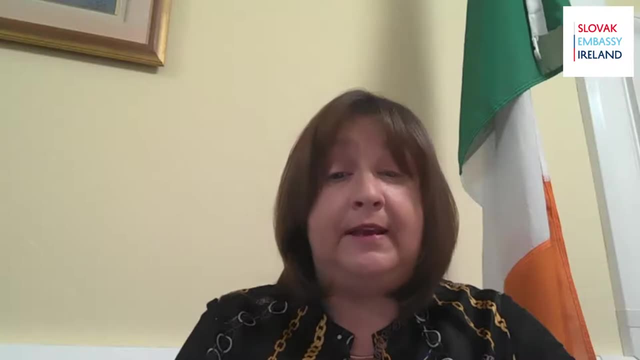 manufacturing in Ireland, adding to our traditional manufacturing base in small molecule manufacturing. Over 10 billion in new investment has been committed in the last decade for new biotech manufacturing facilities. in both drug substance and drug product, Ireland has an extremely regulatory compliance record. 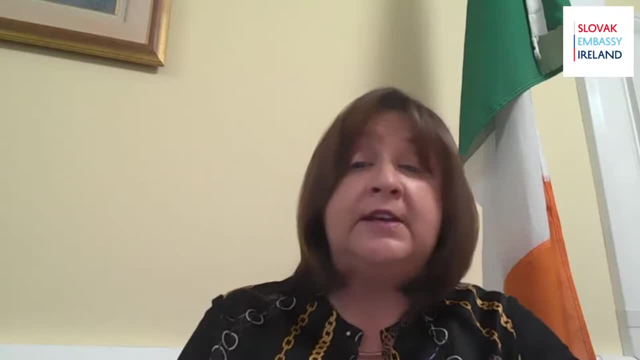 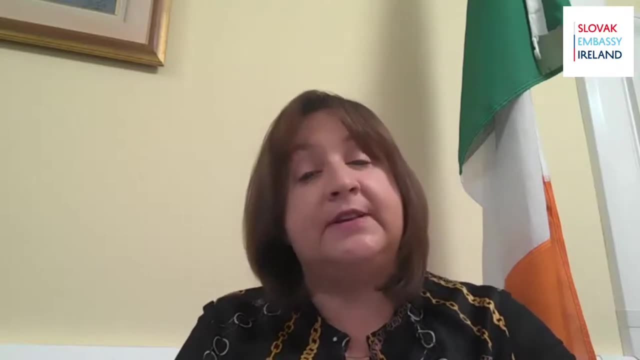 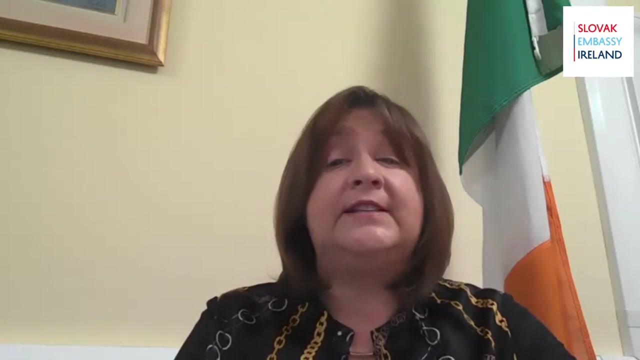 strong government support for R&D and zero defect biopharma manufacturing excellence- All factors which have contributed to these recent wave of investment in biotech facilities. The Disruptive Technologies Innovation Fund, or the DTIF, is a 500 million euro fund established in 2018 as part of the National Development Plan. 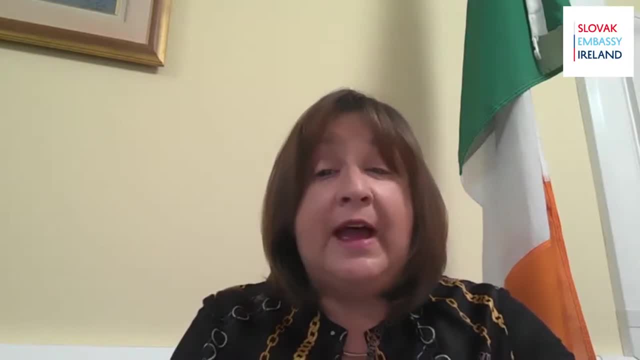 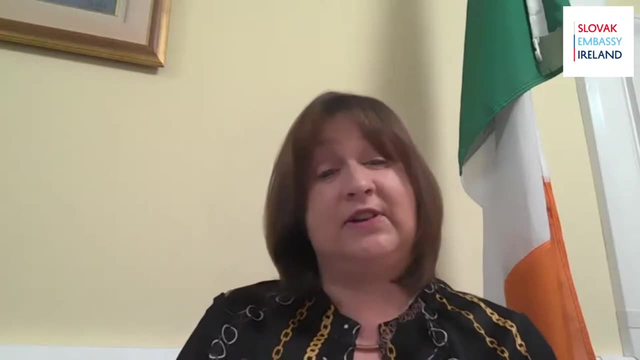 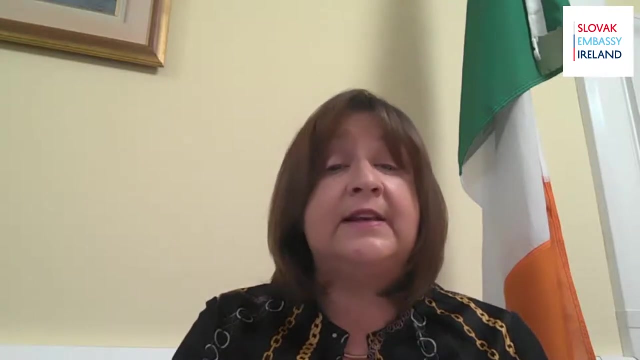 And its aim is to stimulate disruptive innovation and collaboration between Ireland's world-class research and base industry. To date, 72 projects have been funded, with a large proportion of those in life sciences research priority area, largely due to the healthy and innovative ecosystem in that sector in Ireland. 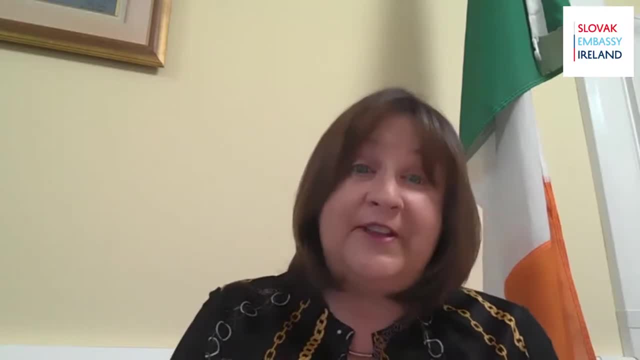 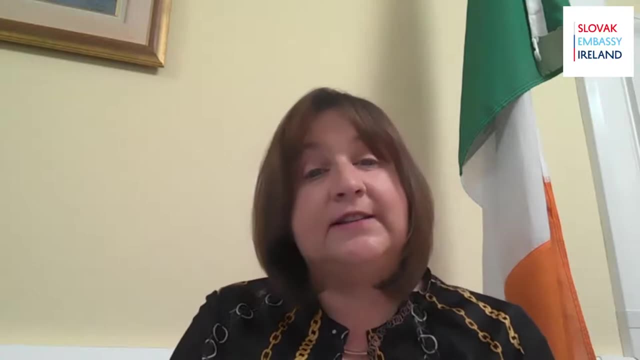 A fourth DTIF call was launched on the 8th of November 2021.. To conclude, Ireland is recognized as the world's leading industry in biotech. As a major center of excellence in the medical and technology sector, the Irish cluster is on par with some of the world's leading medtech clusters. 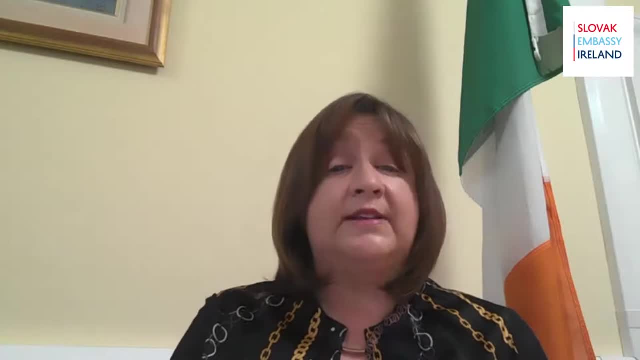 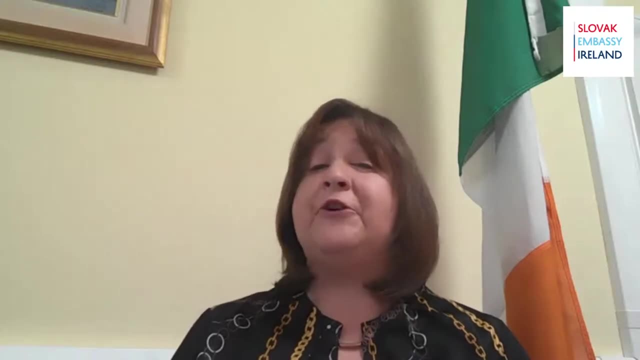 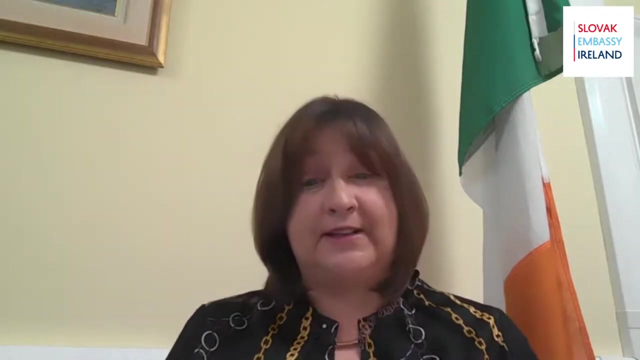 such as those in Massachusetts and Minnesota in the US We are seeing here today demonstrates the importance of cross European partnership, allowing us all to gain further insight into the ongoing developments both here in Ireland and Slovakia. I would like to wish everyone the best of luck and I look forward to the continued cooperation across borders. 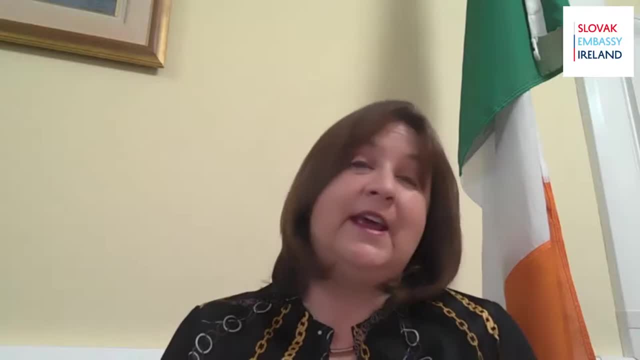 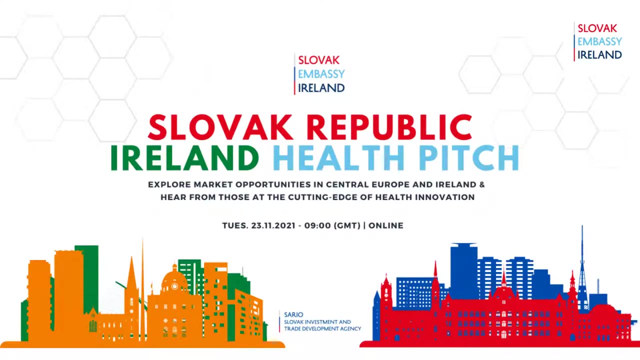 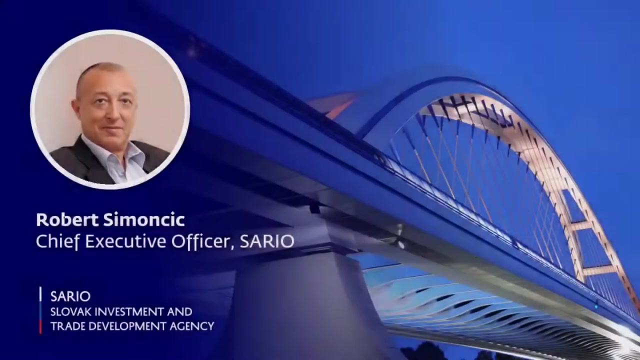 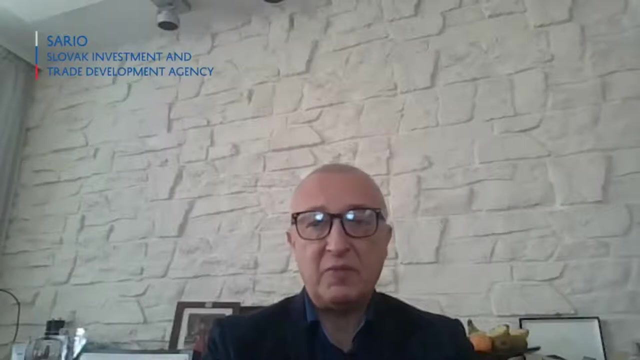 in the development and support of emerging technologies. Thank you, Ladies and gentlemen. on behalf of the Slovak Investment and Trade Development Agency, SARIO, it is my great pleasure and an honor to be a part of this event. I'm very pleased that after a half a year there is another event of Irish and Slovak companies. 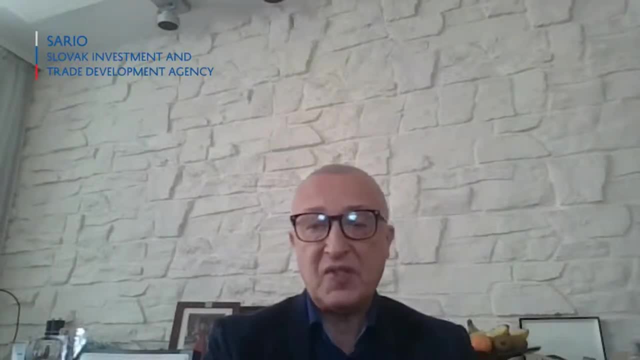 to have an opportunity to present their skills, products and achievements. SARIO, in the last 20 years, has brought billions of US dollars worth of high quality investments to Slovakia, created tens of thousands of jobs, helped hundreds of Slovak companies to realize their full potential abroad. 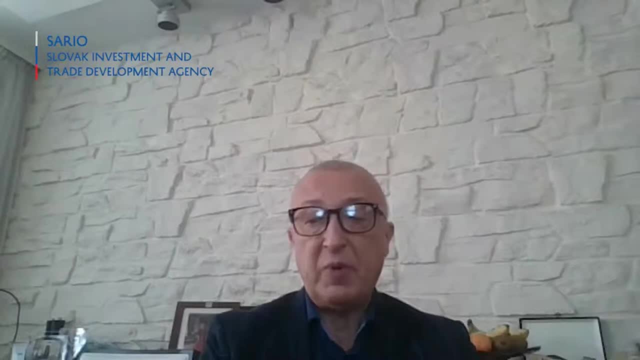 Because of this, we are very glad that we can participate in this event. An event like this is a great opportunity for all participants to present their new ideas and solutions. Pharmaceutical and health care sector in general has got a strong tradition in Slovakia. The first manufacturers in this sector started their production in the early 50s. 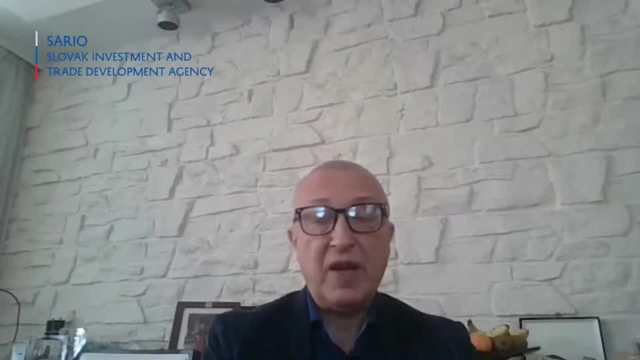 of the 20th century. Actually, we have now almost 200 companies operating in this field and the total exports from this field from Slovakia is close to half a billion euros. Actually, the sector employs very qualified and skilled workforce. Nevertheless, the volume of international trade in this area, 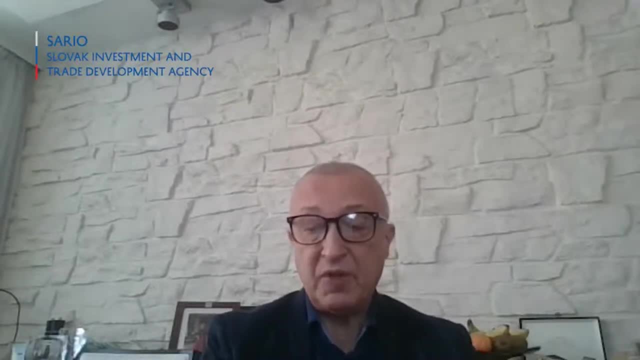 is kind of low in terms of Slovakia and Ireland, And we hope that this event will support that and support more of an international cooperation. I'm very pleased to hear a lot of interesting companies from both countries are presenting today, While the first event was focused on startups and innovative IT companies. 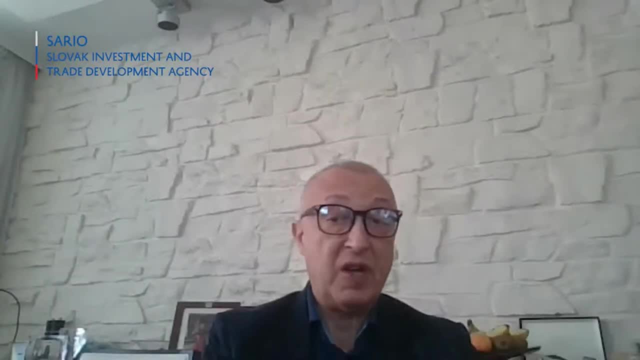 this time we'll see the companies from the health care sector. a number of our Slovak companies in this field are very successful abroad as they are offering very competitive products and services. During COVID-19,, they went through a speedy innovation and improvement of their products, and services became even more attractive for foreign markets. 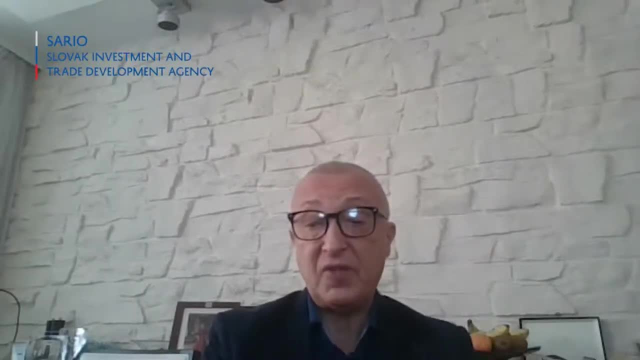 During today's pitch, you will see 12 very innovative Slovak companies with their portfolio of pharmaceutical products and devices. They also offer unique software solutions And, in addition, new innovative diagnostic methods will be also presented. I hope that our event will be inspiring. 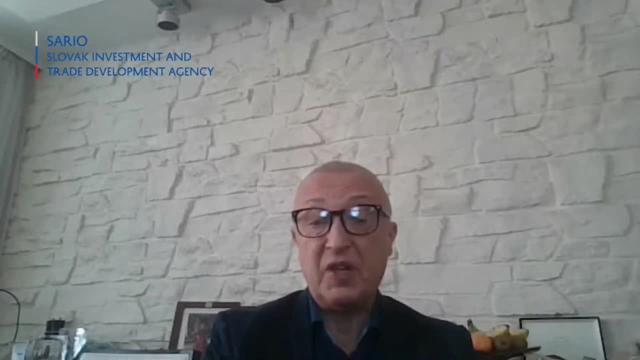 opens new perspectives and potentially brings a lot of new opportunities for future international cooperation and business. I would like to take this opportunity to express my sincere thanks to the Slovak Embassy in Dublin, honorary consulate of the Slovak Republic in Galway, to our Sario team and all our partners. 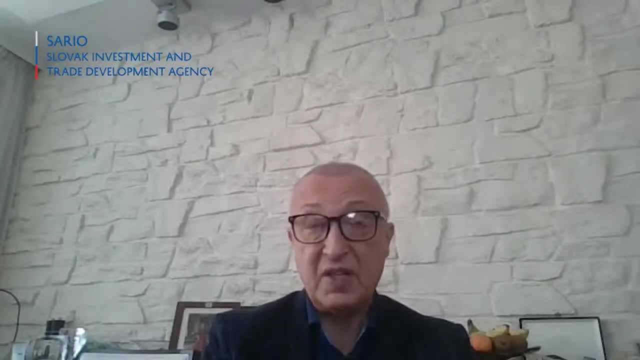 all of which contributed to this great event. Finally, I would like to say good luck to all participants in this health care pitch, And I hope that all of the companies involved will find something new, either new business relationship, learn something new how to operate in future. 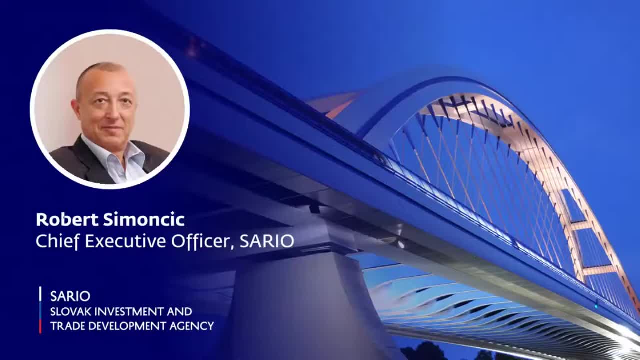 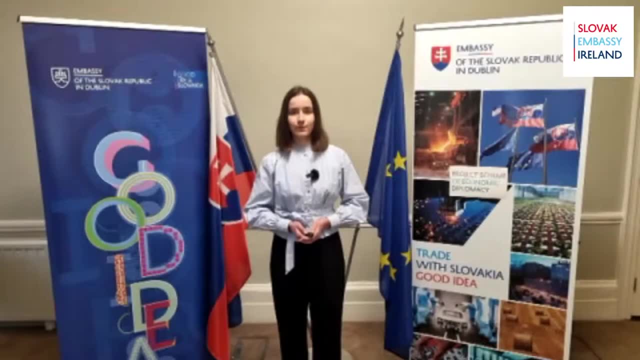 Thank you very much and good luck again. Thank you, The first presenter is Mrs Mirjam Škulinková from the Slovak company MB. MB created a simple and intuitive outpatient software for general practitioners, pediatricians and specialists, available anytime and anywhere. 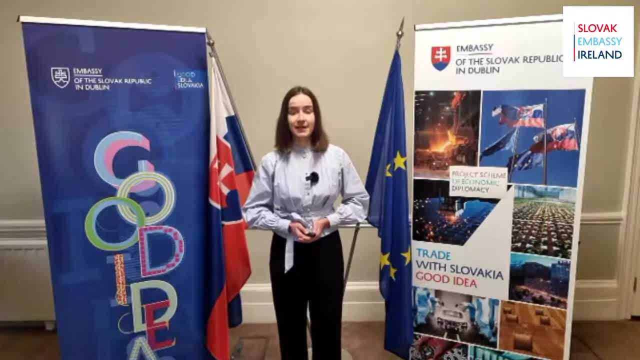 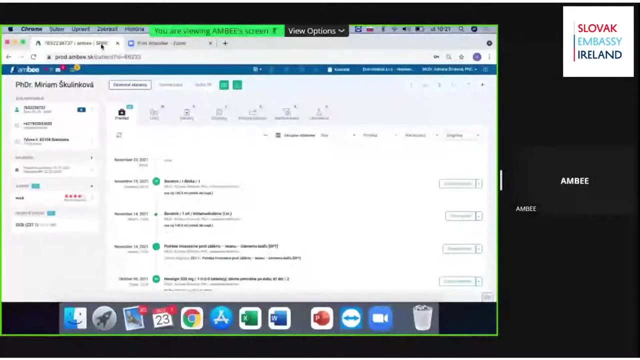 The company developed it together with doctors and nurses. It depends on their opinion. MB is supposed to help them and assist in processing the daily agenda. Hi hello, Thank you very much for your time. My name is Mirjam Škulinková. 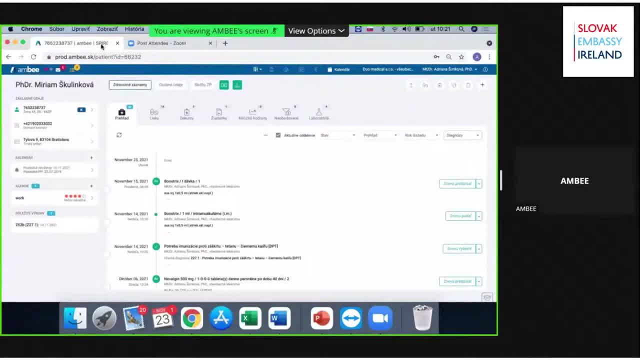 I'm from Slovakia. We would like to present very briefly our system. We call it our baby because basically cooperation with our doctors and with our nurses. we created this system. Our doctors and the nurses showed us and taught us and told us what is necessary. 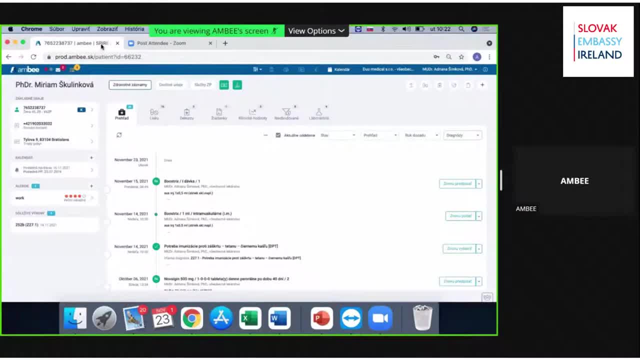 for the daily work. So in the last three years we just created this, this, this product. Sorry, I was just reading the message Right, So hold on. If you look at our system, our system is web based, So if you go back to the main page you see all the patients you have. 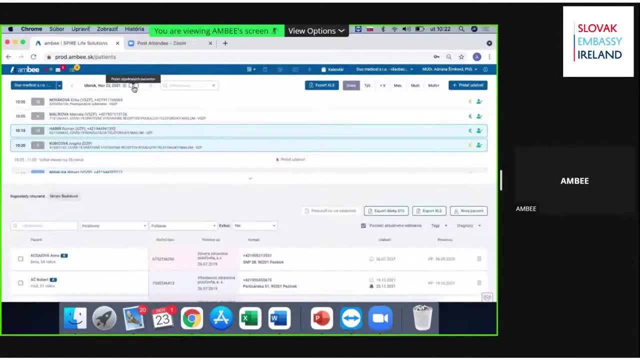 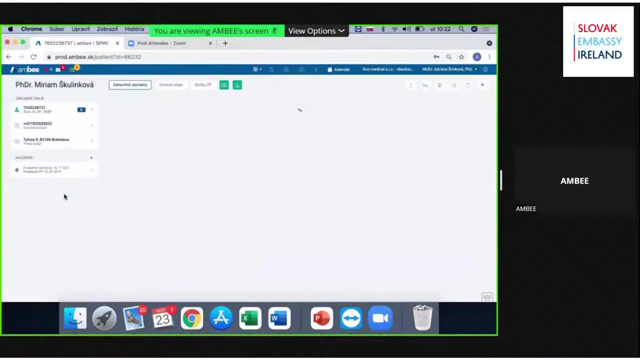 You can see all the patients that the doctor has planned for today If you want patients. if you click on your selected patients, you see the health report. Your patient is the. Is he in this hotel? It seems like the connection is very slow, very, very low, slow. 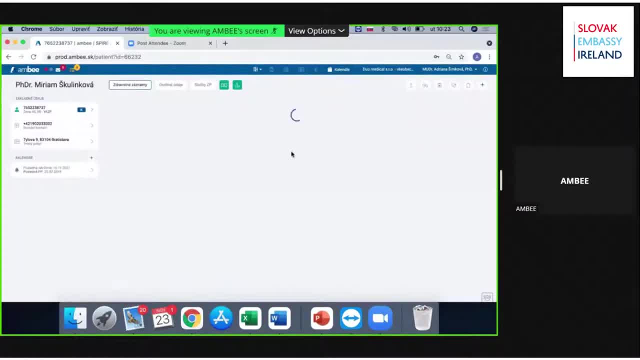 It's unstable. Give me one second. OK, so I'll just go back and I click on on the patient card. So on the left hand corner you see my name as a patient name, my data, my contact numbers, my address. then you can actually check any allergies or any. 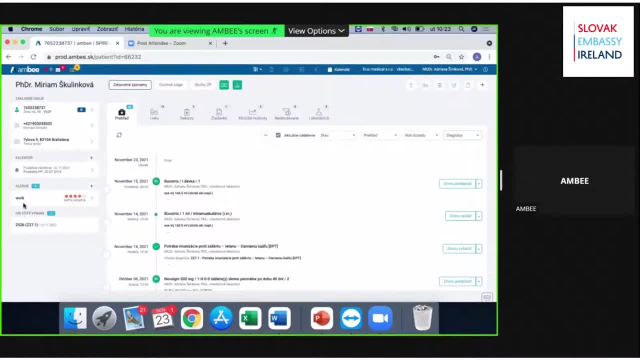 necessary information you want to keep on your patient, So you have sticky notes. You can make your own sticky notes in your system. Also, you can see the most important procedures or whatever you've executed on your patient. You can see it on your on your left hand side. 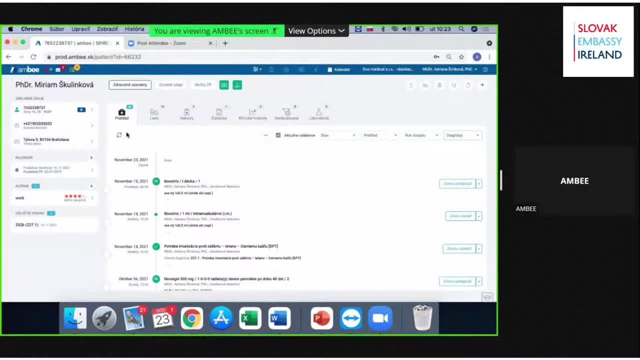 Then what we've created is that we have this one little electronic health record, like a file, with all information related to your patient, including the prescriptions, including the health The record. Tell me, what does it do for you? What is your doctor's job? 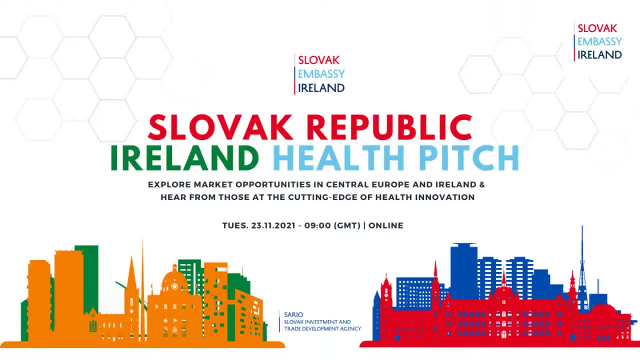 What are the changes? They can tell you anything. Does it help you? I think it does. It's a smiley face. I think it does. I think my, my doctor's office is a bit different. I think it's a bit more. 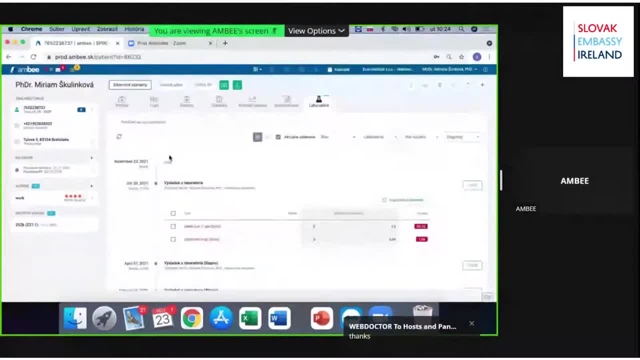 simple and it's a little bit strange, but it's a bit more realistic And I think it's just a little bit more amazing to see what they're doing with the stuff they can do. I can see that some patients do have a distinct 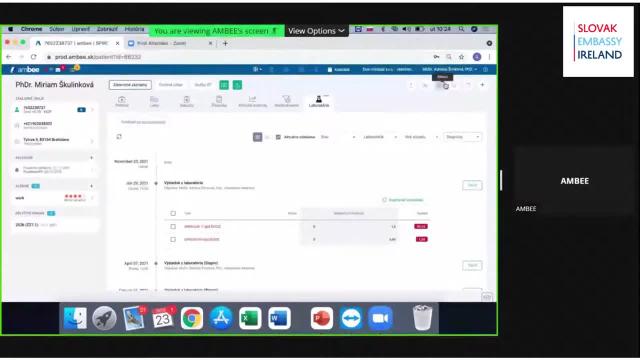 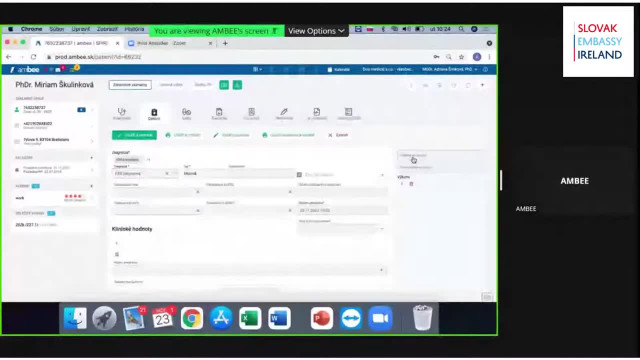 problem with their risk management system- And some patients do have a bit of a risk management system- The main trends into the information or insurance companies and recording those specific executed services that the doctor executed on the patient. We have prepared loads of templates with loads of. 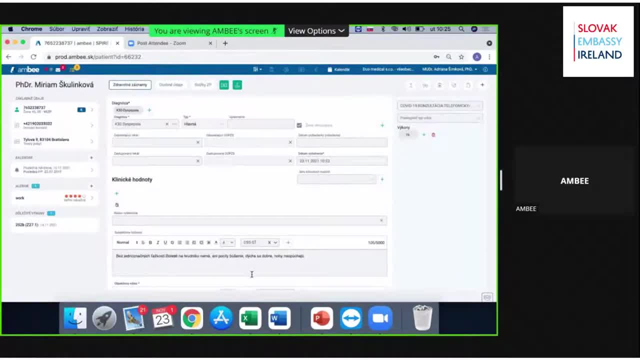 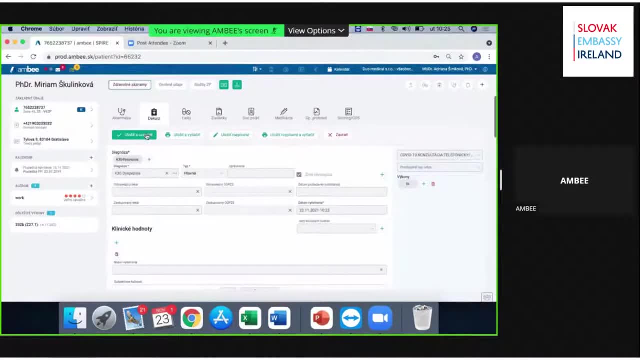 information. so the doctor doesn't have to rewrite every single medical record or prescription one by one, but they can use the templates. The moment we click on our save and close, the record is directly sent to the national health system, Also so integrated to the contact of your employer. you have to contact social 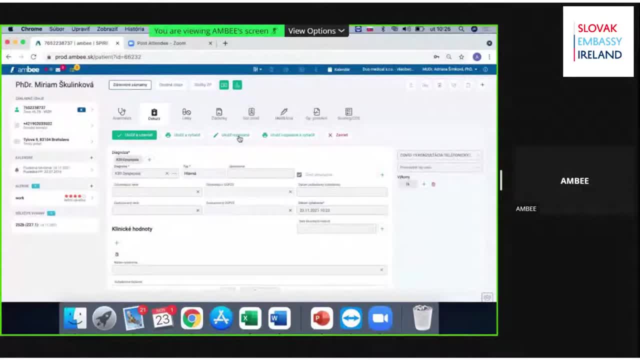 securities, So it's also directed through another little button. Also, we do loads of little scoring for our patients in terms of, for example, colon cancer or certification of of stroke if the patient is at risk to get any serious health problems in future. for 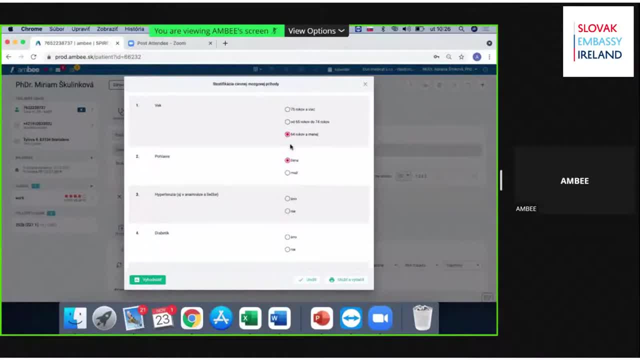 example, we click on age, it's directly crossed sex of the patient- and then you just select: if the patient has hypertension, if the patient has diabetes mellitus, et cetera, et cetera. then you create a check and your scoring system is done. 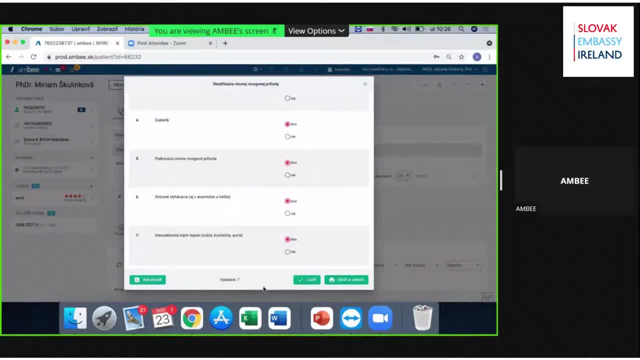 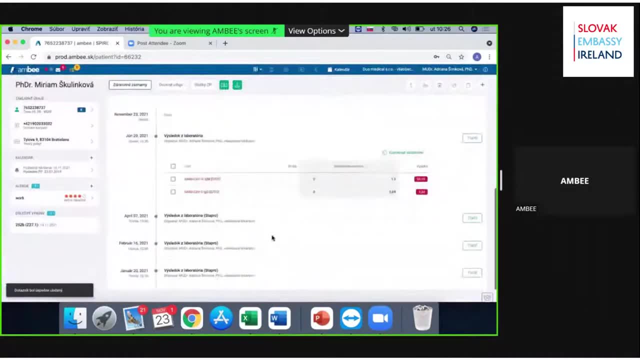 Look, I'll just show you very quickly: Done and safe. So the moment we have that, we can actually move to the next step, saying, okay, this patient needs another further checkup. We need to because of the stratification. we need to contact further specialists. 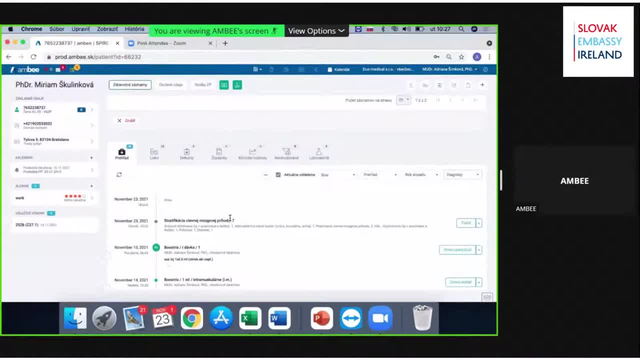 We have the same opportunity, not only for stratification of risk of strokes, but also, as I said, colon cancer, diabetes mellitus and other health issues. We have started to teach our doctors to do the repetitive prescriptions, so we can save. 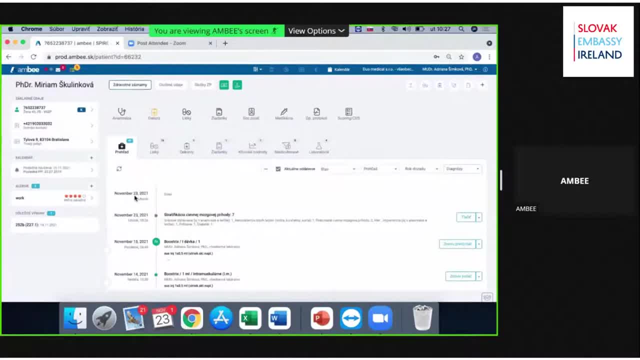 some money in terms of time and money in terms of writing prescriptions to patients. So our nurses don't have to rewrite prescriptions every month. They do it once and then they keep it like repetitive for nine months. So we save also daytime. So we have a lot of time and energy to heal people rather than do loads of paperwork. 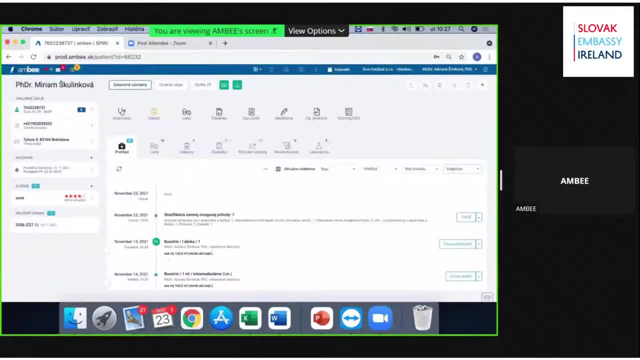 I'm not sure if I've done my three minutes. I just don't want to. I don't want to be longer than necessary. Are we okay, Or shall I finish, Or am I used? Have I used my time? Sorry, I just don't really know if I have used all my time. 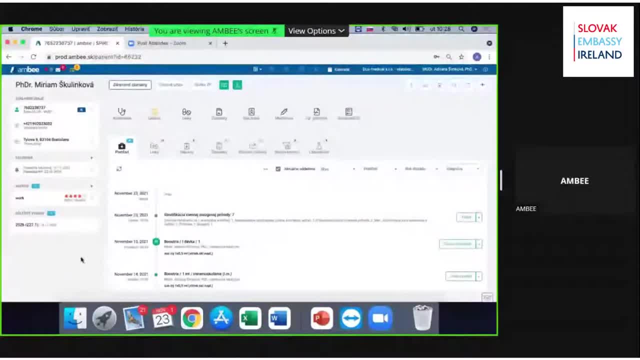 I'm we're good, We're good, Great, We're good. Thank you for doing all of these workups And you can get up to leave it up to me. We'll have a lot ofier work up to we have on next two weeks. 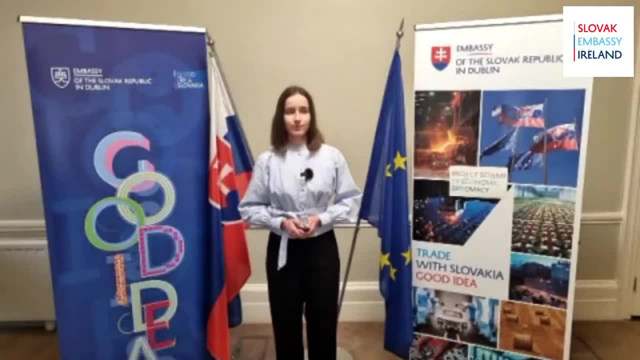 But anyway, thank you so much for sitting with us today. I think it's great being able to join the прич count. Good night, Have a good night. The next presenter is Mrs Nataliya Kr celery darkness. she's from Slovak company Medlerix. Medrax group laboratories examines 1000s of blood examples daily. 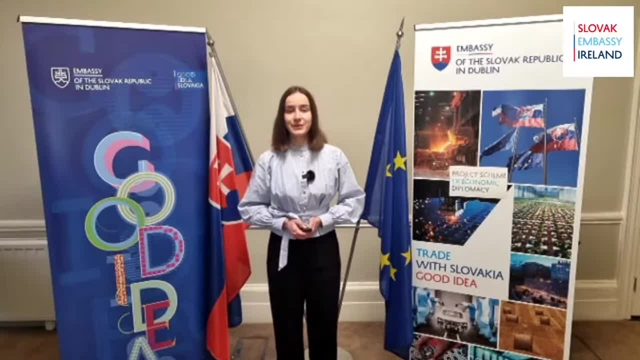 Another matter- for it's an example- Interesting treatments. This learning about diabetes has searched thousands of clinical blood samples. That's all very superficial, so that the staff can devote as much time as possible to more demanding professional activity. The company uses state-of-the-art diagnostic technology. 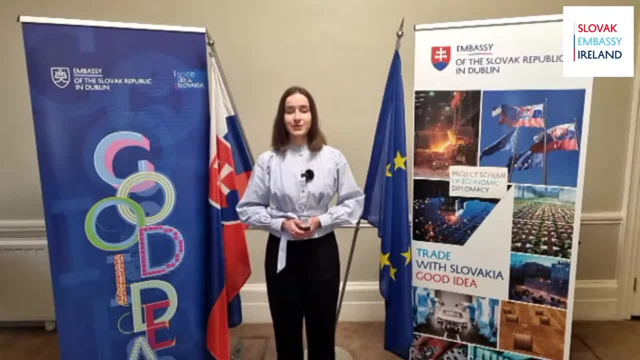 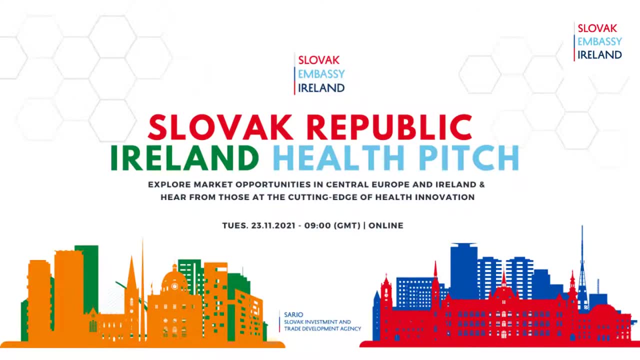 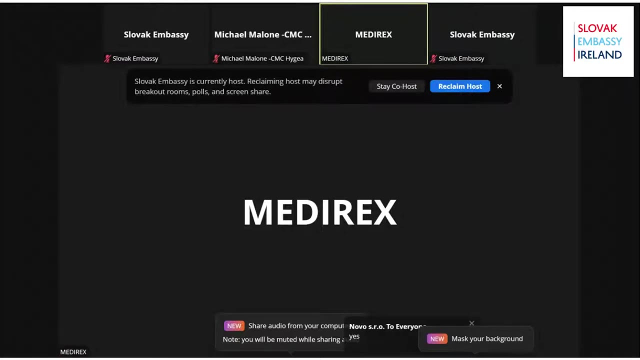 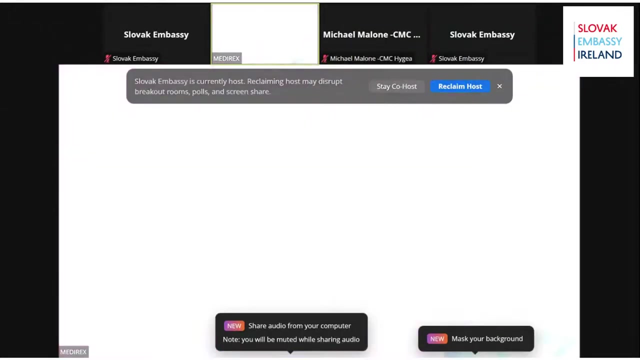 such as Maltito in microbiology to identify microorganisms. Hello, my name is Natalia Černíková. Okay, perfect, If you can just hear me, that's perfect, My name is Natalia Černíková. 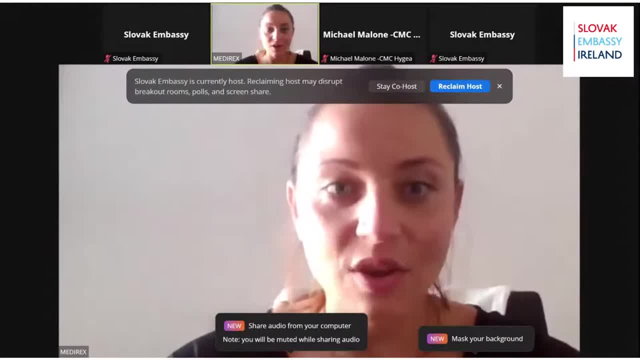 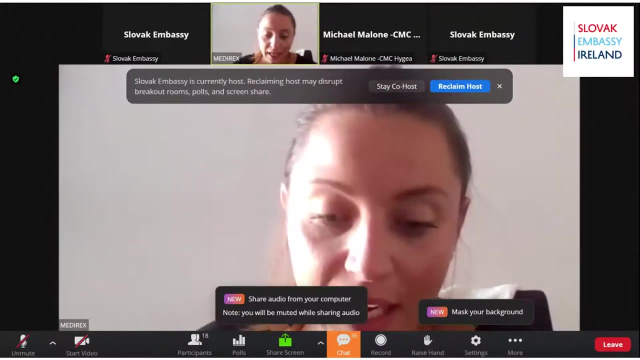 I'm representing the company from Slovakia. The company is called Medirex. Medirex is the leader in laboratory diagnostics with almost 40% of market share, which is the largest market share here across Slovakia. We are providing comprehensive laboratory diagnostics. 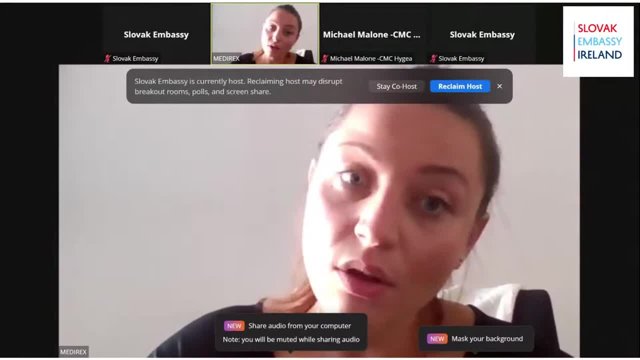 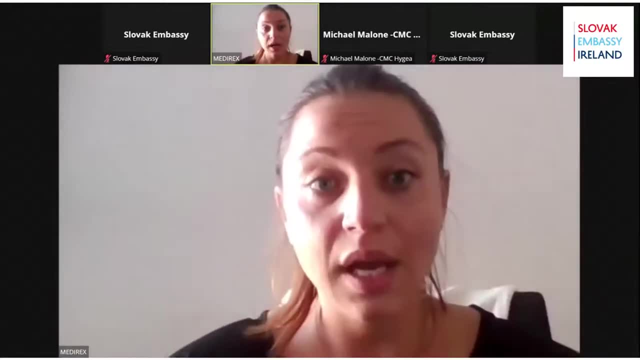 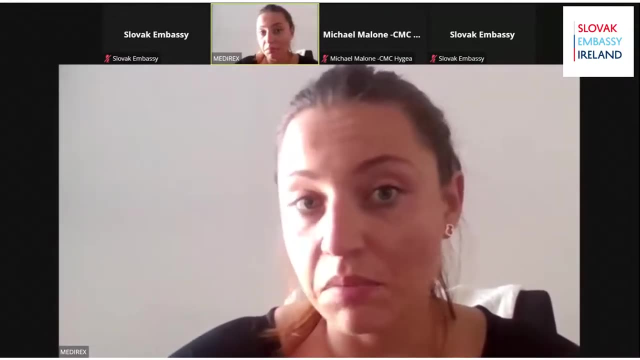 meaning all the departments under one roof, like pathology, like toxicology, biochemistry, genetics- and all these departments under one roof. We have three central laboratories in Bratislava, Nitra, Košice and also around 30 more like polyclinical laboratories. 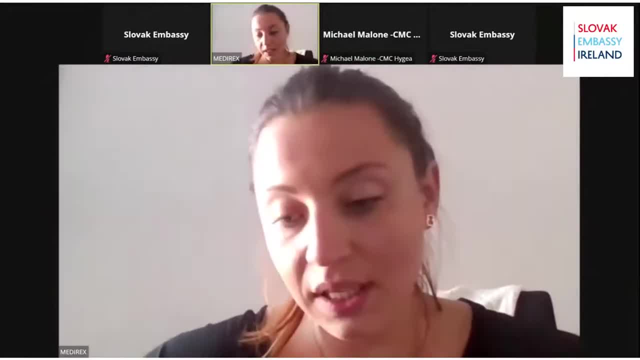 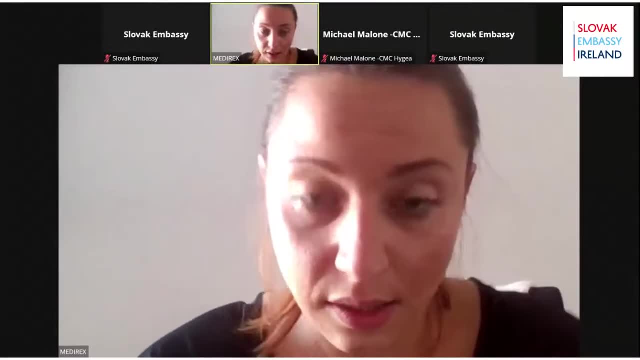 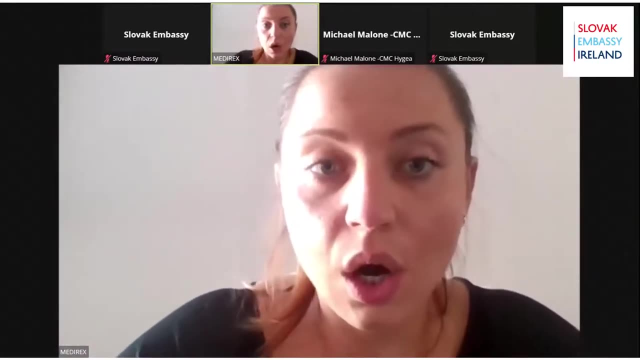 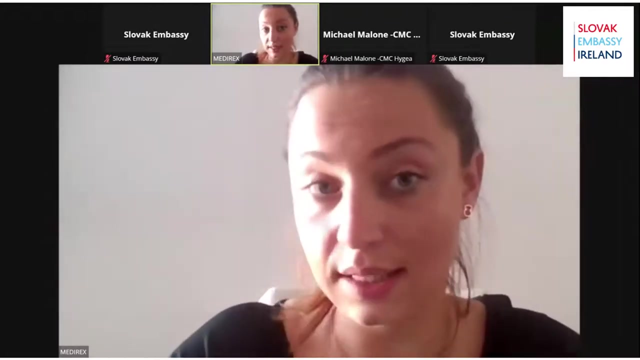 small ones. We have been active, let's say, for 20 years in this field And we are also active in R&D department, research and development. We are implementing our NIPT testing, called Trisomy test, which is the unique test, also here in Slovakia. 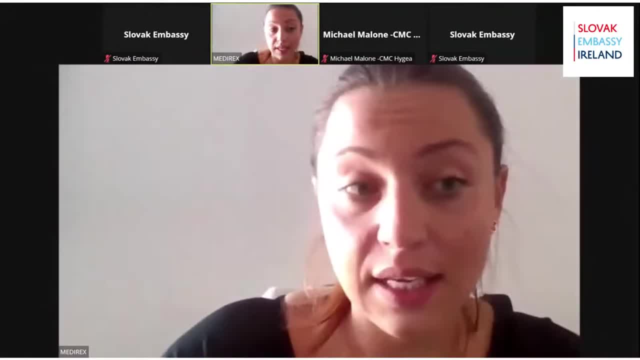 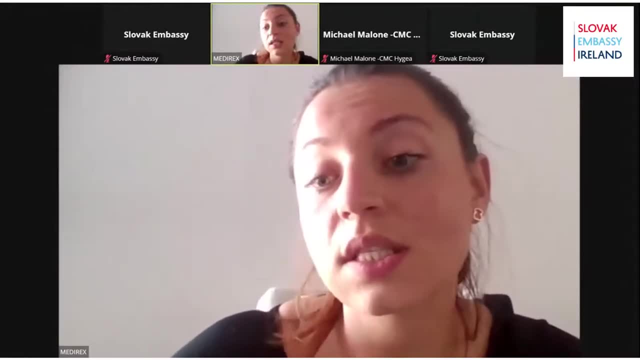 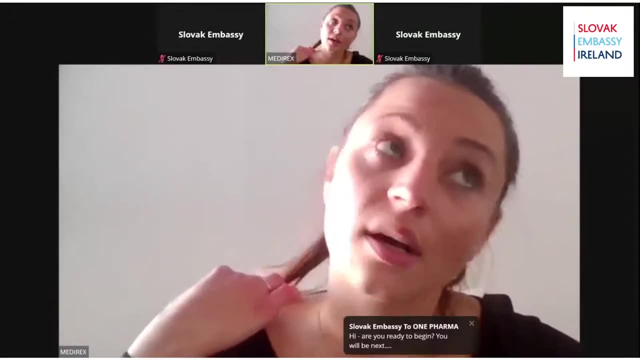 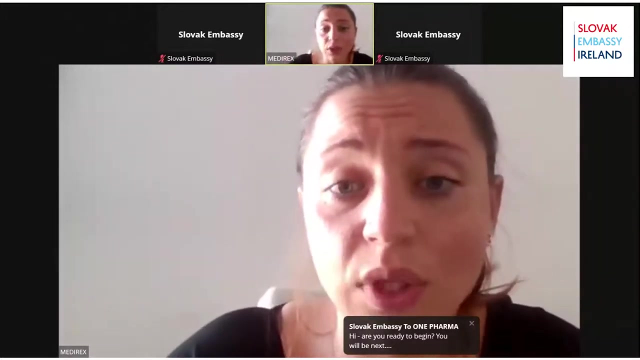 but also across the world. It's a non-invasive prenatal screening test which we can determine the sex of fetus, then Down syndrome, Pazos syndrome and also Edward syndrome and the other syndromes, like by whole genome sequencing. This unique test is called a Trisomy test and is very unique. 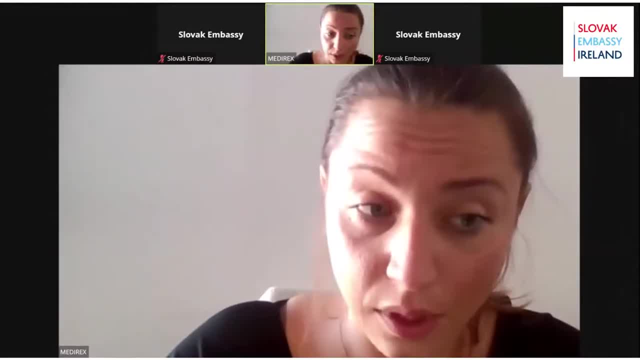 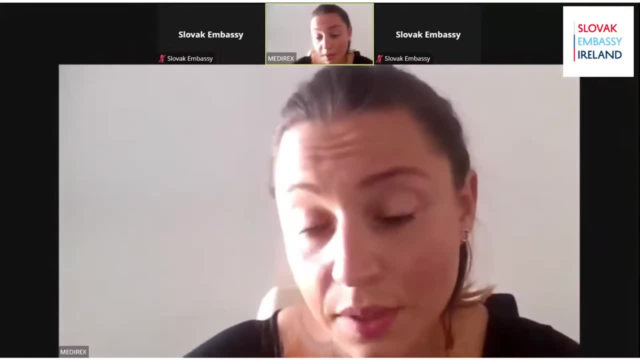 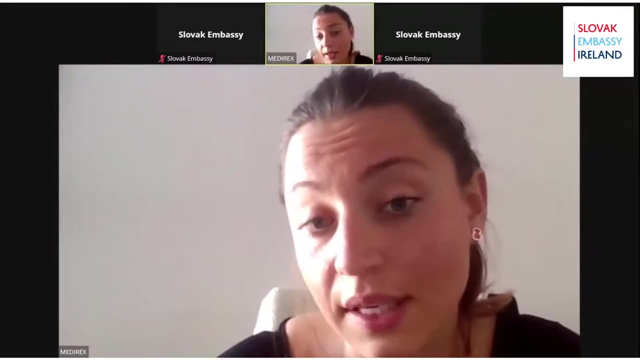 also here and also across the world. We are looking forward to it. Thank you very much, And we hope for a new partners and partnerships also abroad, who can just be our partners, let's say, depending in this kind of field or like meaning R&D in this Trisomy test. 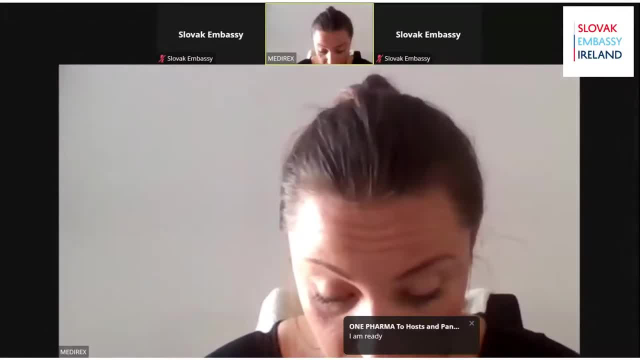 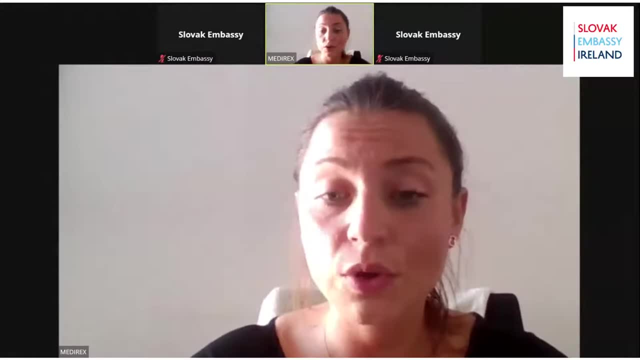 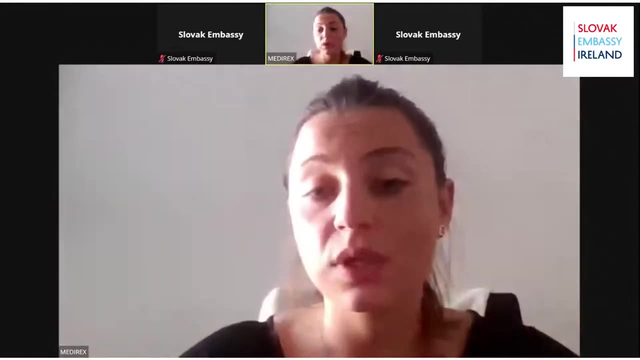 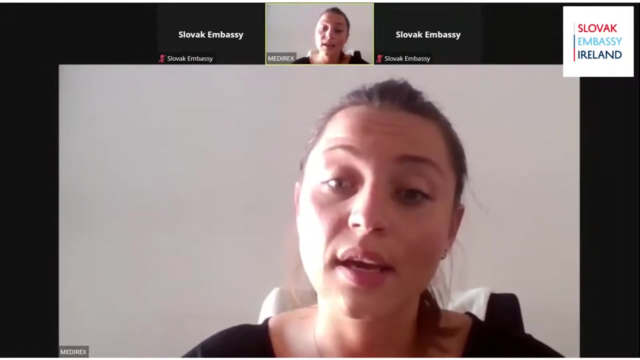 or the other laboratory diagnostics field. In these very crucial days and also in this crisis situation, we are implementing also PCR testing across Slovakia, let's say, building a hub by doing this PCR testing, where our daily limit is around 8,000 PCR samples. 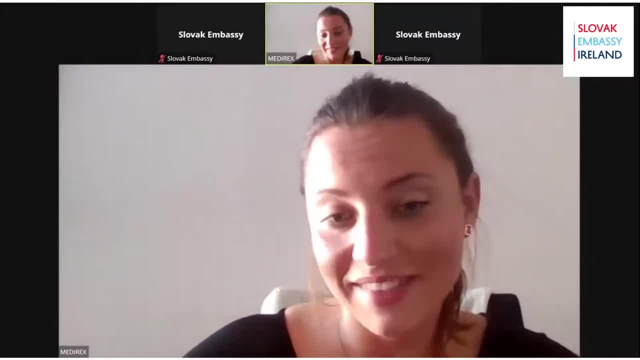 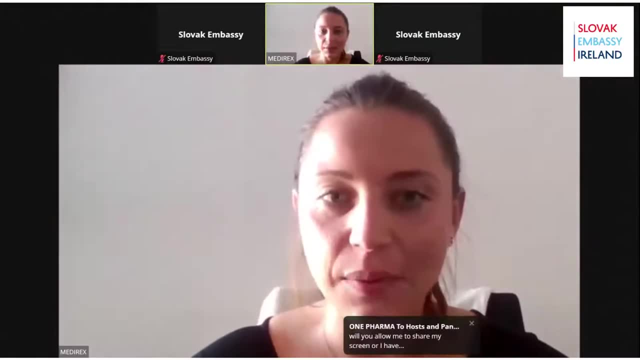 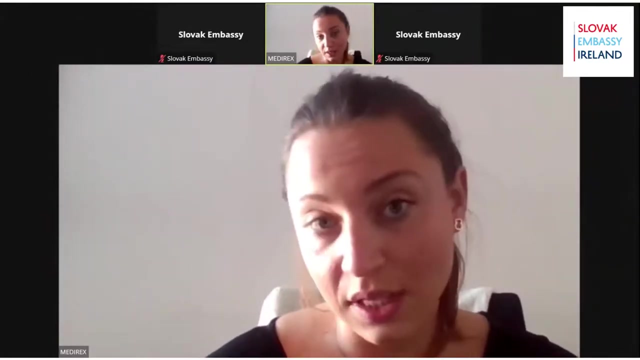 So I think that's enough for us to represent and enough for our timing- three minutes. We are looking forward to hearing from you or to sharing with you all the information about our laboratory system, our laboratory diagnostics. So we are here to discuss further cooperation. 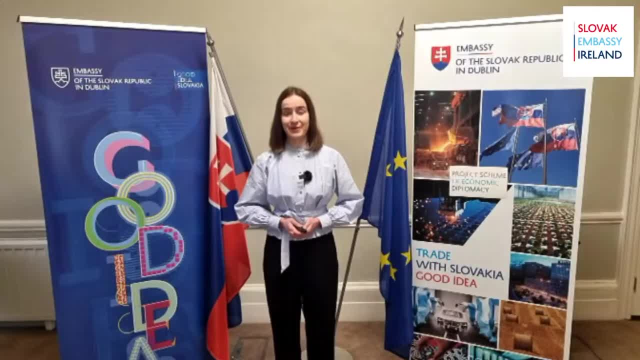 Mr Michal. Mr Michal, I am from Slovak company One Pharma. One Pharma was founded in order to provide the products of highest quality. The focus of production is oriented primarily on products that are of natural origin. The main goal is to take care of your health. 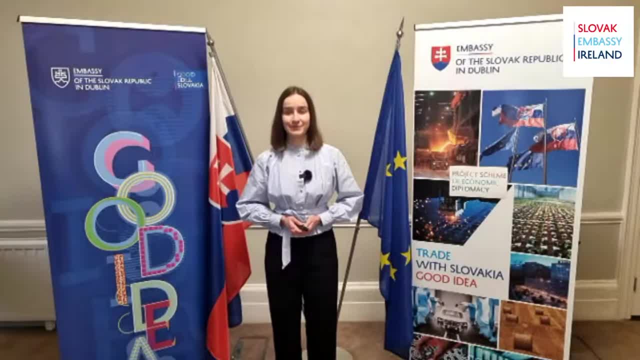 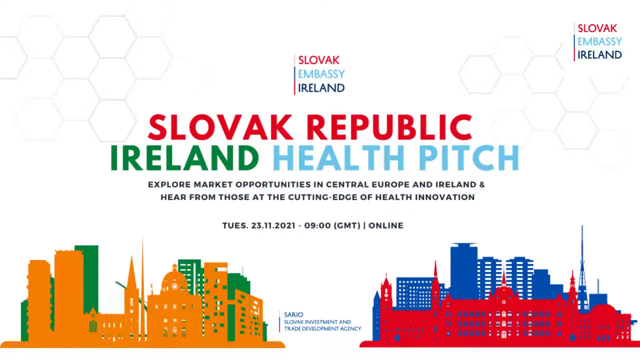 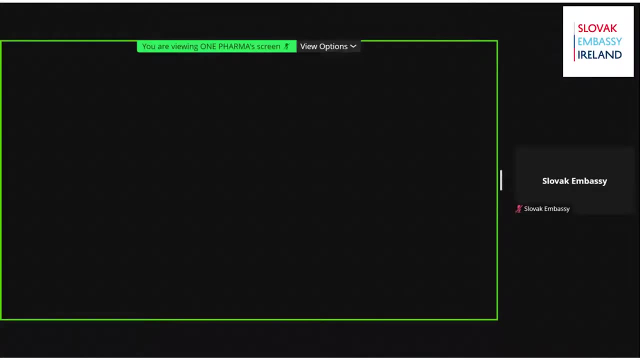 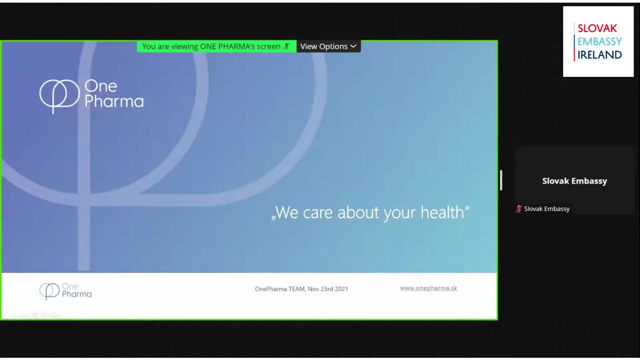 support it for all ages, from the youngest to the elderly, And the goal of this nous is to make sure that we offer the best quality and quality human health services and to make sure that you are doing well in your lives. So, without further ado, let's get started. 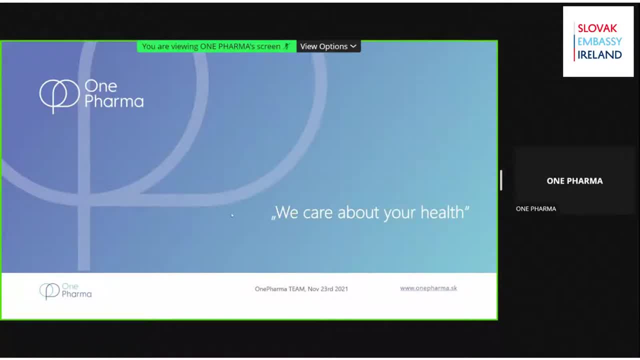 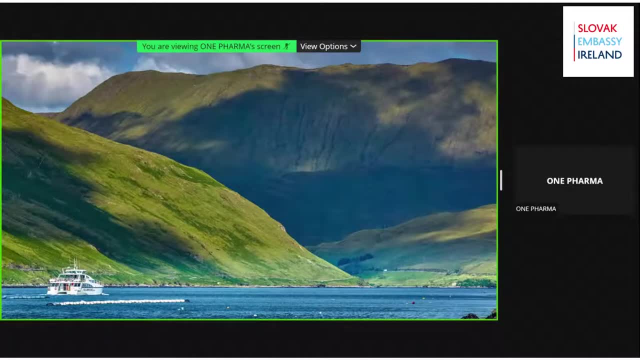 Good morning everybody. Thanks for the words, So let me I'm starting with a beautiful image of Killar, tranquil Ireland. fjord is the result of repetition, repetitive mixing of sea and fresh water moving in and out until it carves the hole through the rock. and this is happening day by day, year by year, millennia by. 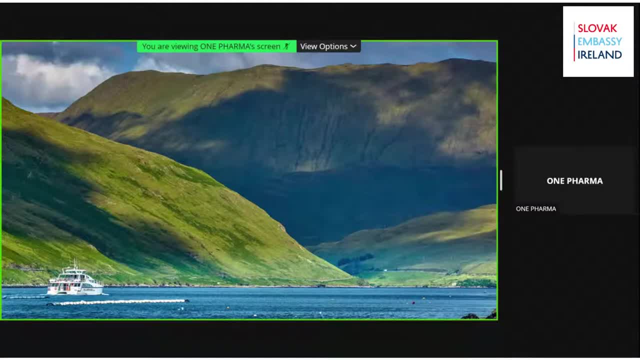 millennia until it carves this hole through the rock. and this is how we are thought to run the business. do the processes, do it again and again, and again, and the hard work consistently repeated over the time can build you a big, big fjord. but today i came to talk about the bike race in italy. 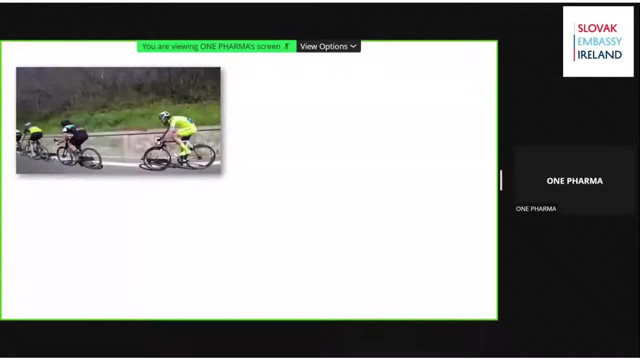 now. this is the snapshot from the very famous video, and you can see the actual footage of a guy losing his bike race. he knows that repeating the thing over and over the time is the isn't the best thing to do, and it's not the best thing to do and it's not the best thing to do and it's not the. 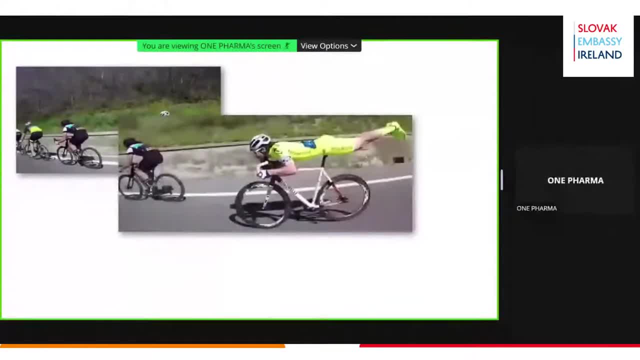 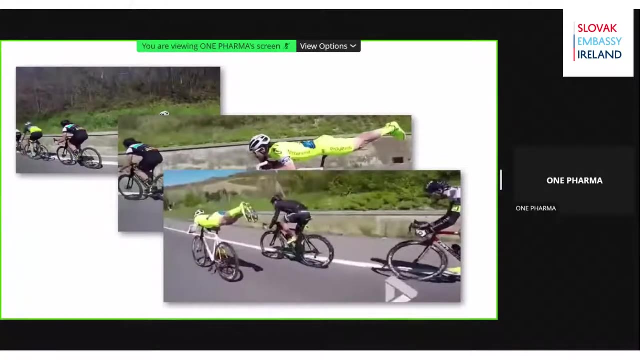 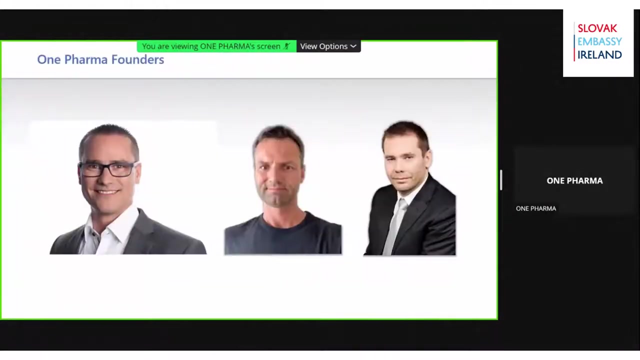 method. so if he tries to use aerodynamics a little bit differently, he can figure out how to get ahead of all other bike racers. and this is it, and this idea that innovation, creativity and focusing on efficiency may pay off, let me and my partners to start our business: one pharma, so we have a strong. 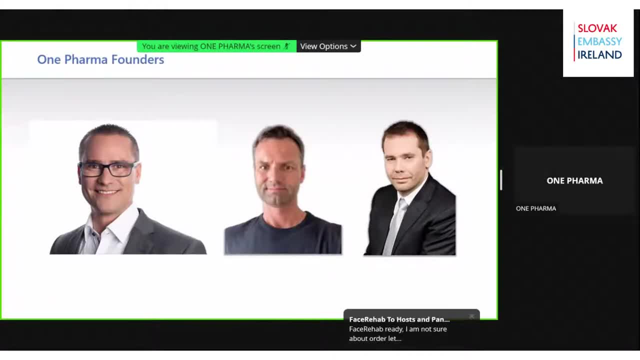 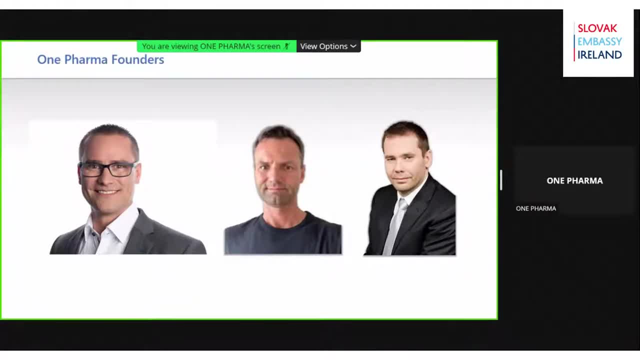 wanted to be absolutely different. we want to bring unique solutions to existing medical issues, rather than just a mix of ingredients or just another copy of existing products. so we build one pharma on the values, principles mostly efficiency, transparency with fair play and science-based approach and, of course, satisfied content, and we want to bring unique solutions to existing medical 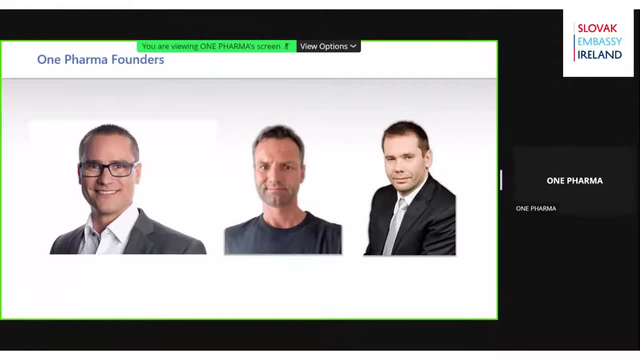 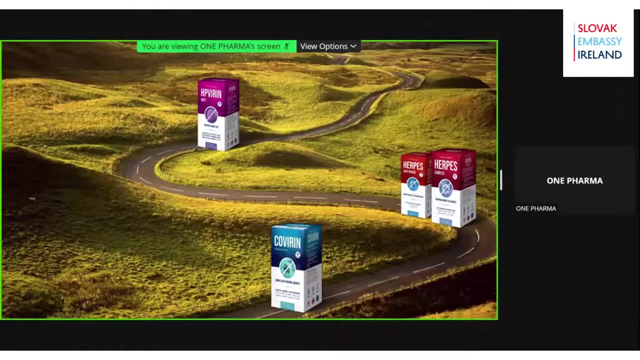 issues, rather than just a mix of ingredients or just another copy of existing products. so we build community цис topics around. We have been on the road for 18 months, so we are a fresh company, but we already hit three significant milestones and you see our production, our own products. because of time I will not go into the details of, but I would like to mention. 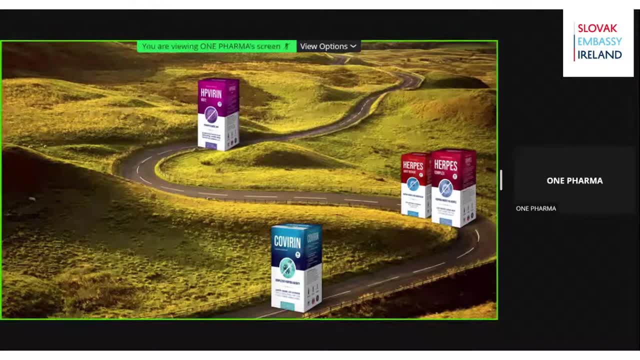 the first product, and most important, is COVID-19, because this is the respond to the current epidemiological situation worldwide. this is a huge εδώ. This is a premium, high-quality immune booster against SARS-CoV-2 and other viruses. consists of 15 active pharmaceutical ingredients. 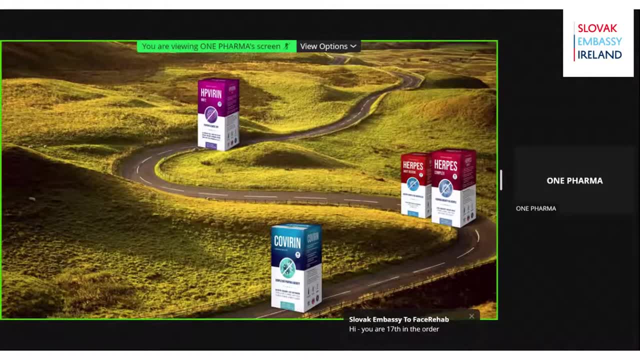 This is about the journey, not the direction, not the destination. but the direction for us is absolutely clear. So next year we are planning in our pipeline next six own products. There is one common thing behind all our products, and this is the memory of Eastern philosophy and Western science. 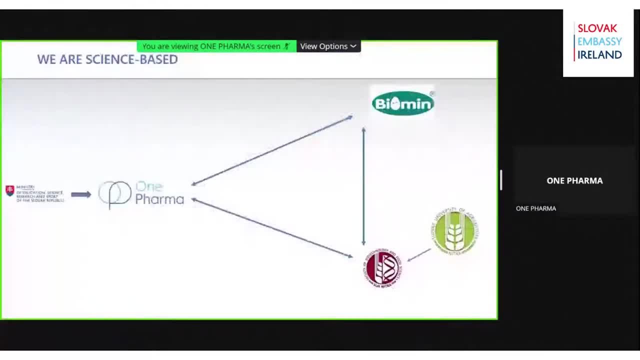 As I mentioned, that one of our values is science-based approach. this is a proof of concept, because One Pharma is a certified company for research and development by Ministry of Education. We are not working and operating alone. We are partnering with Biomin, which is a Slovak pharma company. 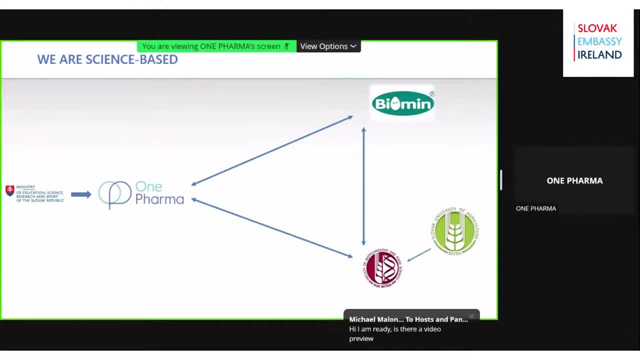 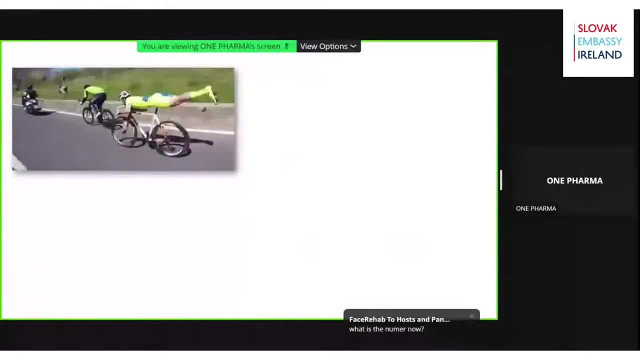 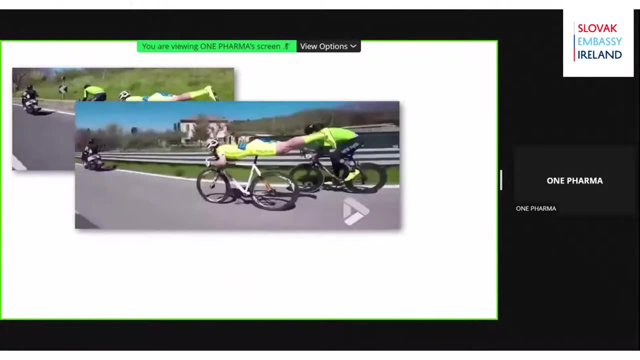 We are a producer and a faculty of biotechnology and food science, So I didn't show you the end of the race. So you saw the principle of the innovation, creativity. So this guy really got ahead of all racers. He is on the first place. 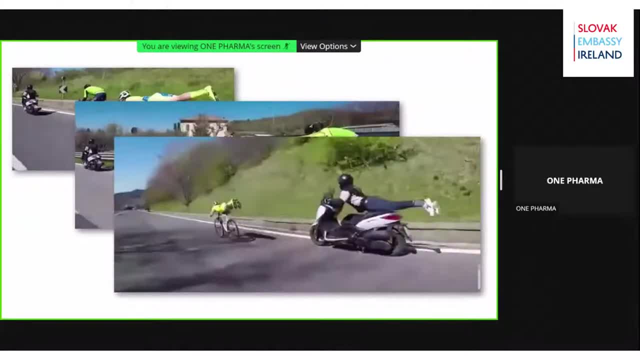 Everything is great until somebody is copying you And you know what you are going to do now. You have to start over again. So thank you for the listening And we know how partnership is important for us, And this is the reason that I hope you are the people with the same values and view on the business. 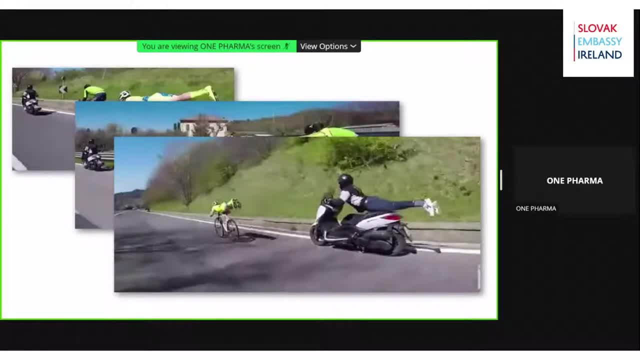 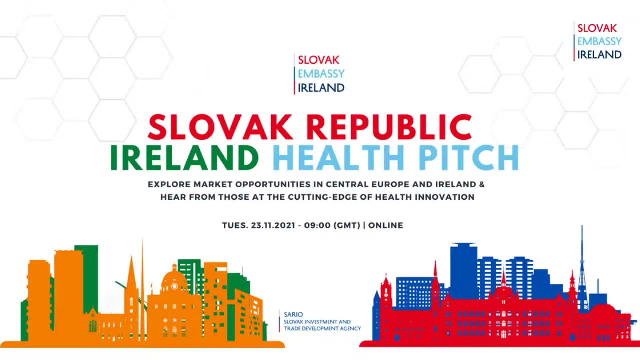 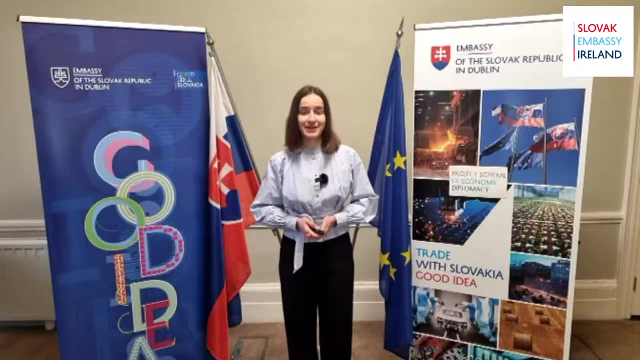 And we'll be glad if you will contact us and we can build our own success story in Ireland. Thank you very much. The fourth presenter is Mr Michael Malone from the Irish company CMC Hygieia. The main mission of company is to develop and deliver unique, hygienic and safe products which make a significant contribution to infection control and prevention throughout the global health care system. 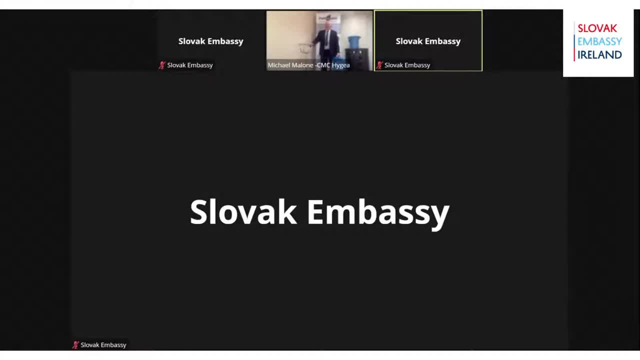 ==pruro plans whatever, and we might get more funding in the near future, which we are hoping to increase soon here. Mr Malone, please go ahead and ask the question. Man at your left hand. we're going to take questions, No focus. 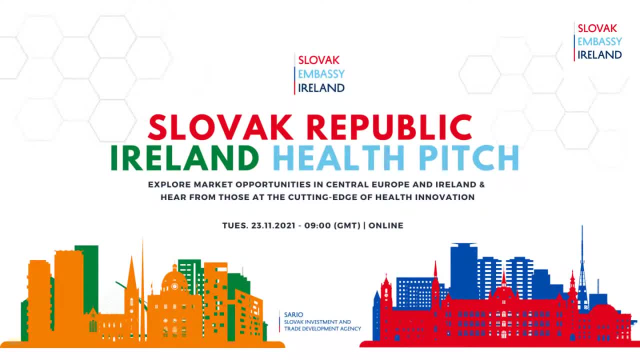 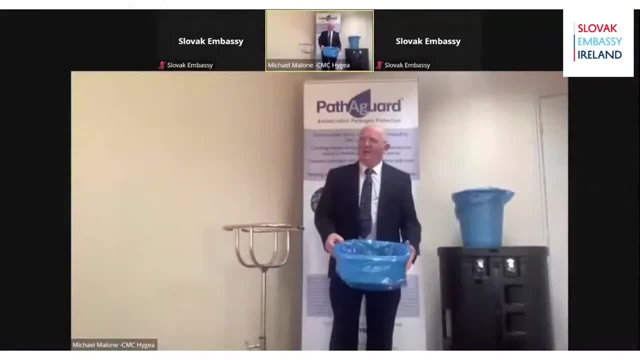 A lot of people asked me to talk and asked Points, to took questions- Main topic- and then you can show us for the next questions. Thank you very much. No, won't be able to confess or say anything. Thank you, mMay be, but Ng. 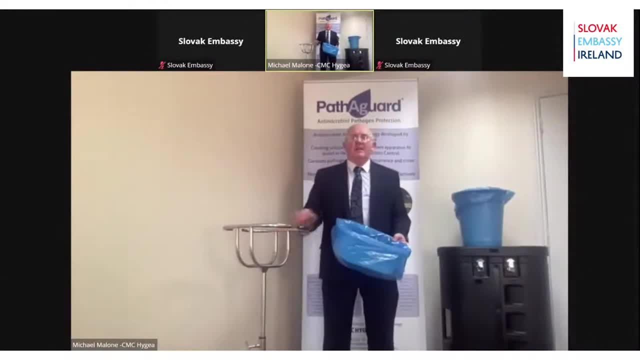 No, Your turned your back and back. Yes, You have a chance. My name is Michael Malone. I am CEO and founder of a company called CMC Hygiene Limited, based in Waterbridge City here in the south east of Ireland. Our aim here was to 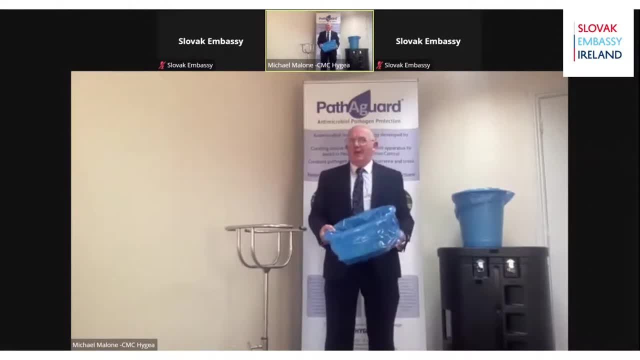 research, design and develop unique hygiene products and room management charts. So here's the first presentation is our Patagard Atlas. It's a bespoke silver iron impregnated basin to mitigate the risk of cross-contamination between patients and the products. It works in conjunction. 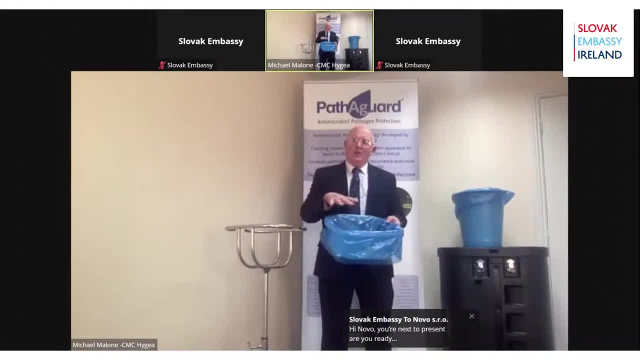 with a single-use disposable liner. When the patient is washed, you simply dispose of the liner, and the patient or the water never comes in contact with the patient. It is impregnated with silver iron technology to mitigate the risk of harmful microbes which could lead to HAI. 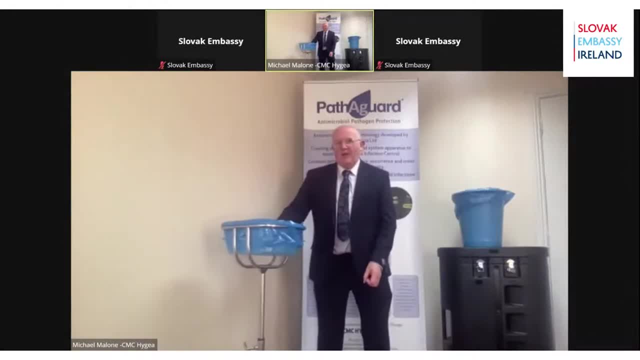 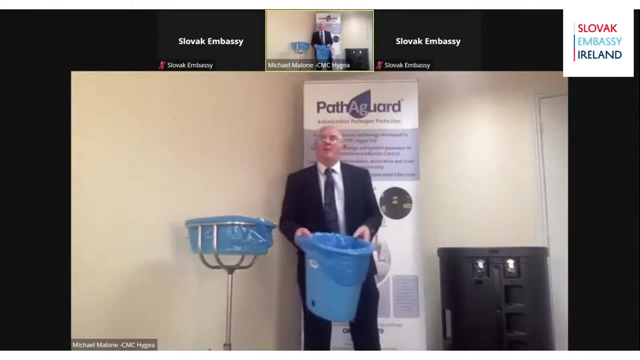 It comes in conjunction with also a wheel-based trolley to mitigate the risk of human factor engineering. Our second product was designed for cleaning and aiding leg ulcers. We call it Deluca leg ulcer cleaning aid. So to date there is no product on the market. 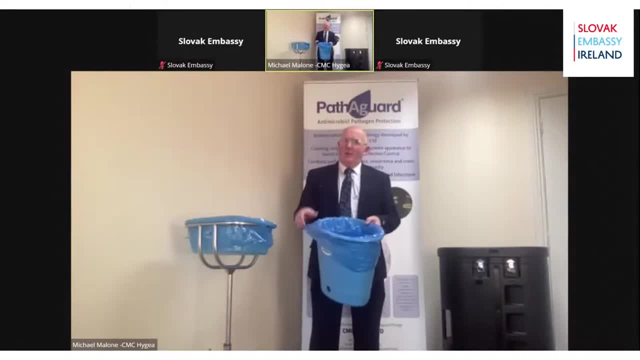 specifically designed to aid and treat leg ulcers, which is, as our populations are getting older, we need more and more care. So you simply pour the water into the vessel, into the liner inside the vessel, put the patient's leg, immerse the wound and this is going to enhance the value. 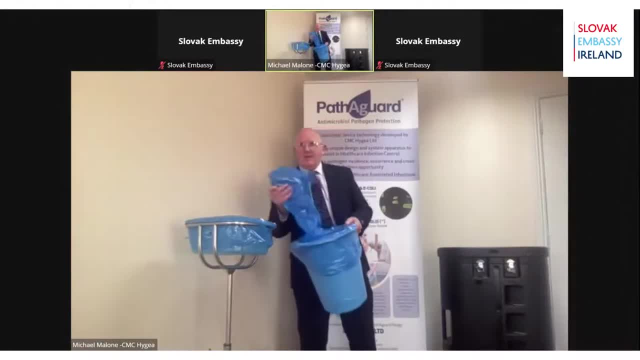 of cleaning and aiding the leg ulcer. There's a number of parts to the um. there's a Lucas sleeve. you probably see it on our website, the Lucas sleeve. You probably see it on our website, the Lucas sleeve. You probably see it on our website, the Lucas sleeve. 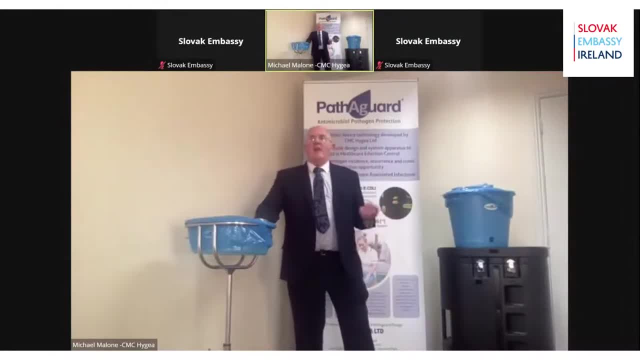 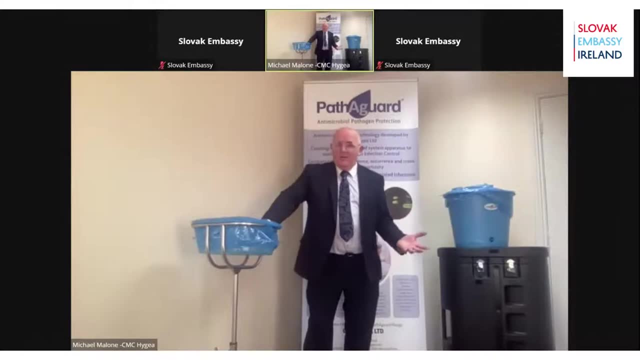 You simply pull the sleeve up on the patient's leg, You can create a clinical setting in any primary or person's home or house. This also is to mitigate the risk of cross-contamination from the products to the patient. Please look at our website on wwwcmcygeacom. 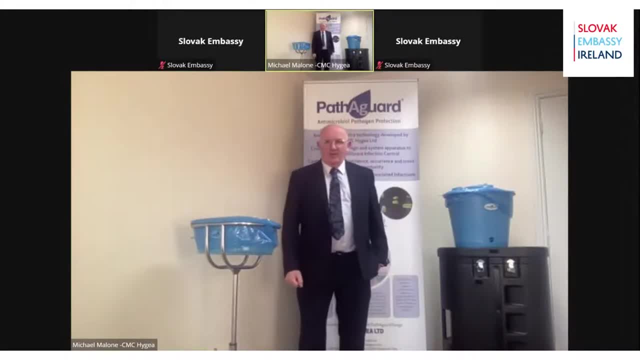 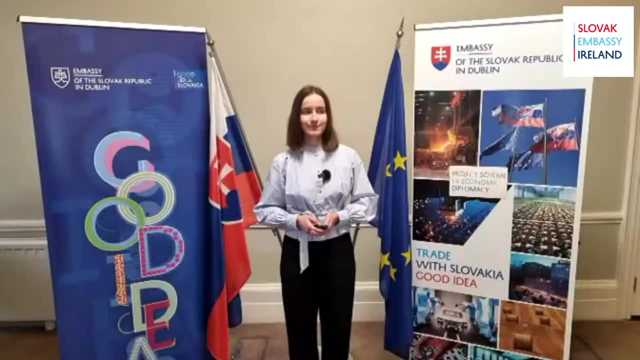 and we will send you any information you need. Thank you for your time this morning. The fifth presenter is Mr Petr Novák from the Slovak company Novo. The company Novo is focused on the development and constructions of technological innovations and devices that help in various spheres of society. It deals with progressive systems for 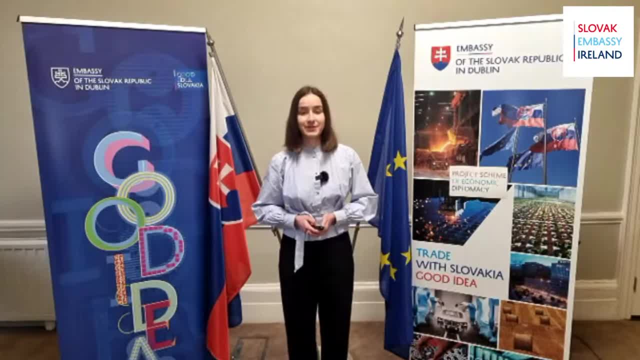 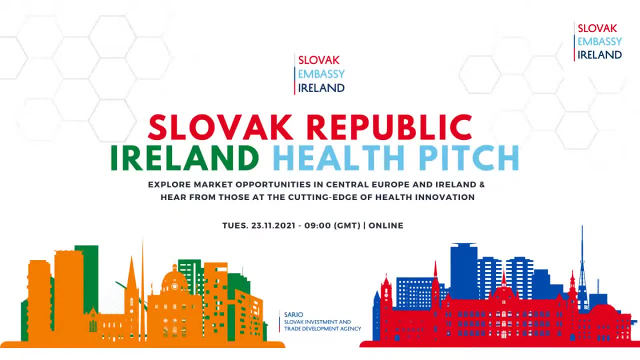 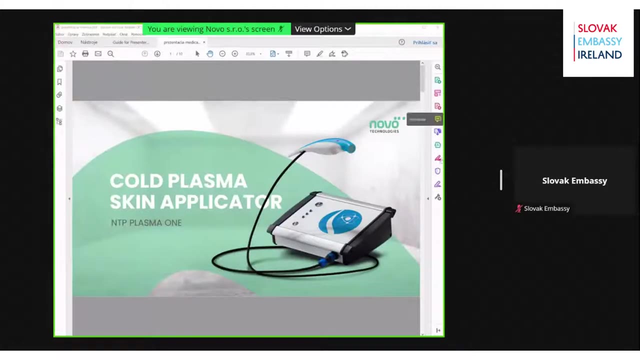 disinfection of skin, air rooms and materials, while the technologies meet the demanding requirements of the international standard. The first and most published covers this open source publication in late 2011,. being the capacity of the Slovenian The Clocare and Pula. 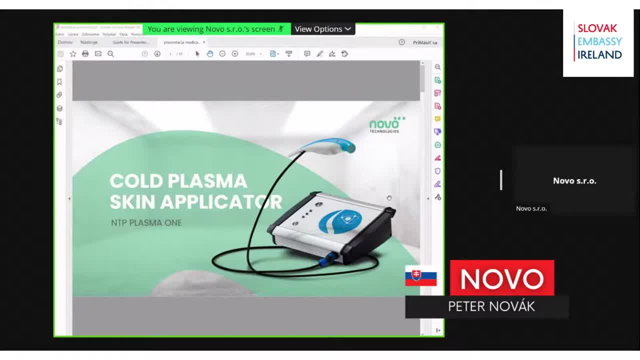 The Clocare and Pula are used as a source for developing medical and cosmetic appliances. They are again developed as a Coca-Cola and by Attila Jankova, a both estudio and research company. These devices are meant for both withcional and post-economic drift. well, what you cars as we do. have a UHM. worst language about these facilities, really, and these products are because we promise to an advantage as you two discover them. Okay, one second. This is Witan, speaking for the technology company, and we are a Slovak technology company in charge of building new medical and cosmetic devices. 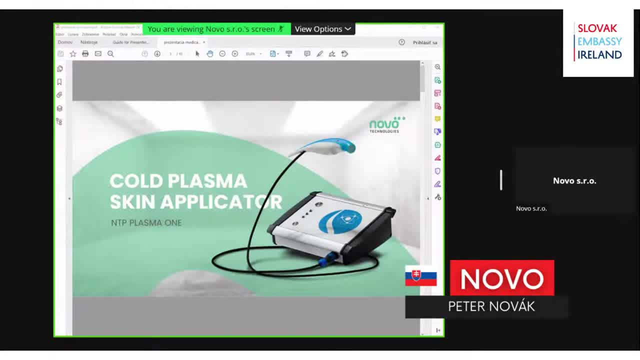 Once again, this is for the technology company, and we are a Slovak technology company in charge of building new medical and cosmetic devices. This device is, uh is at. it is freshly developed and it's patented technology, so we were presenting it last week- medica in this adult- and we find out that actually it's still the first of this type. 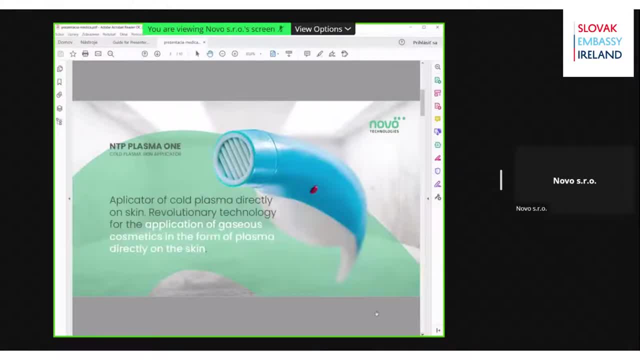 in medical and beauty industry. uh, what is it? uh, we, as, finally, you are using this applicator called plasma directly, uh, to the skin, and it applicates the gaseous cosmetic to the to the skin. so, generally, we have a new type of cosmetic based on the k, on the gas. 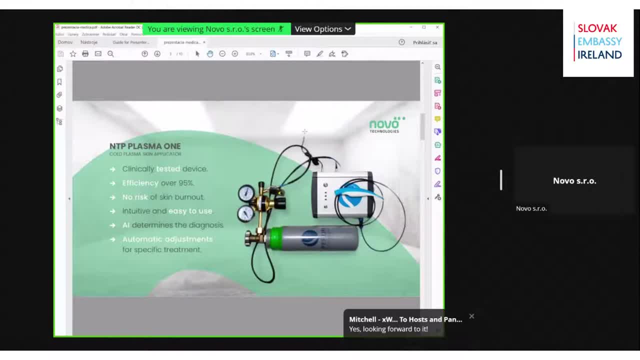 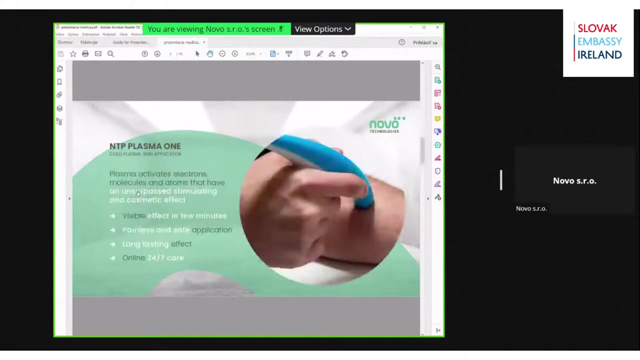 uh, what's the advantage of this device or using the gas in cosmetic industry is that, uh, it has very, uh, very high efficiency and it's very good. it has very good penetration rate and and it acts very rapidly in comparison to the present state technologies. uh, here's, uh, the effect of the plasma. you can see effect in a few minutes. it's very pain, it's very. 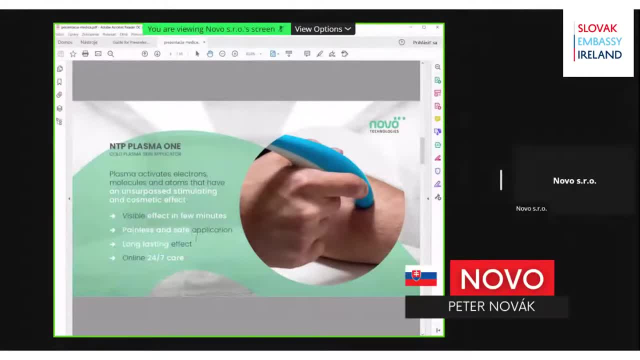 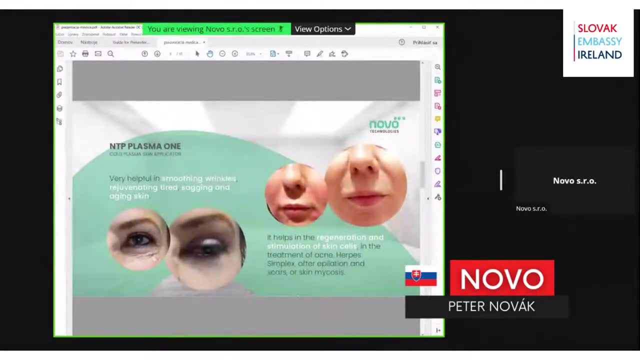 painless and it has a lasting effect. this is just a few examples of the studies we have already made. so this is uh we use it in in beauty industry. it's used for smoothing wrinkles and aging skin and other applications in beauty industry. it helps with the regeneration and 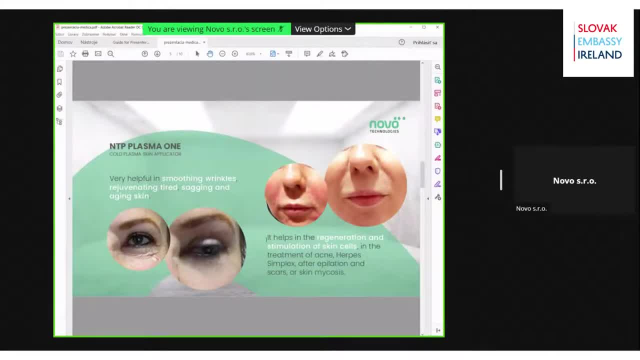 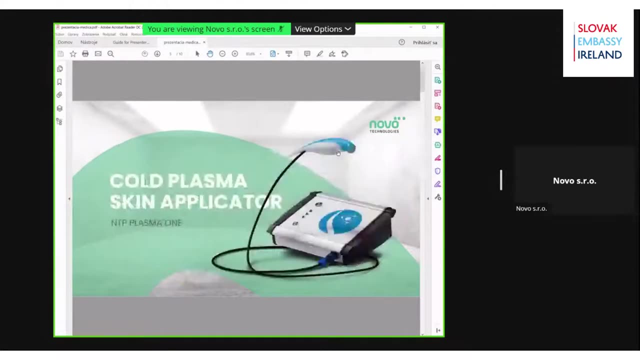 stimulating the skin's cells and those, of course as well, treatment, acne, hairpass, simplex and and so on. there are more application, okay, so this is about our patented technology. it's called plasma skin applicator, and we are now looking for distributors in whole europe. as i said, it's patent protected, so 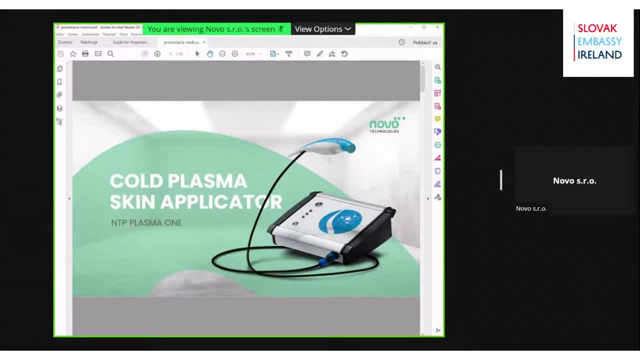 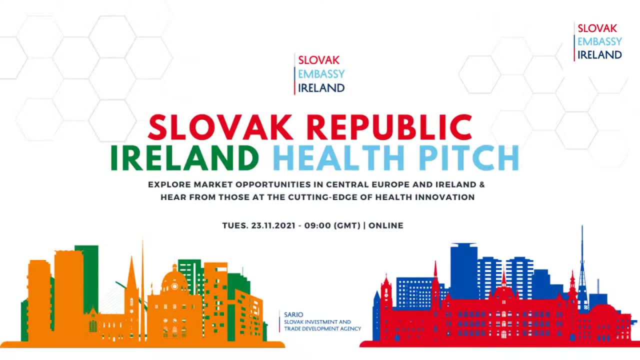 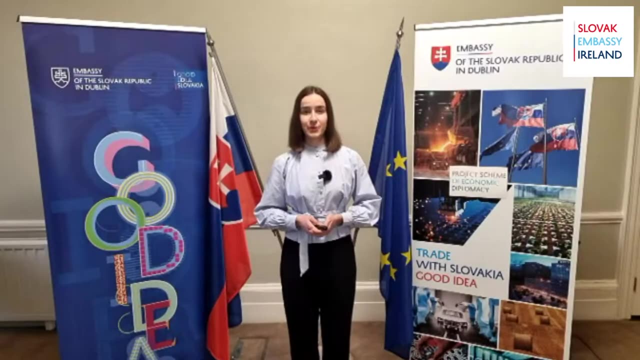 i will be happy to discuss if you have any questions afterwards. thanks, the sixth presenter is mr mitchell o'gorman, from irish company x wave. x wave technologies was founded in 2020 by a leading group of radiologists who wanted to create intelligent 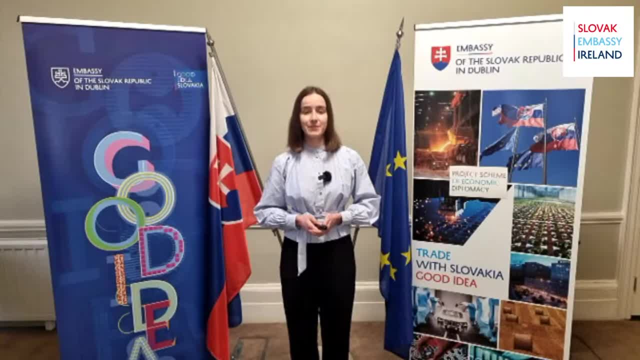 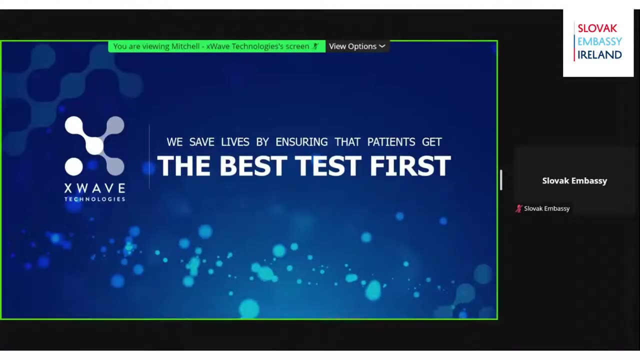 solutions for the problems they were facing. sync in their day-to-day work. X-Wave technologies use brilliant technology and data analytics to ensure that patients worldwide receive the best test first. Good morning everyone. My name is Mitchell O'Gorman and I am the CEO of X-Wave Technologies. 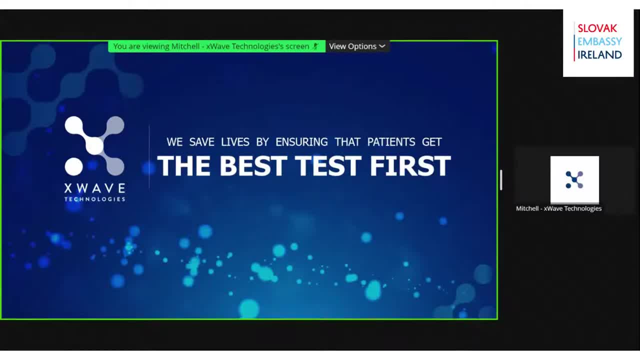 X-Wave Technologies is on a mission to save lives by ensuring that patients worldwide receive the best test first. X-Wave Technologies is on a mission to save lives by ensuring that patients get the best test first. Our leadership team is comprised of a mixture of commercial 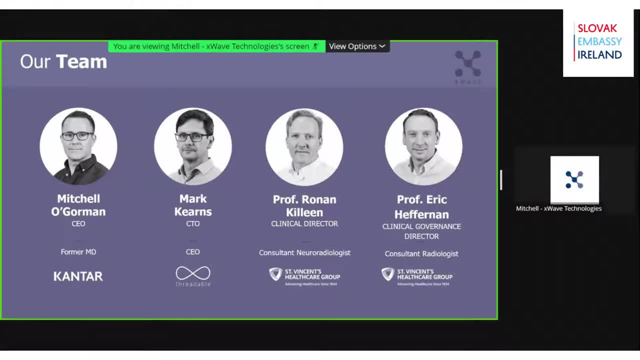 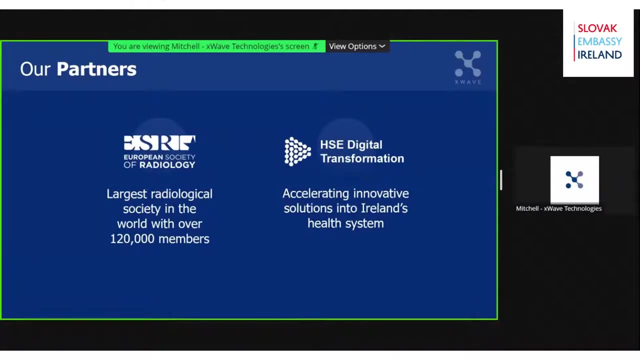 technical and medical expertise. Our Clinical Director and Clinical Governance Director, Professors Ronan Killeen and Professor Eric Heffernan, are two of Ireland's leading consultant radiologists. Two of our key partners include the world's largest radiological society, the European Society of Radiology. 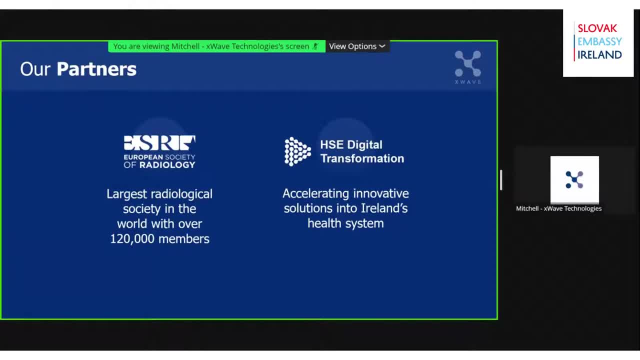 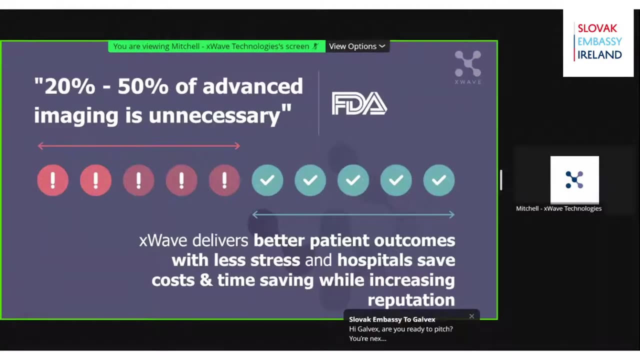 which has over 120,000 members, and the HSE Digital Transformation Team, which is accelerating the adoption of our smart radiology referral platform, X-Refer, across the Irish health system. The key problem that we are looking to solve is that up to 50% of advanced imaging is 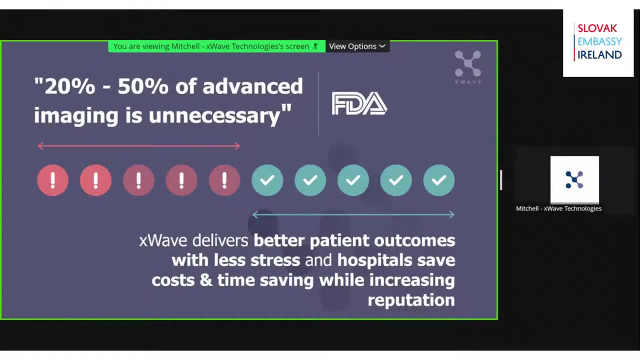 necessary for the patient. according to the Federal Drug Administration, This results in poor patient outcomes, misdiagnosis, delayed diagnosis, and costs health systems huge sums of money. In the US alone, it's estimated that between 7 to 12 billion US dollars. 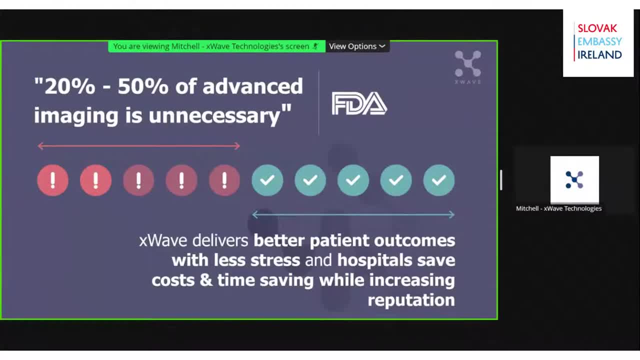 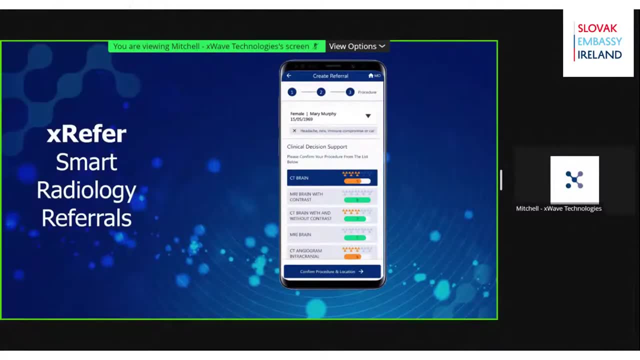 is spent every year on unnecessary imaging. Our solution is Europe's first smart radiology radiology referral platform, X-Refer. X-Refer uses market-leading data developed in partnership with the European Society of Radiology to give a referring clinician, whether they're a GP or a hospital-based doctor. 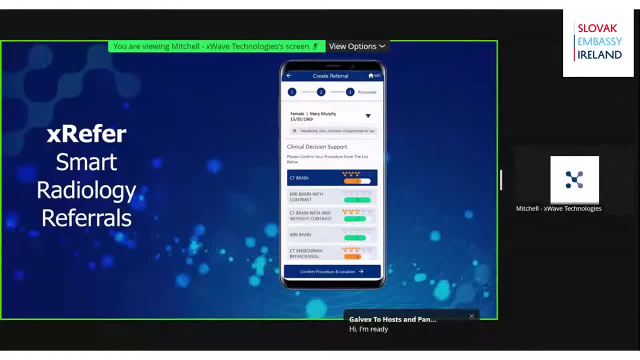 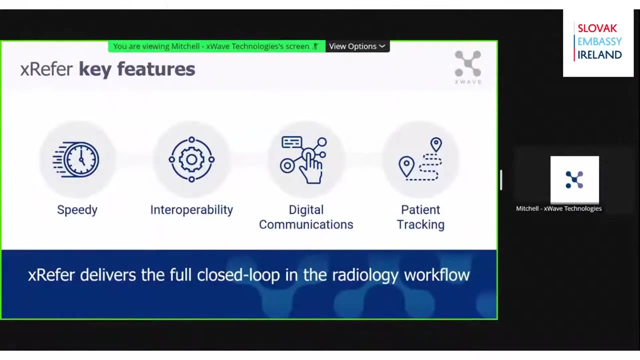 the best recommendation for the most appropriate radiology scan for their patient, based on that patient's age, the patient's gender and the patient's clinical indications. Some of the key features of X-Refer is that number one. it's fast. 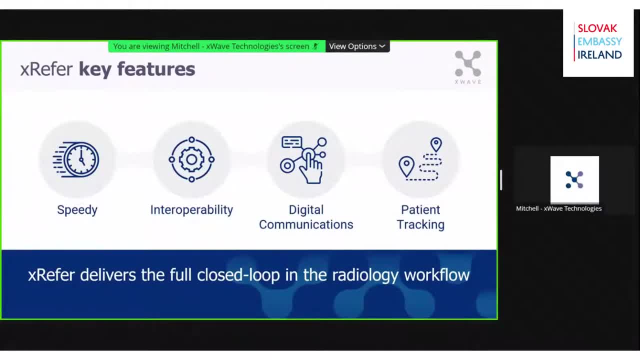 It's a cloud-based system. It's very fast to get set up and it's very fast to use, create and send a radiology referral. Furthermore, we have full interoperability with all systems, including the electronic patient record and wrist pack systems. 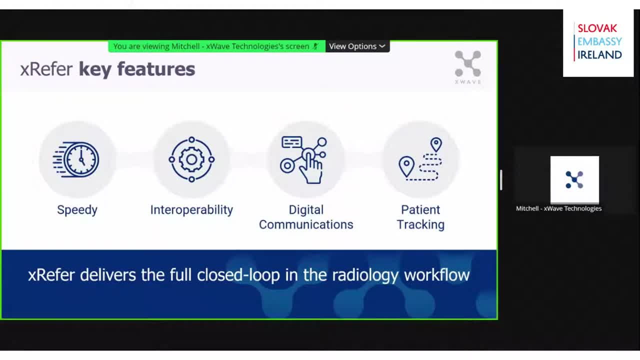 So we've developed a fire and a fire HL7 integration engine that seamlessly integrates. This then enables the referral to be sent digitally directly to the hospital, but it also allows the radiology team to have a digital chat directly with the referring team. 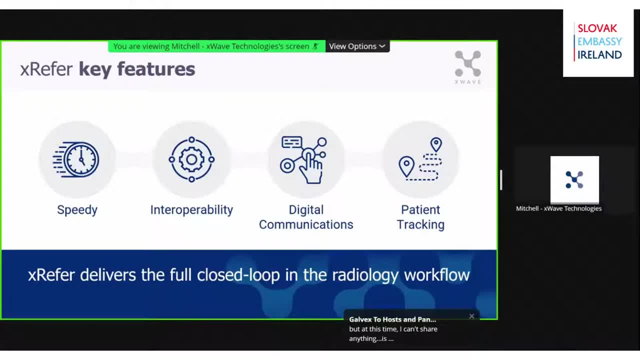 It also sends the radiology report and image back to the refer once the scan has been performed. Furthermore, we enable full patient tracking by the refer of their patient, so they know where their patient is at at every stage of their journey. 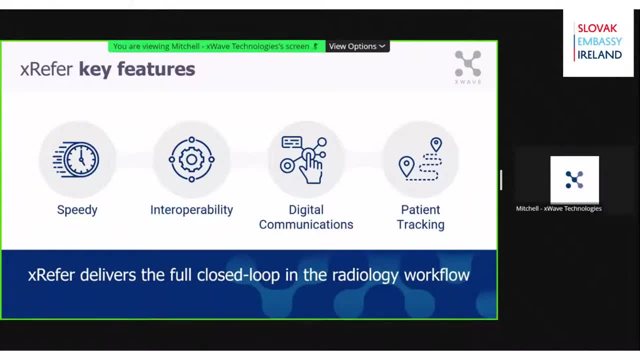 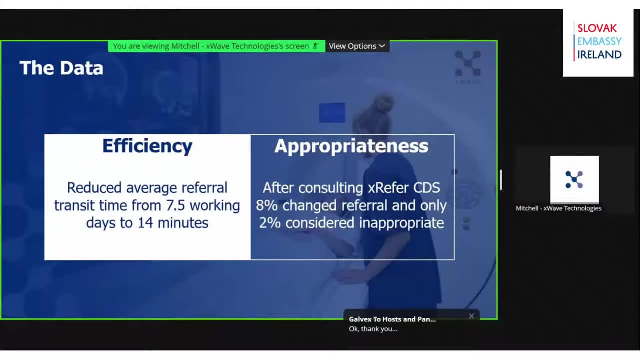 We deliver the full closed loop in the radiology workflow. Here's some case study data from three hospitals that we've connected in Ireland: a smaller specialist hospital linking into a large university hospital and to a private hospital. In terms of efficiency savings, we have reduced the average referral transit time. 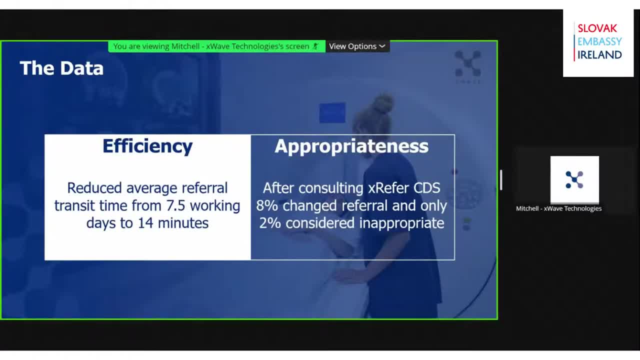 including radiology, from 7.5 working days to just 14 minutes, meaning that patients are getting scheduled for their scans a week in advance. In terms of appropriateness, after consulting the X-refer clinical decision support system, 8% of referrers change the referral, with only 2% of referrals then being considered inappropriate. 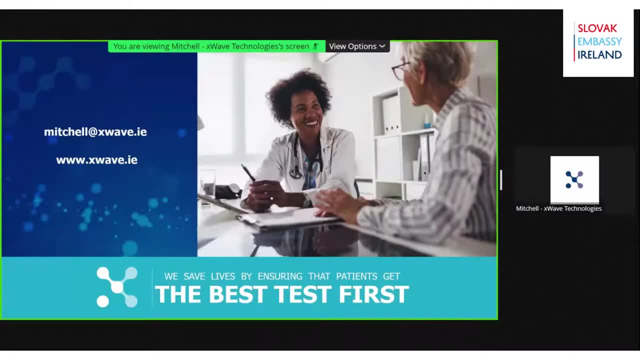 We're looking at a global market. Our ambitions are global. This is the reason this is a global problem. So we would love to chat to hospitals and health administrators in the Slovak Republic to ensure that we continue to save lives by ensuring that patients get the best test first. 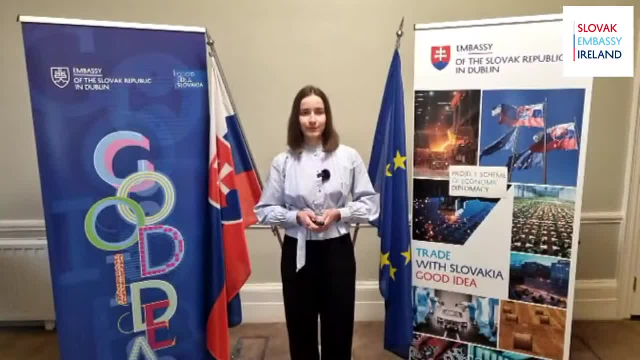 Thank you. The seventh presenter is Mrs Patriciak-Emes, from Slovak company Galvex. The company Galvex is focused on the technological equipment of renowned world manufacturers. Galvex has the authorization of the Ministry of Health of Slovak Republic for the production. 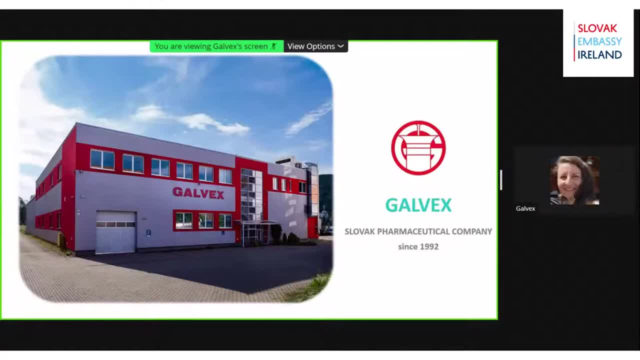 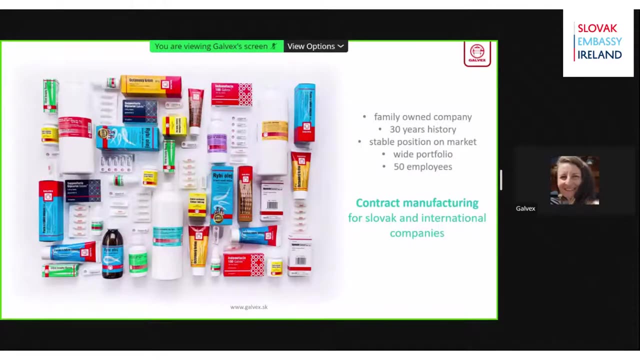 Hello, Can you hear me? Yes, My name is. My name is Patrícia. I'm representing the Slovak pharmaceutical company Galvex and I would like to briefly introduce you what we do and how we could potentially collaborate. The company Galvex is a family-owned company established in 1992, so at the beginning of the next year we will celebrate the 30th anniversary. 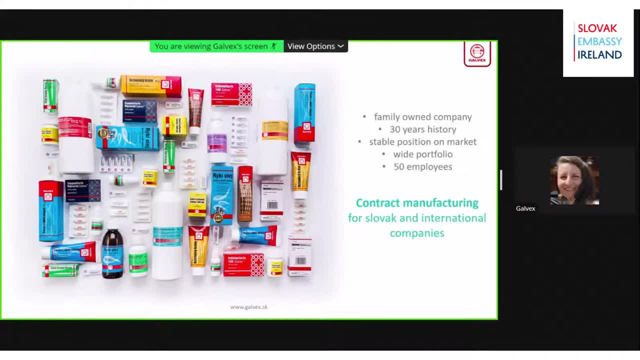 During our existence, Galvex has built the stable position on the Slovak market, but, what is also important to mention, we became the reliable contract manufacturing partner for many Slovaks, but also many international companies, And now I would like to show you what we offer as the contract manufacturing partner. 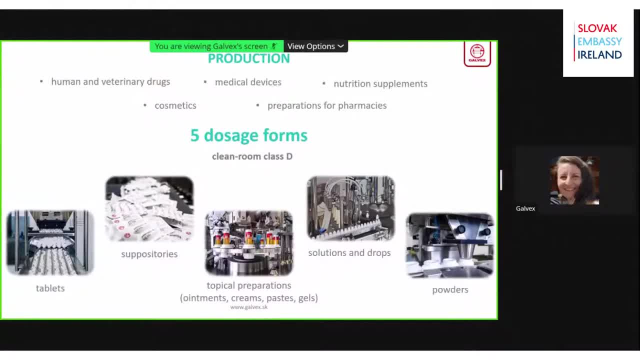 Although we are a small company with only 15 employees, we have a large number of employees. We are licensed to produce human and veterinary drugs, medical devices, nutritional supplements, cosmetics and preparations for further processing in pharmacies, And all these in five different dosage forms, like tablets, suppositories. topical preparations like ointments, creams, pastes, gels, solutions and drops. 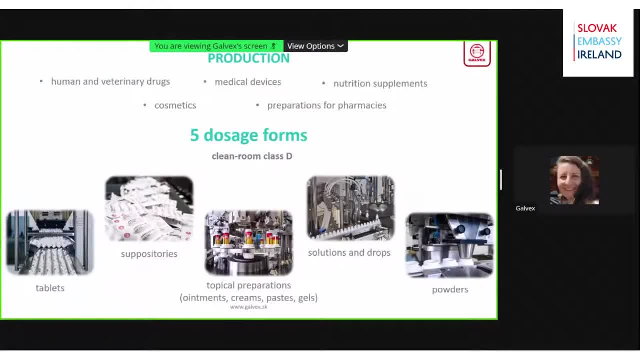 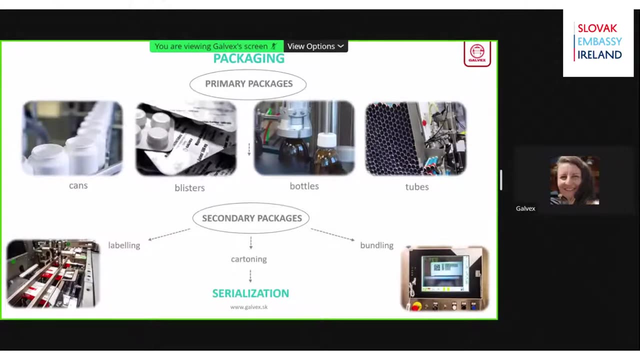 The whole production is realized in clean room capacity on the technological equipment of the well-known producers. The next step after the production is packaging into the primary packages like cans, blisters, bottles and tubes, and then into the secondary packages, And we can also do labeling, bundling or, for example, for prescription drugs, we are able to realize serialization according to recent requirements. 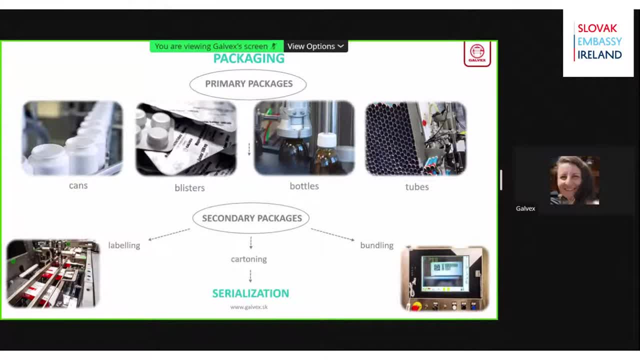 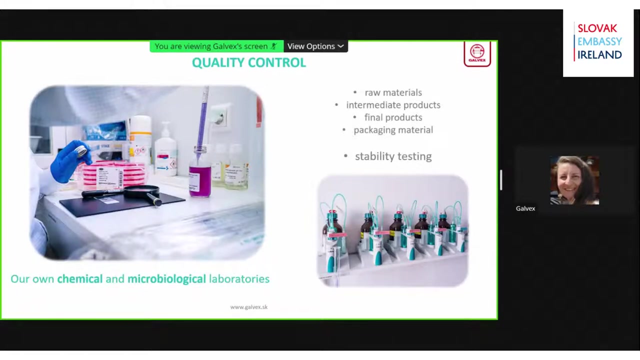 So we can prepare your product from the beginning until the end, from the raw material until the final packed product, Or you can bring your bulk product And we will pack it into the secondary packages, or we will process it according to your requirements. The quality control of raw materials, intermediate products or final products is realized also in our own well-equipped chemical and microbiological laboratories. 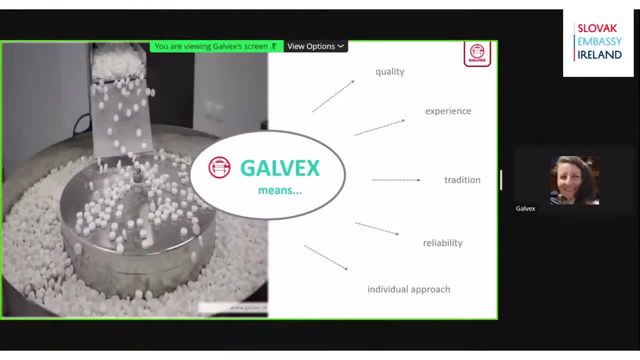 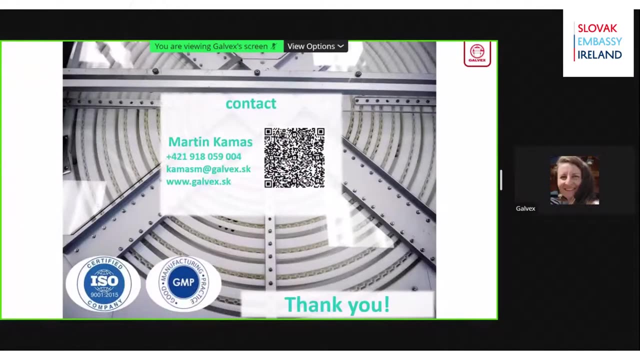 So what characterizes Galvex? Its quality, its experience also, tradition, reliability and, surely, individual approach. So do not hesitate to contact us, because every new partnership moves us forward, and that's our everyday motivation, Everyday motivation to improve ourselves, and that's our power. 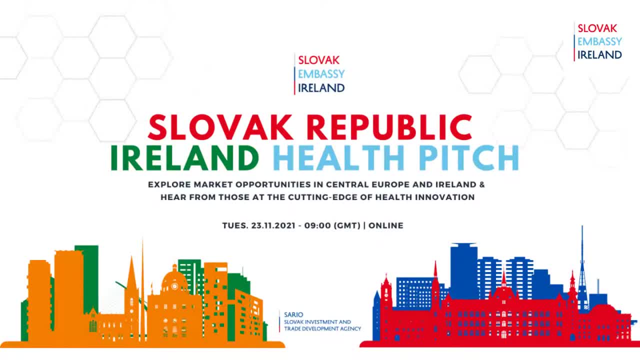 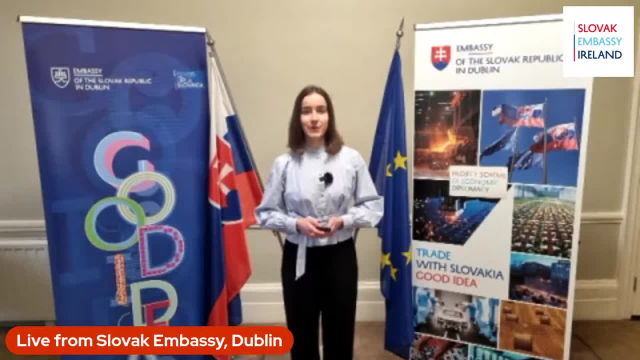 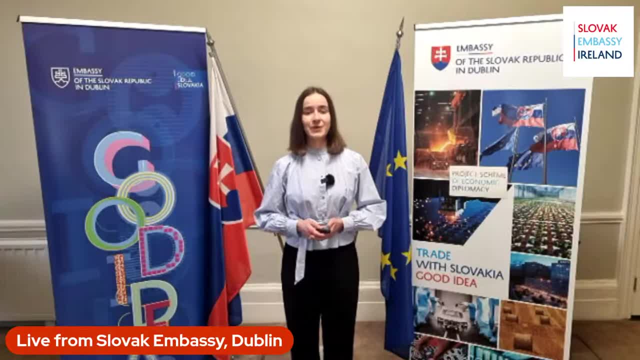 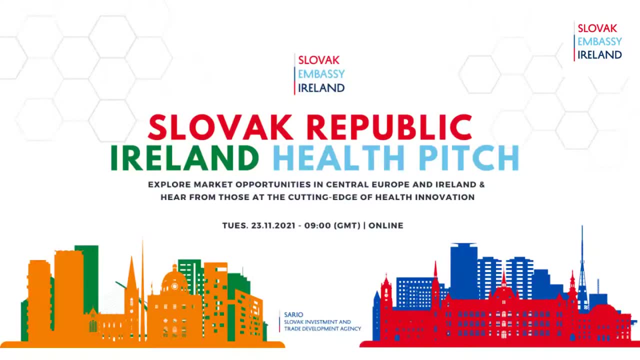 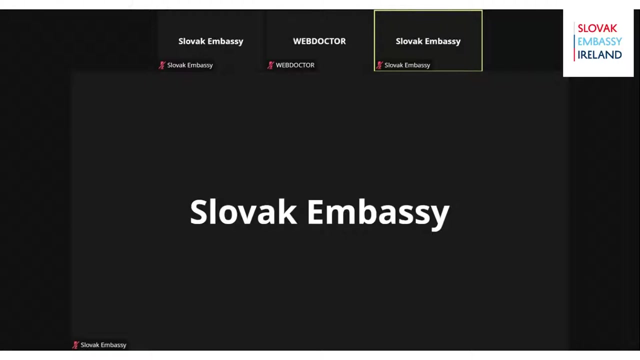 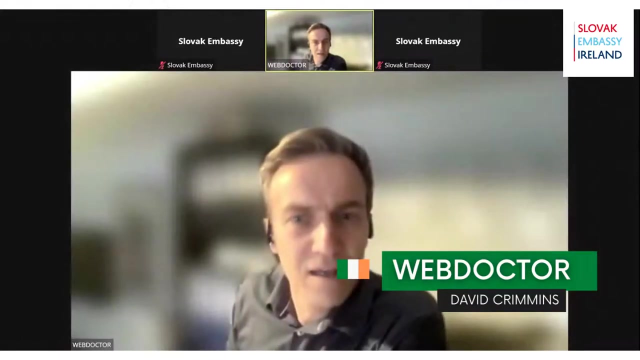 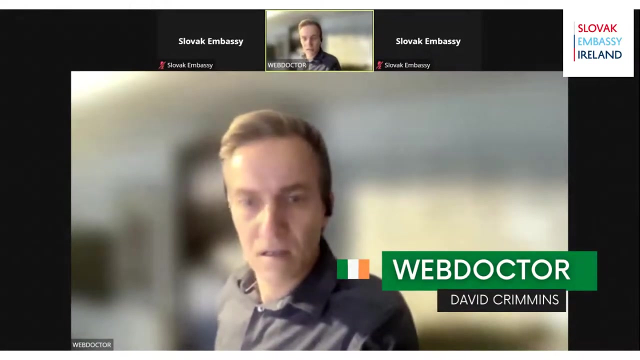 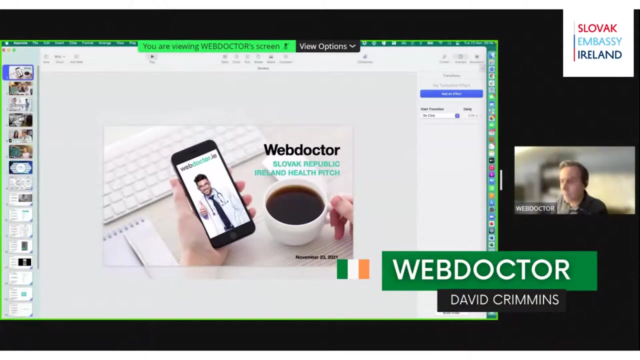 All results are reviewed when on the online consultation with one of the doctors and results are available to employees while they are patient record. you, Hi, can you hear me? Sorry, keep getting messages from. I think I'll start again. So WebDoctor was founded in 2014 with a very simple view. at the time, a GP in Dublin was 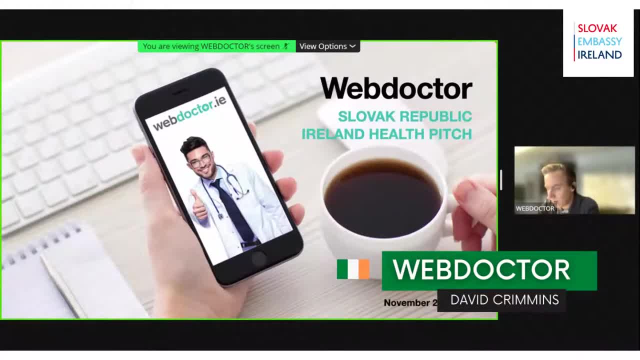 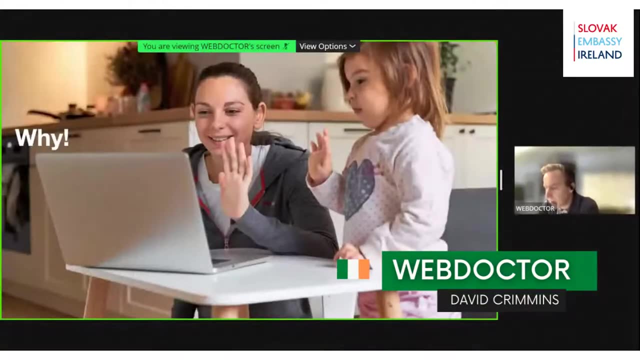 paper-based and had a couple of friends who were involved in IT and asked him to come in and help them To try and bring his surgery into the 21st century. and from those kind of humble beginnings WebDoctor was born and we have a very simple sort of manifesto as to why we get out of 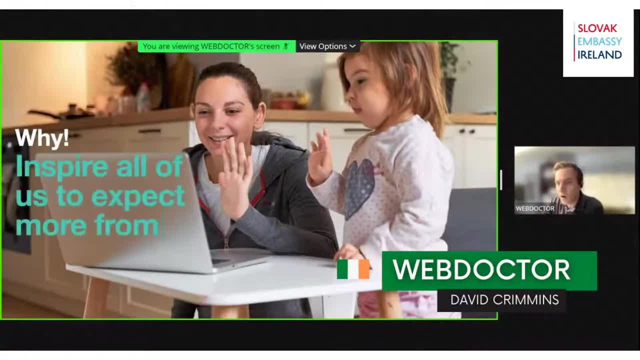 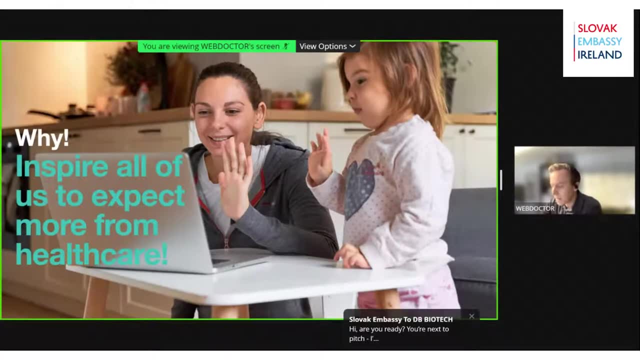 bed every day, And what we want to do is to inspire all of the planet, basically to expect more from healthcare, and we think this is a goal that is lofty, is ambitious, but actually is something that empowers all of us. So, whether there's a patient or a clinician or a receptionist, 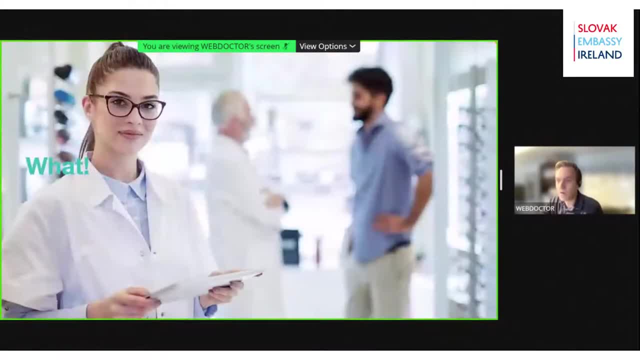 Or an administrator, or a hospital worker, et cetera. So how do we do it and what do we do? We allow clinicians to operate at the top of their license, and what we mean by that- and I think Mitchell maybe touched on this in the X-Way presentation- is that doctors. 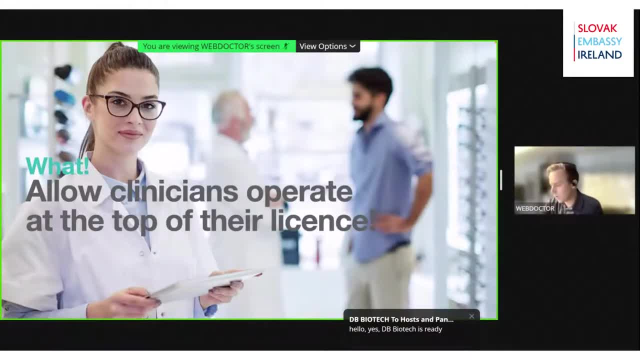 and clinicians spend a long time in medical school or interning, et cetera, and once they start working they actually stop using a lot of that knowledge and they spend a lot of their time doing housekeeping, admin And work that can be done either by somebody else or, in our case, with the help of artificial. 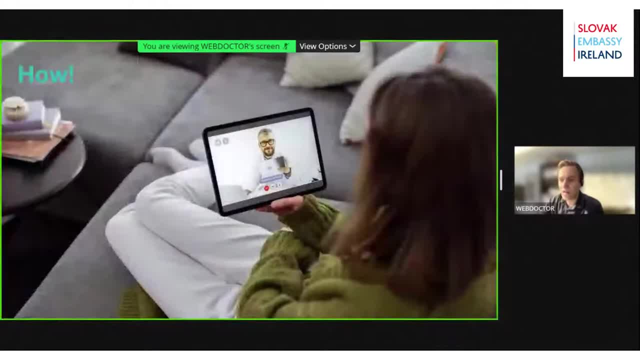 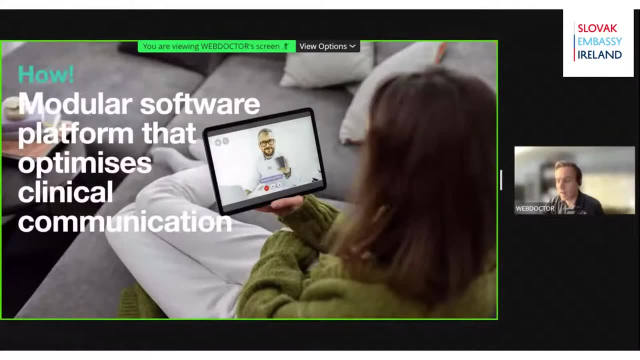 intelligence and machine learning. So what we provide is a modular software platform that optimizes clinical communication, And in the couple of minutes that we have here I don't have time to go through each of that, But basically, what that allows the customer to do is to pick and choose the elements of 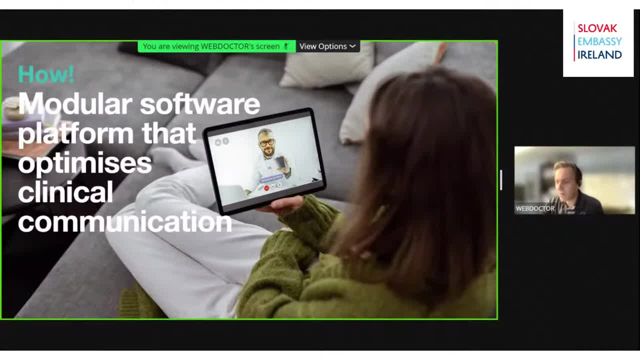 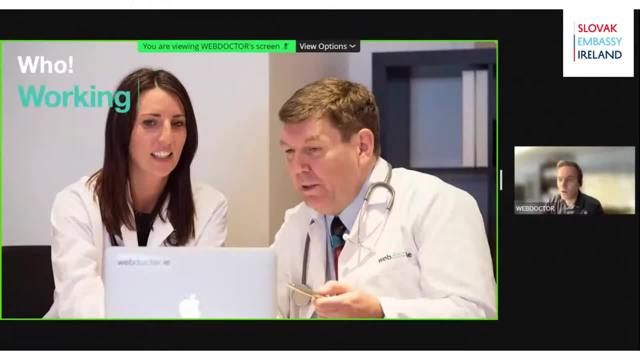 our platform That most And represent their needs in terms of how they deal with their patients. So who do we work with? We work with a couple of industries across the globe. We work with, obviously, healthcare, So you can see there the HSE, which is Ireland's national health provider. 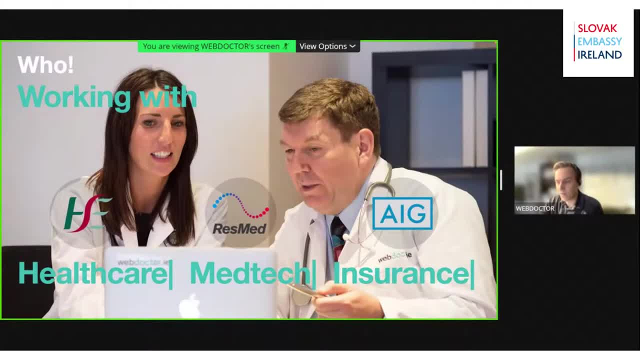 We also work with Medtech, So one of the companies we work there is a respiratory device company called ResMed. We also actually work with insurance companies- Another one there is AIG- And they might seem quite disparate, But what's common to all of those companies is that at the end of the pathway there's 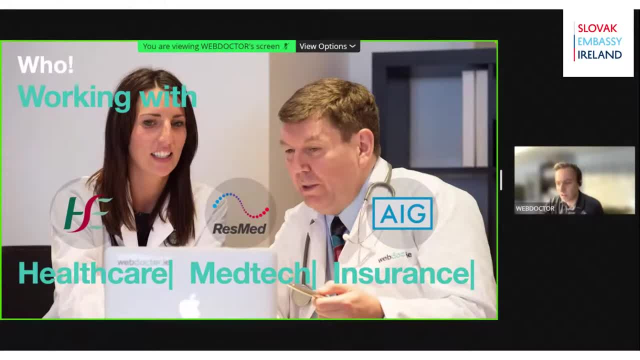 always a patient, Even in insurance. if you think about travel insurance, someone could be out of their home country and get sick and need to seek medical advice, And we work with the insurers to make sure that their patients get the medical advice that they need. 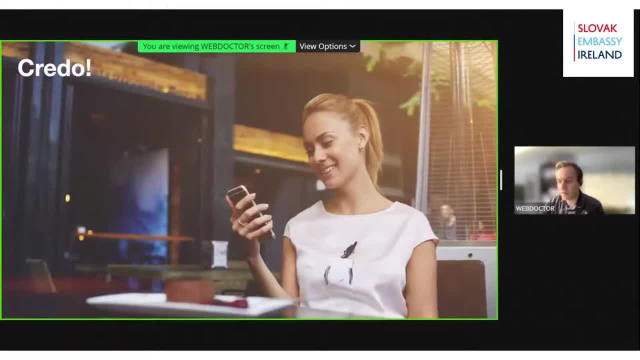 Our credo is very simple. We have a couple of principles that we stick to no matter what. So, first and foremost, we are patient centric, We co-operate, We codify all the data, And that is crucial because, by codifying the data, we allow the machine learning or the 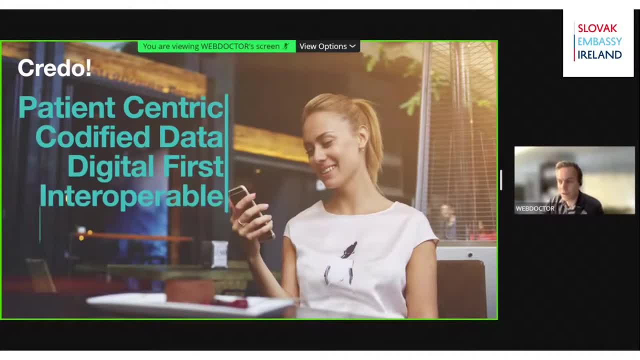 artificial intelligence to complement and support the clinician. We do not believe in replacing the clinician, but we, as I said earlier on, allow the clinician to operate at the top of their license. We're digitally first, but we're not digitally only. 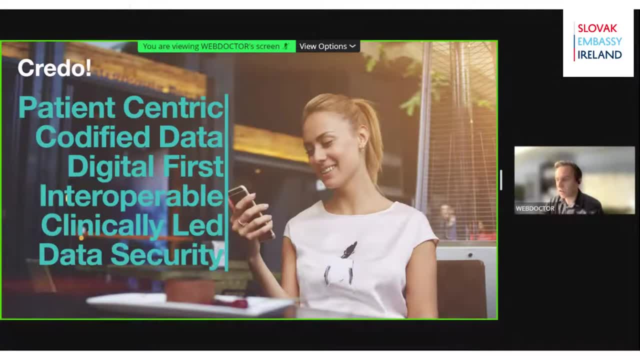 So we do operate and integrate with hardware such as CPAP devices, spirometers and another piece of hardware. We're also interoperable. So, like one of the previous presenters, we also work with fire. We can work with legacy systems from insurance companies, from health cares. 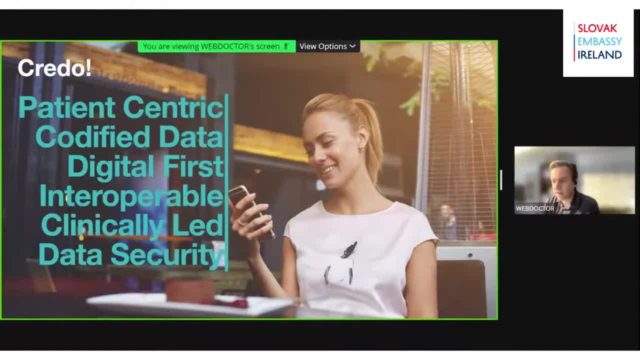 And, as we all probably know, in healthcare it's one of those industries that has a lot of legacy systems, as we all in Ireland found out a couple of months ago when the HSE got hacked. We are clinically led, So we're a software company, but at the heart of our company are clinicians. the founder. 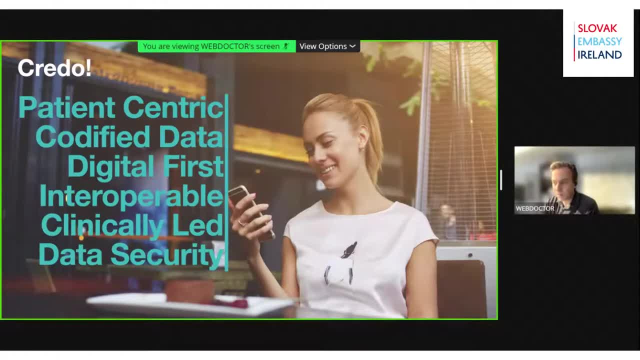 and we have 50,000 clients, So we're a software company. We have 50 doctors and nurses in our company, So it's not software for the sake of software. it's software to improve the clinician's ability to treat their patients, which improves patient outcome. 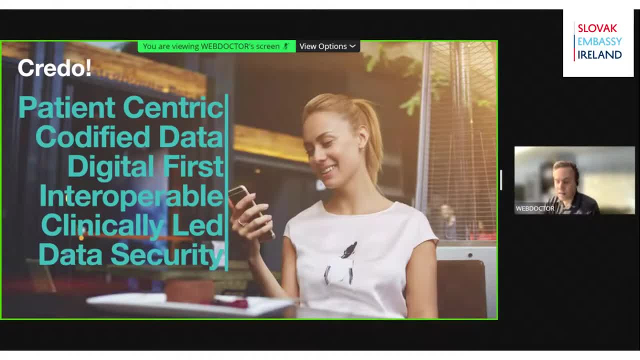 And critical is data security. We are constantly penetration tested by a number of our global customers, along with our own data security, to make sure that the data that is provided to us is safe. Our platform is, as I said, modular and I won't go through all of it, but probably what? 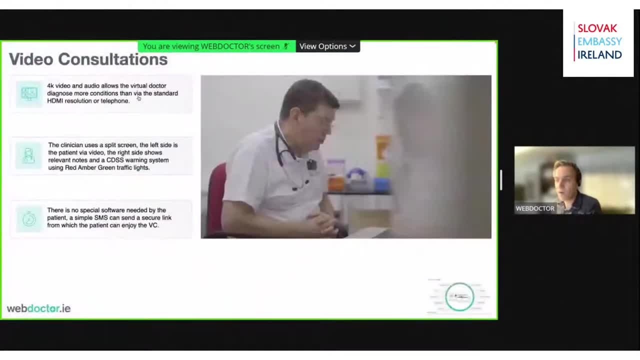 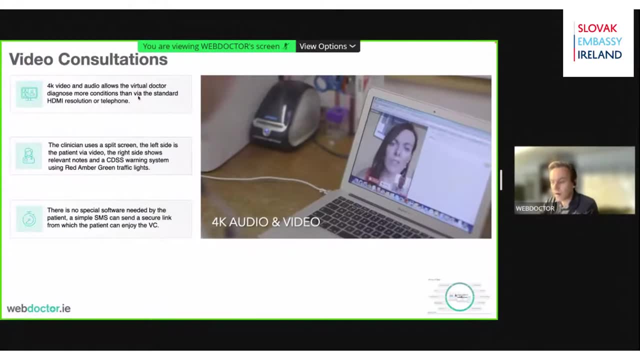 we are best known for in Ireland anyway is telemedicine And telehealth. So in telehealth we provide 4K video and audio. The audio is very important because it's 4K. it allows for doctors to pick up on quizzes. 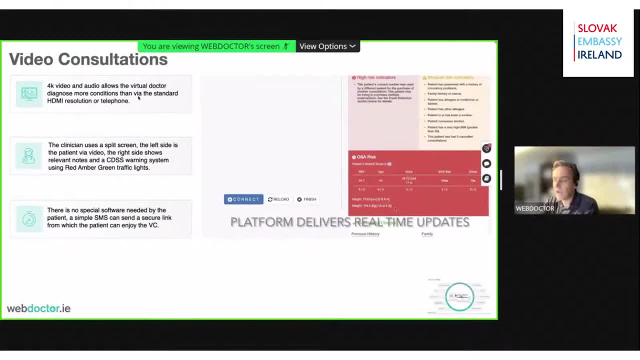 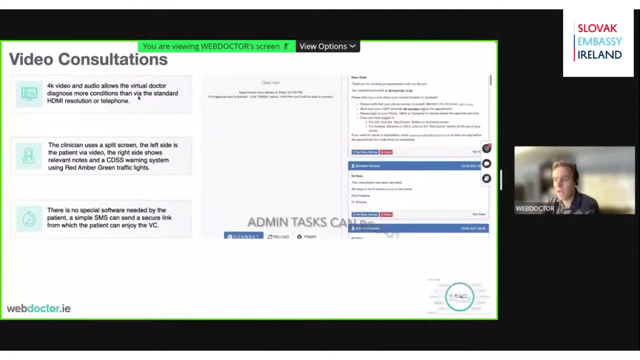 and coughs, et cetera. that's not possible over the telephone line. We have a warning system so that when the doctor is speaking to the patient, our AI is giving them real time alerts as to things that may have come out of a questionnaire. 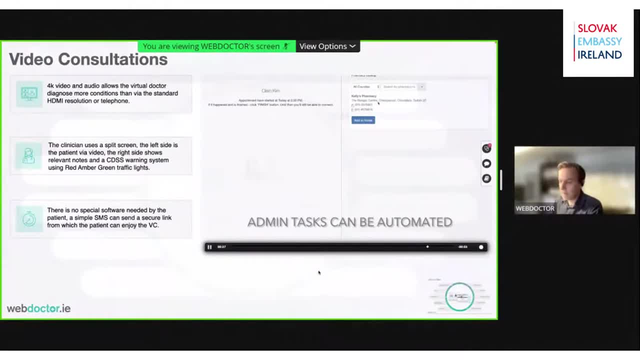 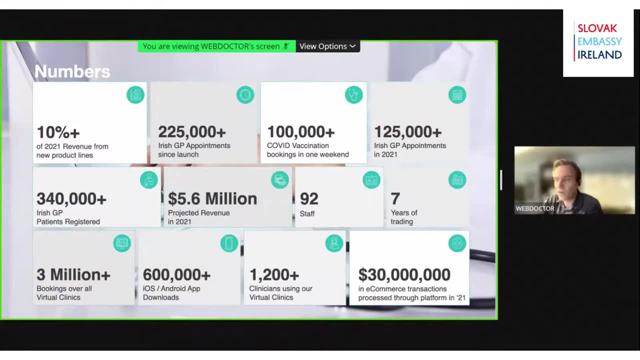 that the patient would have done prior to doing the teleconference. Finally, just to give you some sort of sense of the scale of the company, We do about 225,000 GP appointments since we launched, but given COVID and the acceleration of telehealth, probably 50% of those have happened in the last 12 months. 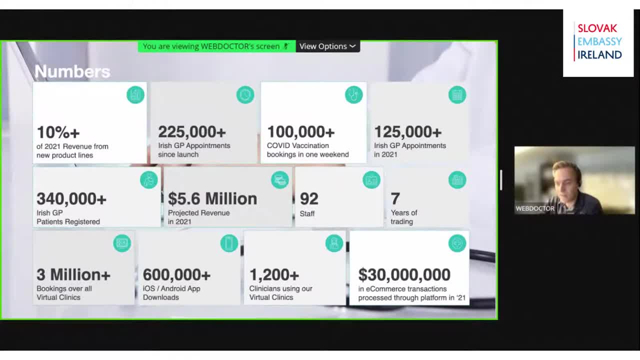 We will shortly reach a hundred staff, seven years of training. as I said, We've had over 3 million bookings on our clinics. We've over 600,000 downloads on the two various app stores. We've had over 3 million bookings on our clinics. 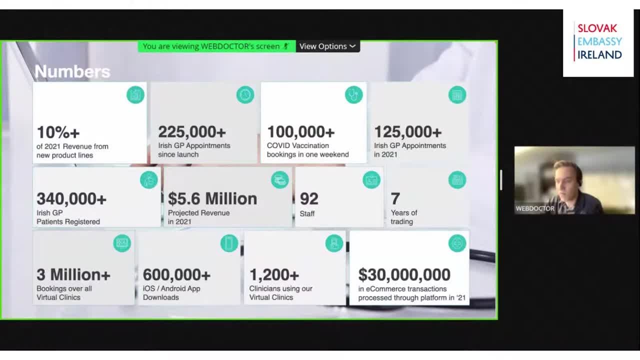 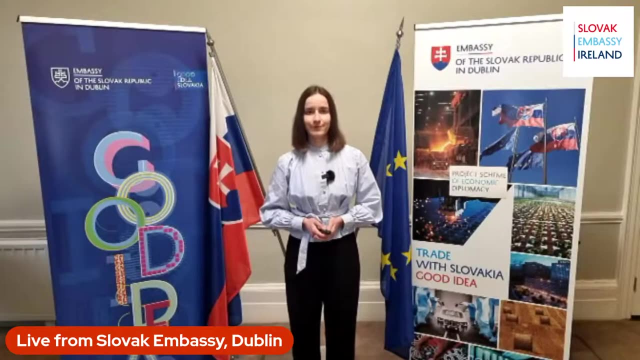 We've over 600,000 downloads on the two various app stores And we also provide an e-commerce platform to our customers, And this year alone, over 30 million US dollars has gone through that. The next presenter is Mr Jan Spivak from the Slovak company DB Biotech. 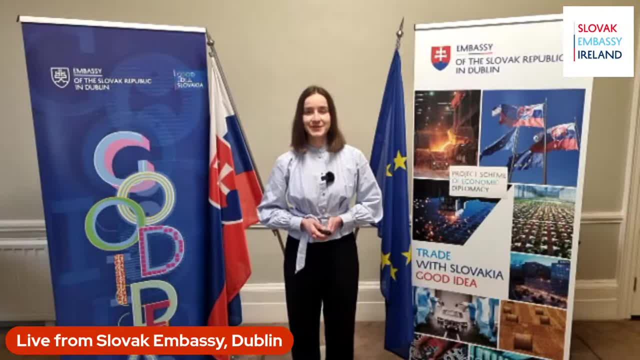 DB Biotech is focused on the design and production of high quality Arabic clonal antibodies developed by a novel and innovative technology. It's a B2B, an in vitro cloning technology, which has been developed and perfected by a scientific team over a period of 20 years. 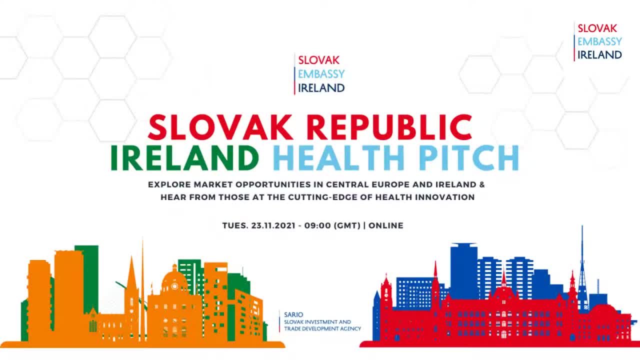 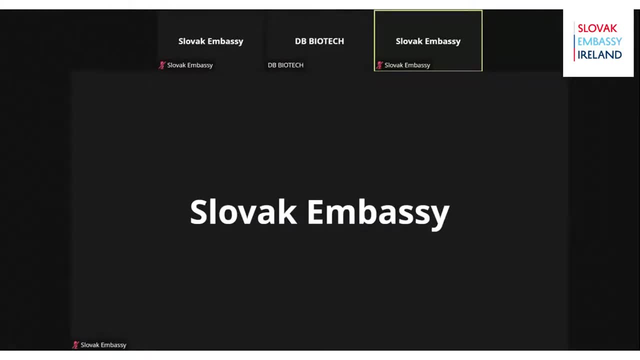 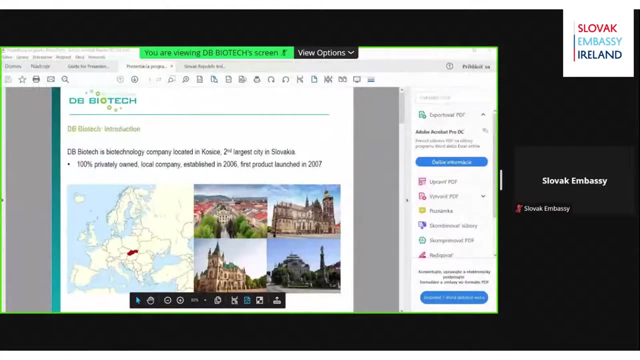 Jan Spivak, sales and product manager DB Biotech. Hello, my name is Jan Spivak. I'm a sales and product manager at DB Biotech. First of all, I'd like to thank the. i would like to thank you for the opportunity to go through what db biotech does and what are our 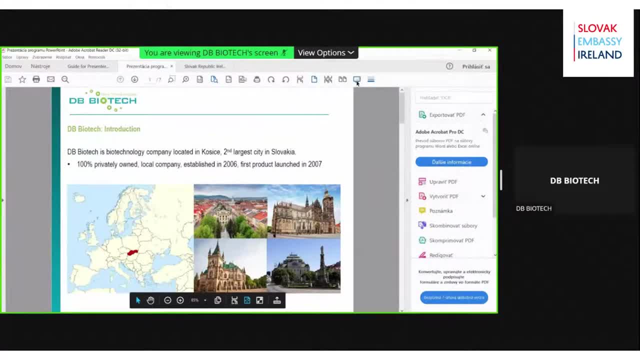 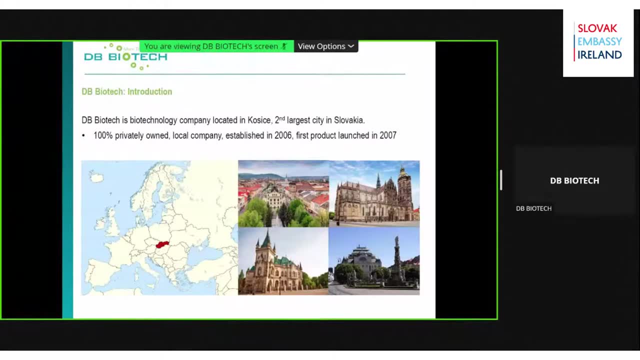 main activities. let me therefore start with the presentation itself. so db biotech is biotechnology company located in kosice, which is second largest largest city in slovakia. we are local company, privately owned. we were established in 2006 and we introduced our first product a year later, in 2007.. 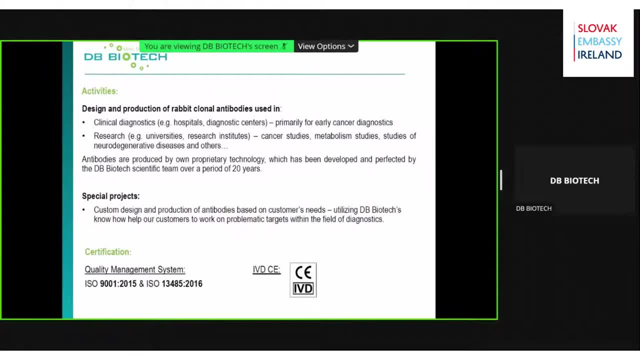 our main activities are design, production and supplying of rabbit clonal antibodies used in clinical diagnostics and research. as for the clinical diagnostics, we are mainly focused on early cancer diagnostics, so our end users are hospitals and diagnostic centers. as for the research, there are many ways how the antibodies can be used. for example, those can be used in: 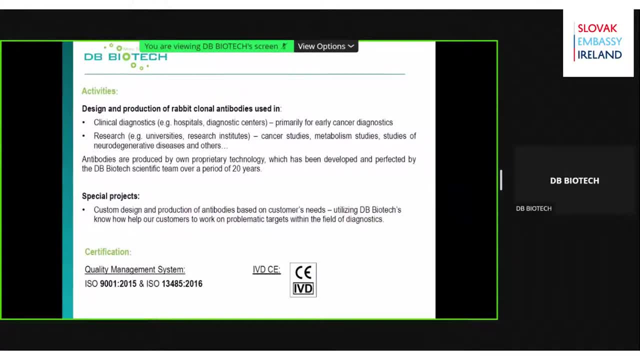 cancer studies, metabolism studies, studies of neurodegenerative diseases and many others. we produce our antibodies with our unique proprietary technology, which has been developed and perfected by our db biotech scientific team. on top of the antibodies that we have in our portfolio, we are able to design and produce the antibodies based on the specific needs of our 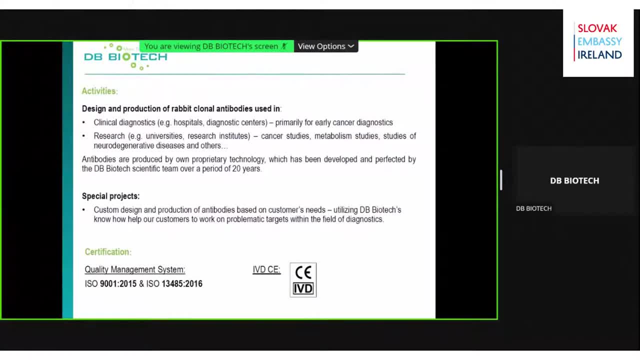 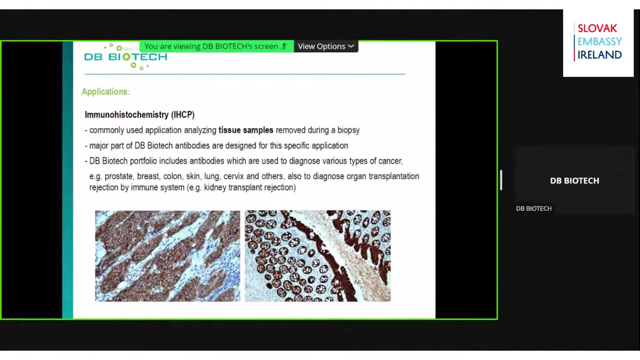 customers, so-called special projects, where we help our clients with diagnostic problematic targets by utilizing our know-how. we are ceivd certified and we also hold uh iso quality management system certificates- uh nine, zero, zero, one and a thirteen, four, eight, five, speaking about the applications where our antibodies can be used. 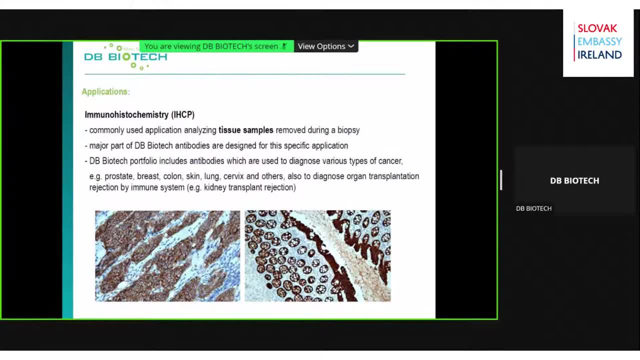 so the first and major one is immunohistochemistry, which is a popular application that analyzes the tissue samples removed during the biopsy. also, major part of our portfolio is designed specifically for this application. our antibodies can be used for many different kinds of diseases, be used to diagnose many types of cancer, for example, prostate, breast, colon cancer, skin, lung. 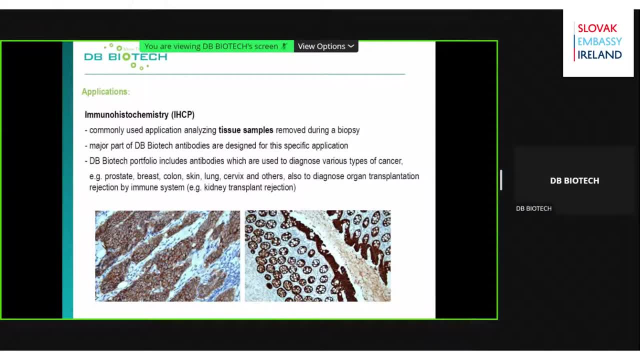 cervical and others. we do not talk only about the cancer but, for example, with our antibodies we can diagnose whether the immune system is accepting or rejecting the origin after the transplantation, for example the kidney. as for the illustration below, we have two pictures of human tissues. the left one is breast tissue and the picture on the right is cone tissue. both issues show that cancer. 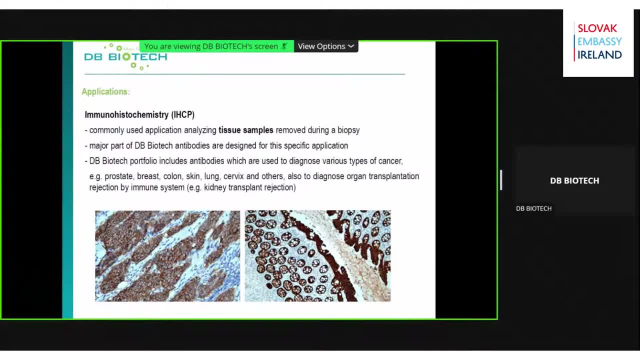 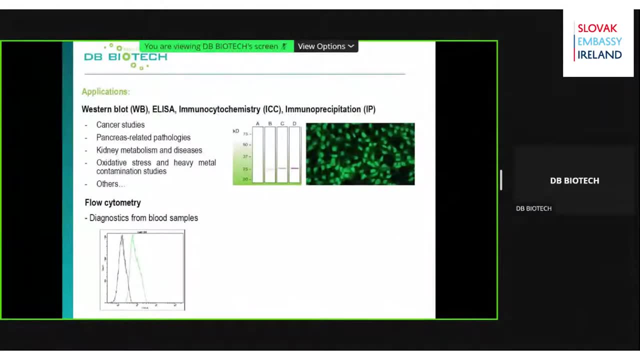 process is already ongoing and those are the brown cells, or brown parts, which were marked by using our antibodies. speaking about the other applications, those are western blood, eliza, immunocytochemistry, immunoprecipitation or flow cytometry. again, there are more ways how the 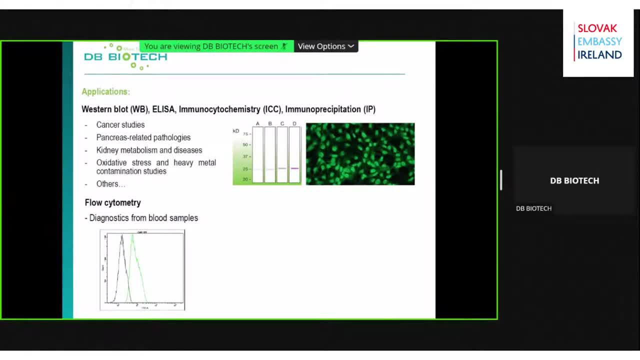 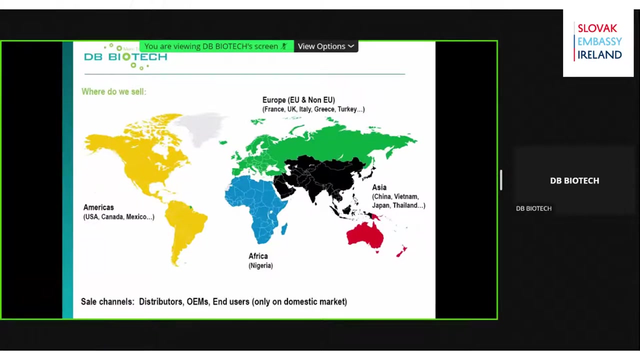 antibodies can be used for, for example, we can speak about cancer studies, bankrupt creos, related pathologies, kidney diseases and others. as for the flow cytometry, the diagnostics is done from blood samples and from the. for example, this is an option how to diagnose leukemia. we supply our products to more than 30 countries worldwide as we are european company major part. 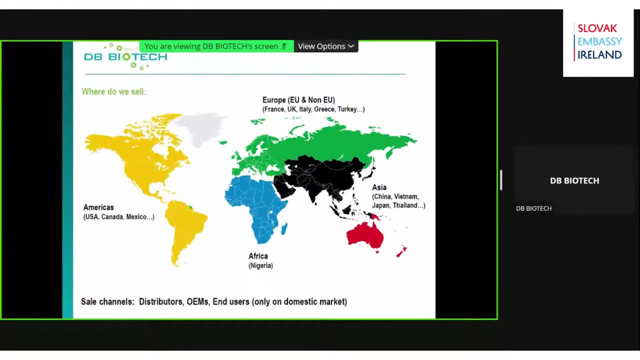 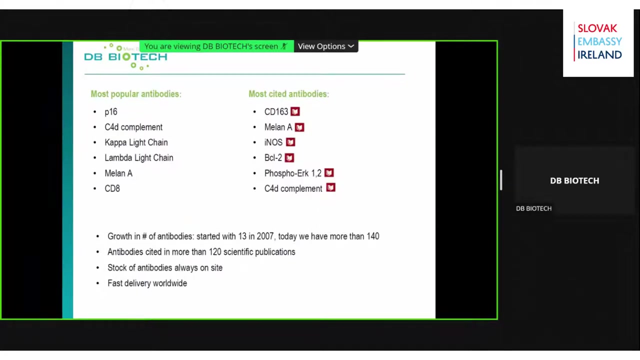 of our revenue is generated in europe. we are active outside of europe as well, for example, in asia, us, canada, mexico and africa too. we sell our antibodies via distributors and oem partners. we provide products to end users only on our local domestic market. here's the short list of some of our popular antibodies and most cited antibodies. as for the 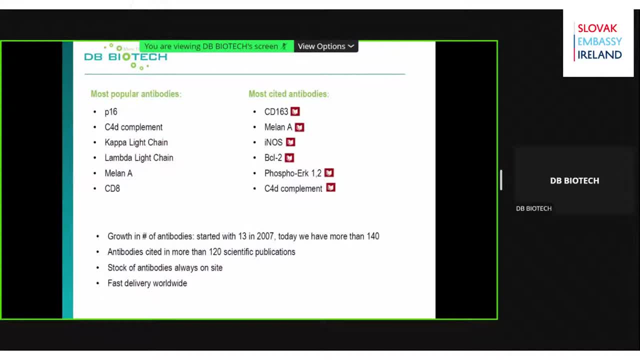 citations: our antibodies are mentioned in more than 120 scientific publications. to this day, we have more than 140 antibodies available that will be produced by our technology. as we are the manufacturer, the products are always available at our site, ready to be supplied worldwide within the short period of. 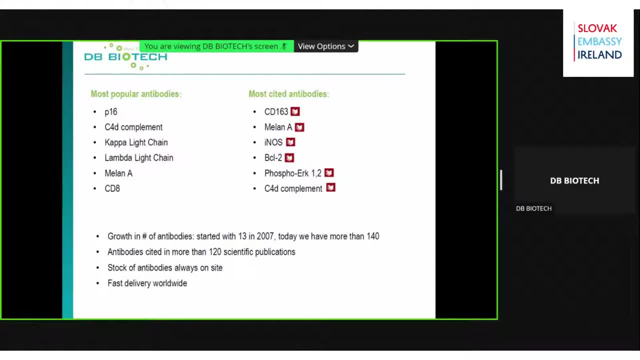 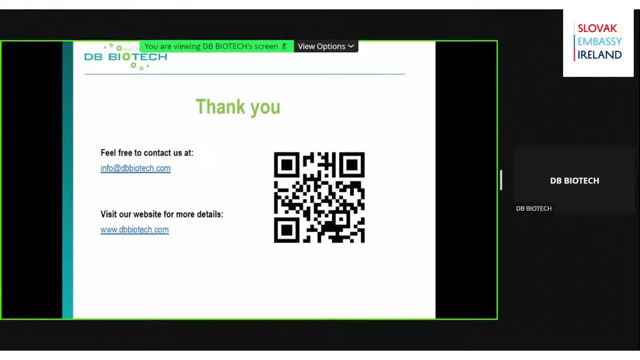 time, as we work with major shipping companies. in case of any questions, you can contact us at email address: info at dbbiotechcom. we'll be happy to provide you any further information. you can also visit our website at dbbiotechcom for more details about our products. thank you once. 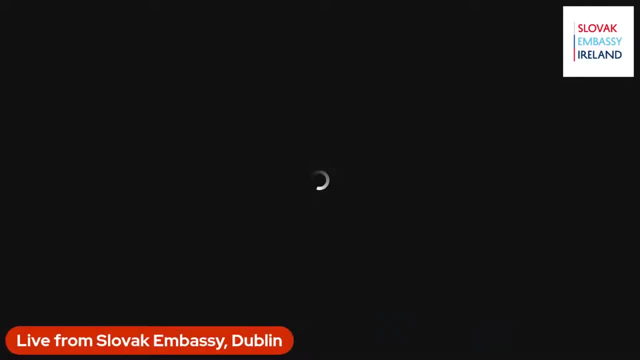 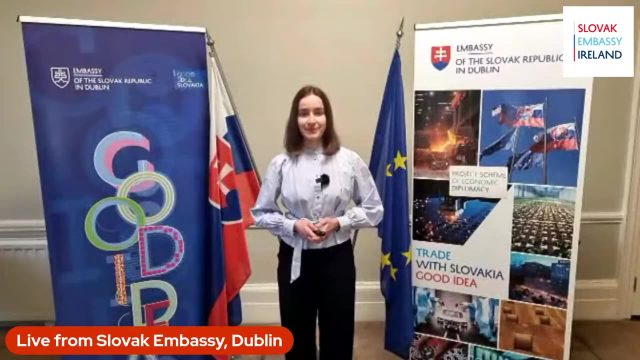 again for your attention. the tenth presenter is mr laun atkins, from the irish company impact privacy. impact privacy provides compliance as an outcome for privacy and data protection. the main task of the company is to help clients to better manage privacy risks. businesses supporting healthcare across europe and north america. 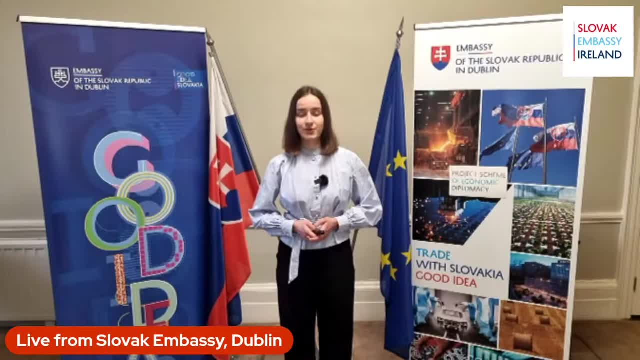 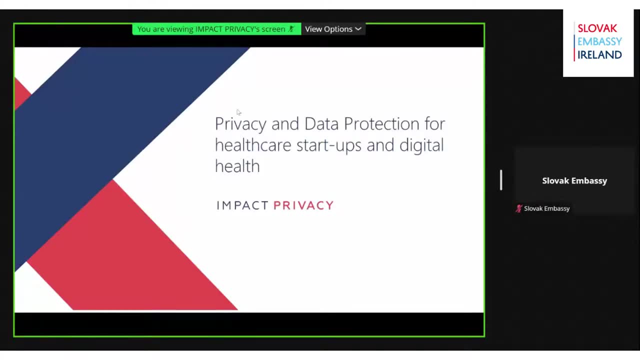 to give confidence that the privacy risks are being properly addressed and the needs of the community at large are extremely important. thank you so much. thank you so much, mr leonard. thank you so much and thank you for the one minute meeting, yeah, and thank you for your time. thought a lot. thank you so much and thank you very much. 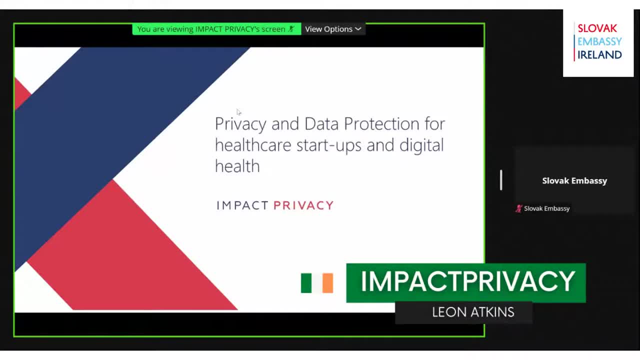 you know, we've been hearing for over a year now. it's been a very fun conversation and i'm sure a lot of us have seen this particular coven and it's been a wonderful beginning to all of you and for those of you that are new to this. um in the field of data science and Peggy that we performed. 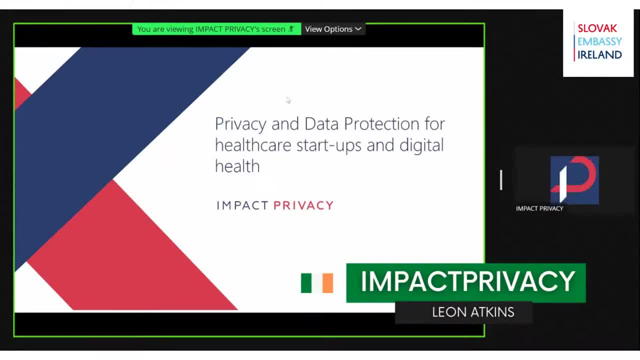 in recent years. with the new address fft, we have a security issue that we're going to see if we're going to Good morning from Dublin. My name is Leon Atkins. I'm the CEO of Impact Privacy And when we launched Impact Privacy in 2019, just two years ago, we knew that you had plenty of things as healthcare startups and digital healthcare businesses, and even established businesses, to think about before your products or new products were investment, patient ready. 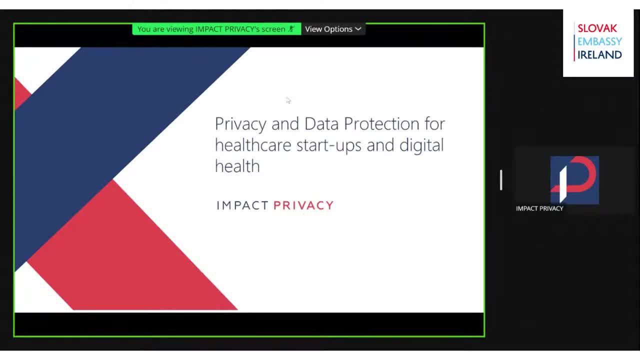 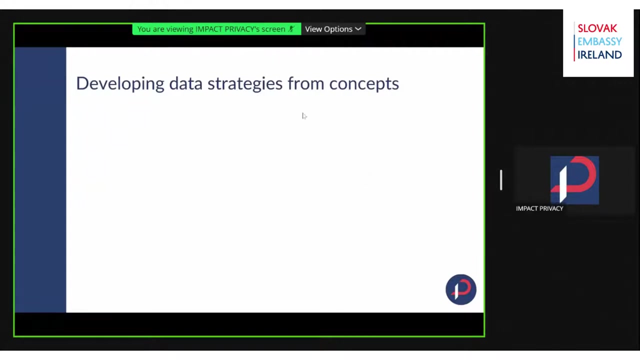 including the trustworthy and compliant use of health data. Impact Privacy is a healthcare solutions business, and we have a three-step support program for healthcare startups and digital health designed to help them deliver. Ensuring the technical design of your healthcare solution is privacy friendly means getting to grips with data strategies for the product. 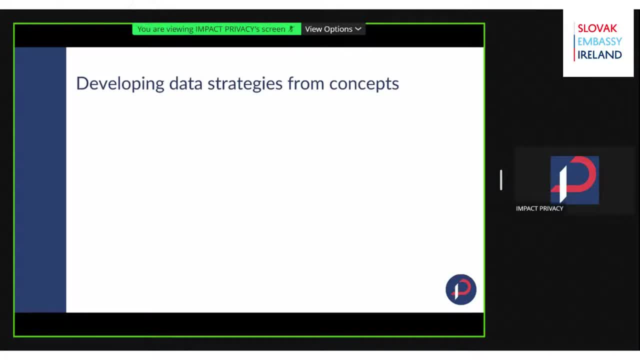 From the moment of its conception, we work with healthcare companies and digital health companies to identify privacy by design strategies and technical goals, starting with a privacy risk assessment of the concept. We provide your team with privacy insights essential for delivering a product that minimizes, separates, abstracts and hides personal data. 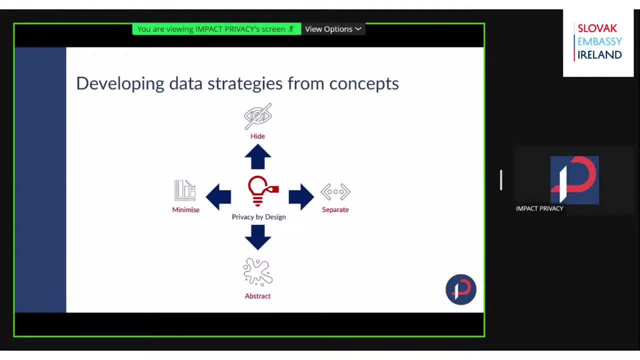 And the whole idea of that is to give you an outcome. We provide a clear product roadmap that supports ultimately the design and development phase of your product. But privacy and data protection requires more than just implementing a responsible solution designed to underpin your healthcare product. 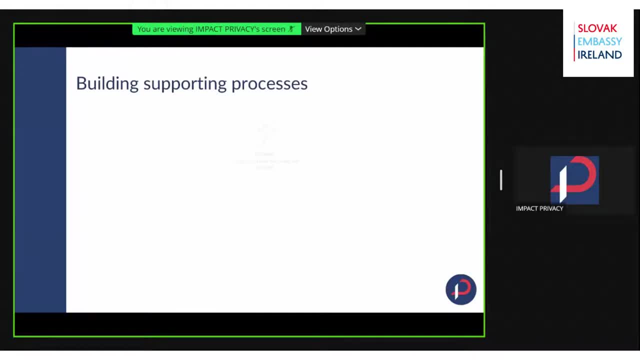 It's also about ensuring the use of health data meets established privacy principles. So we help you demonstrate your solution is built on a sustainable foundation For future growth and development and meeting your healthcare objectives, like some of those you've heard about this morning, with a framework to support privacy goals. 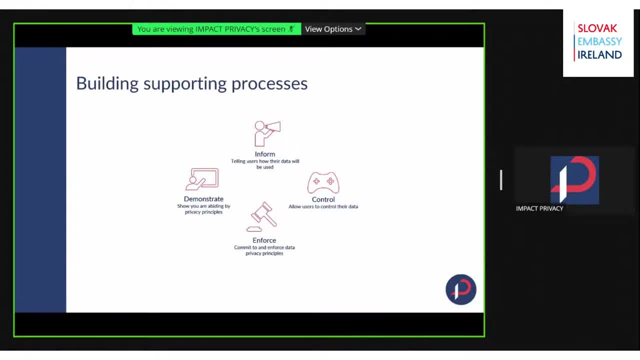 We help you design a process framework that delivers trustworthy and compliant use of personal data. But, of course, you have a business to run and you have your own vision and objectives to meet the needs of your patients and their outcomes, So we want you to focus on that. 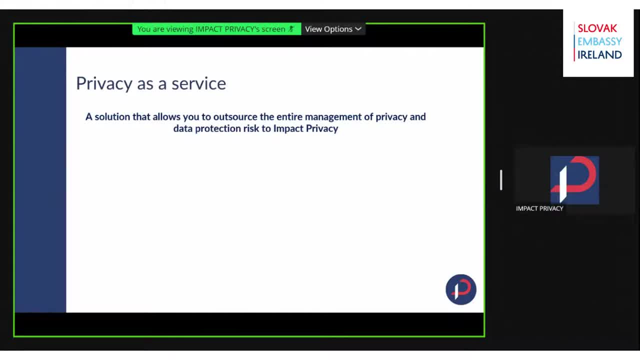 So we're about providing a solution that allows you to outsource to us the management of your privacy and data protection risks, relying on our healthcare credentials, which we've built up over our focus on healthcare over the last two years, Supported by the multidisciplinary expertise of our team in privacy, security, technology, legal risk. 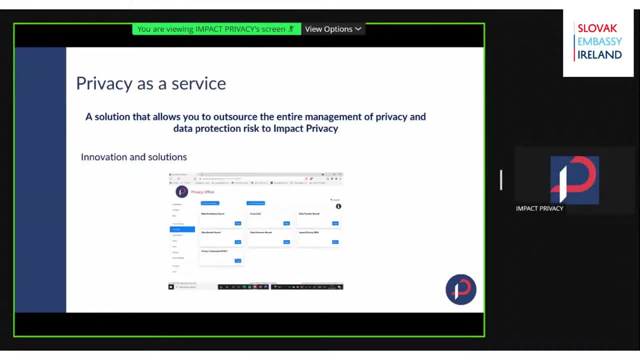 and operations, as well as our full suite of innovative solutions, including proprietary privacy management software that is unique to us and designed for the healthcare sector specifically, and we have a unique multinational presence and capabilities specifically made to allow our clients to expand into the main jurisdictions for healthcare growth and expansion, where the big markets are. 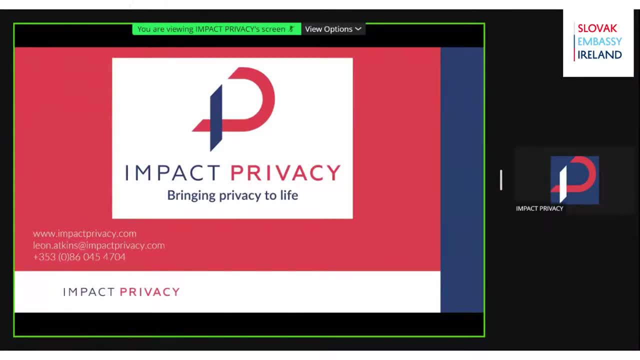 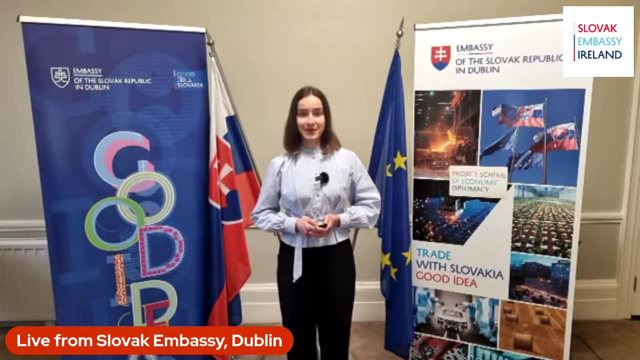 if we can help you, we'd love to be able to help you and we'd certainly like to help you with your visions and objectives. like us, we want to bring privacy to life. thank you. the 11 presenter is mr derma dempster from irish company clonalone. clonal manufacturer is focused. 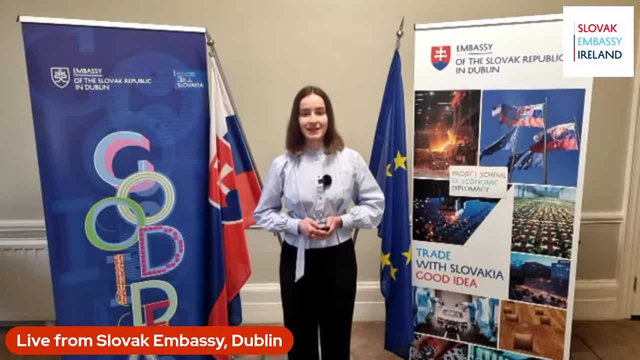 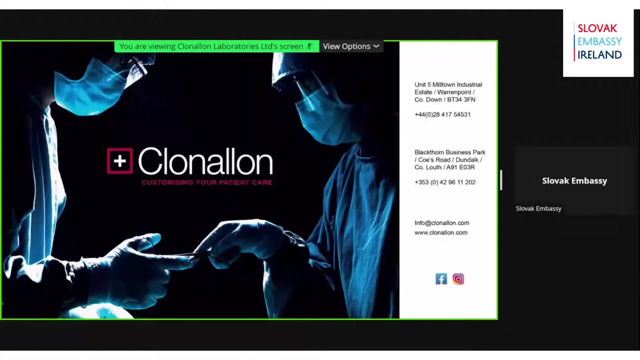 on the clean rooms customized surgical tray sets and distributes these for use in hospitals, general practitioners and dental surgeries. all company products bear the ce. all senior members of clonalone staff have over 60 years clinical experiences in providing clinical solutions. we can't wait to see your stories and we encourage you to tune in, see more and contact the brenda. 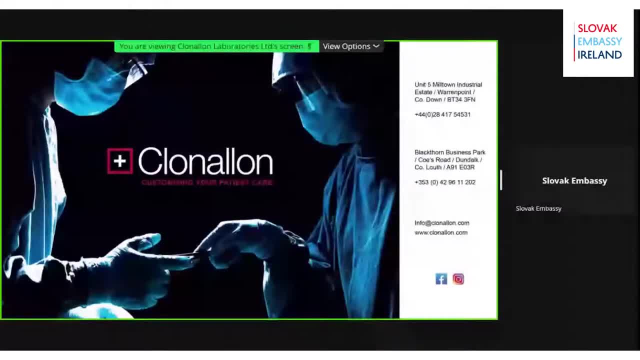 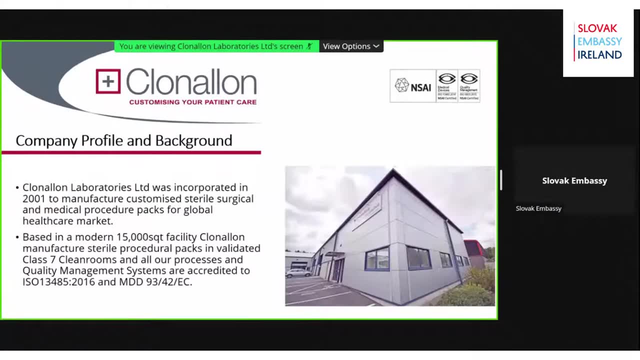 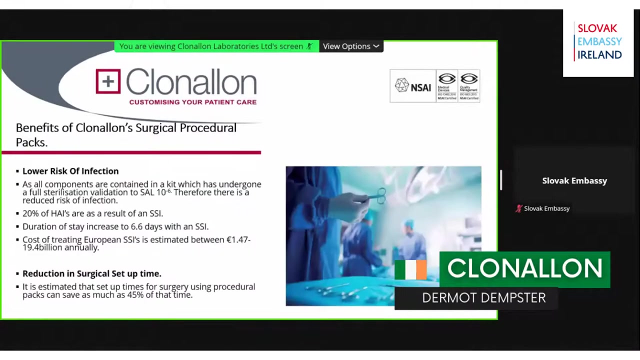 and her team for more information. thank you, and we look forward to seeing you on the screen. thank you. Customized procedural packs is to lower the risk of infection. Almost 20% of hospital-acquired infections are as a result of a surgical site infection. 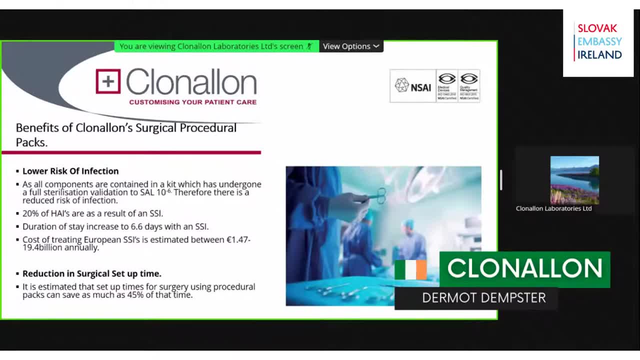 With the use of procedural packs. all the components required for the procedure are contained within the kit and have been subjected to a full sterilization validation process. Patients who contract a surgical site infection will stay, on average, 6.6 days longer in hospital than is otherwise the norm. 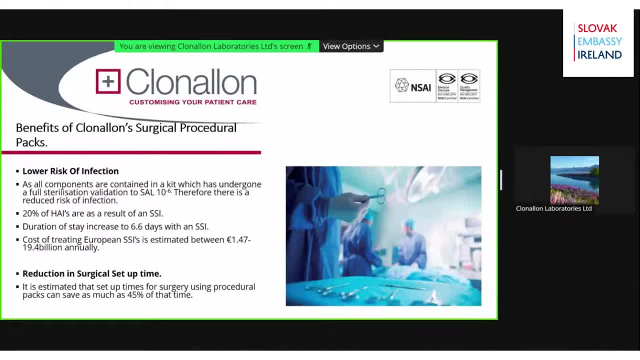 This constitutes a significant burden on healthcare budgets. SSIs are grossly underreported. The EU spends somewhere between 1.47 and 19.4 billion euros annually in treating SSIs. Many hospitals across Europe will still use surgeon preference cards that specify the 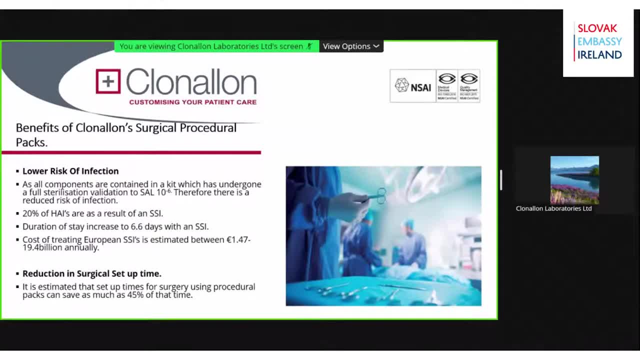 components that a surgeon will require to carry out a procedure. The average procedure will require 20 to 40 different components that must be gathered prior to surgery. This takes up very precious, valuable time. Very often a key component is not available and will result in the surgery being cancelled. 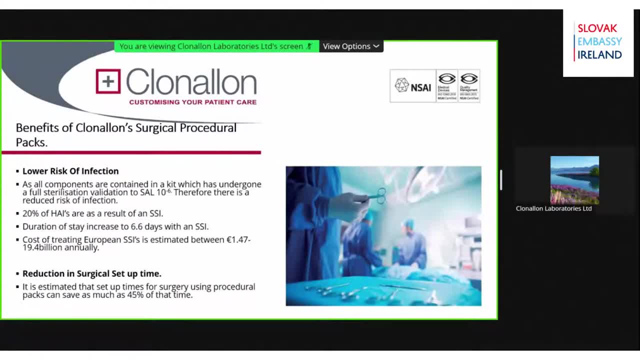 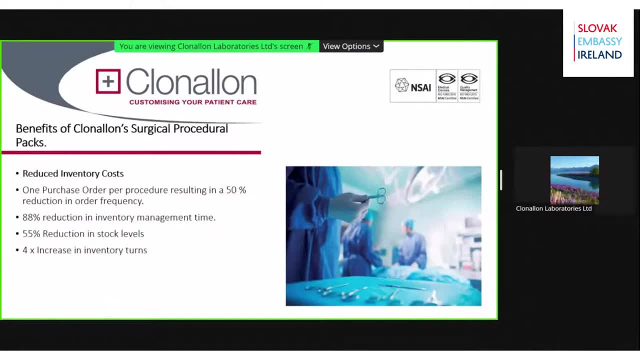 With the move to the use of surgical procedural packs, the time taken to set up for a procedure is reduced by 45%. With the use of Clonallan surgical procedural packs, there is only one purchase order required per procedure. This results in greater procurement. Clonallan Surgical Procedural Packs can be used in a variety of ways. For example, in the case of Clonallan Surgical Procedural Packs, there is only one purchase order that may be used, and among these two is one that is best suited to all procedures. 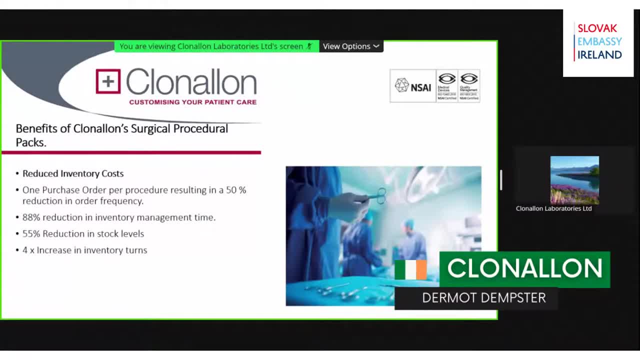 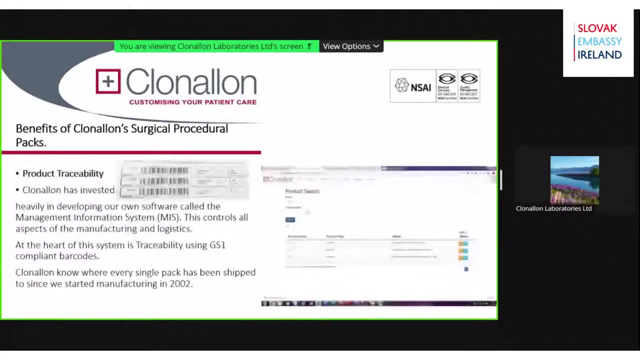 up to 3 and the second a change in the place where it has to do with the lab conclusion, to ensure a notification with the much larger HoC 3.1nt. five percent reduction in stock levels while at the same time increasing inventory turns by a factor of 4,. 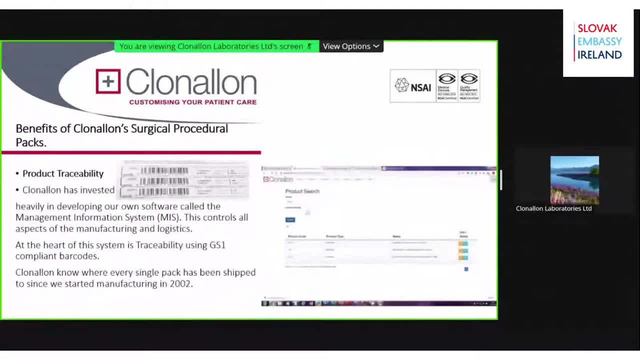 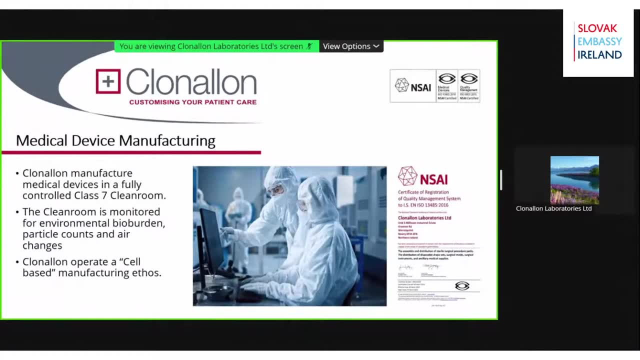 and for many other procedures it does not have. Clonallan has introduced GS1 compliant barcodes on all its products. for fullد seniors brush, 260 0000달러 facilities are accredited to. um are audited by our nsai, a notified body to iso 13485 and 9342 eec. 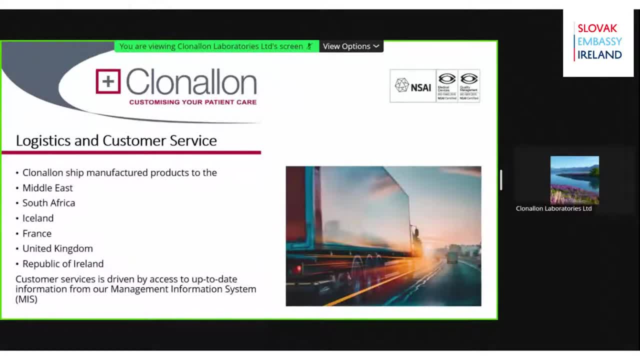 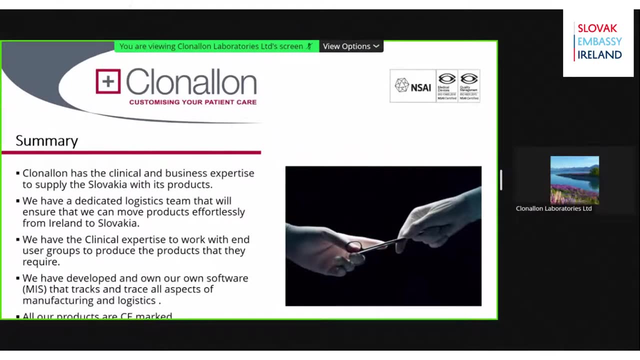 canal and serve customers right across europe and under the northern ireland protocol allows us to access both the eu and the uk markets. so just to conclude, canal has the clinical and the business expertise to supply additional vacuum market with our product range. we have a dedicated logistical and regulatory team that will ensure 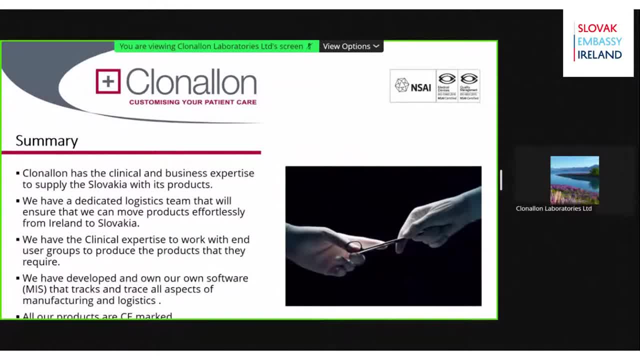 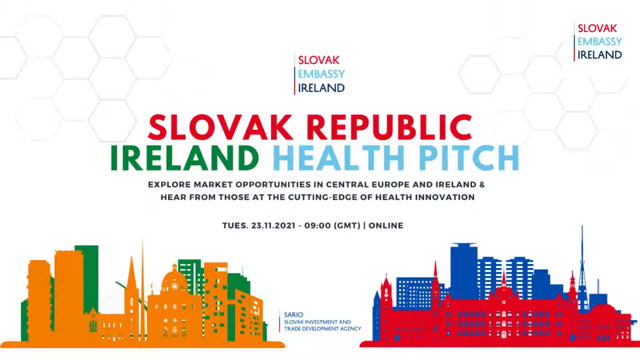 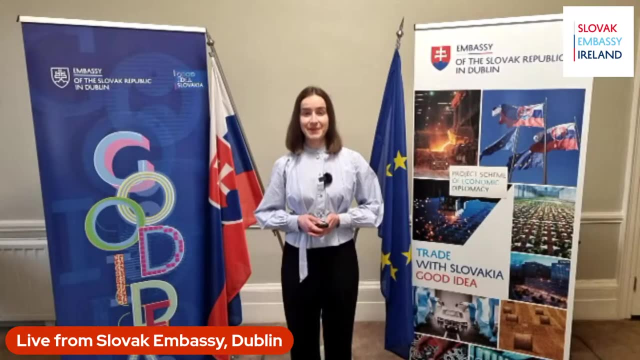 a smooth introduction of our products to the market. all our products are cd marked and we look forward to introducing canal's products to the market. thank you, then. the 12th presenter is mr peter polak from the slovak company unimed pharma. univet pharma is focused on the development and production of generic ophthalmic products. 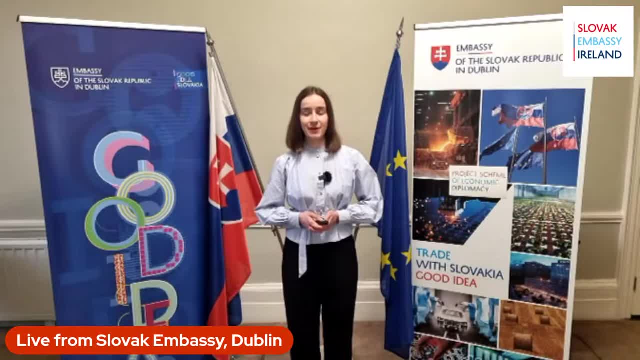 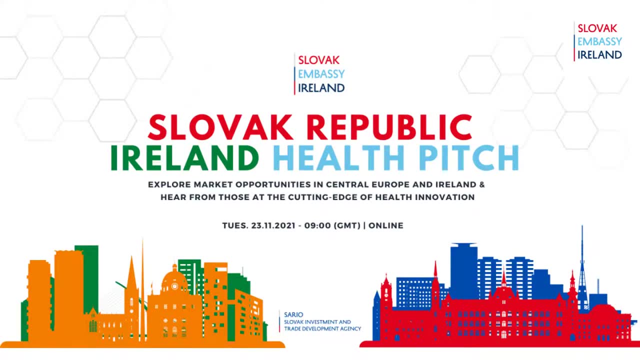 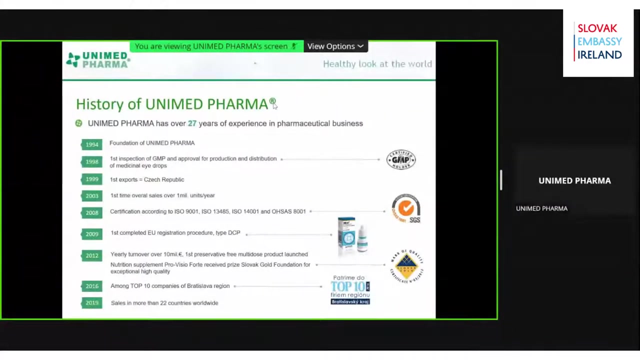 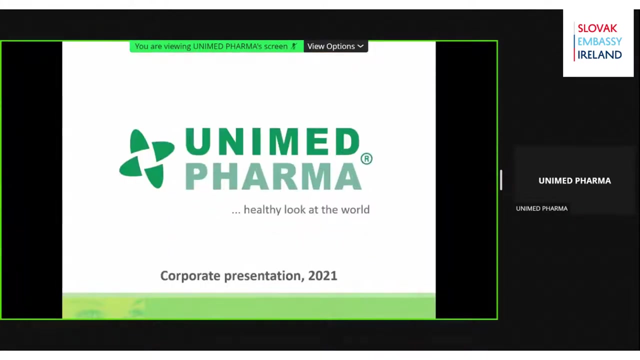 the company develops, manufactures and supplies of atomic trucks from a range of chemical materials, such as: So one more time, hello everyone. my name is Peter Polak and I work as a business development manager in Univet Pharma and, as you can see, our company is focused on bringing healthy. 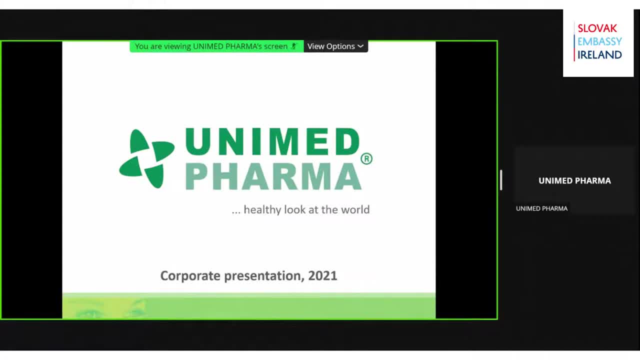 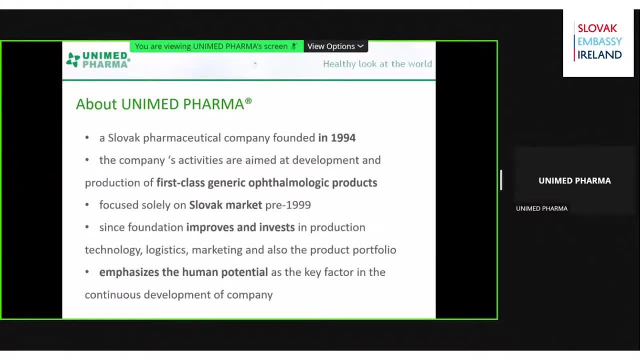 look at the world for the patient. We were established in 1994 in Bratislava in Slovak Republic by a Slovakian pharmacist and since then we produce only generic ophthalmological products and we try to expand on other markets since 1999.. 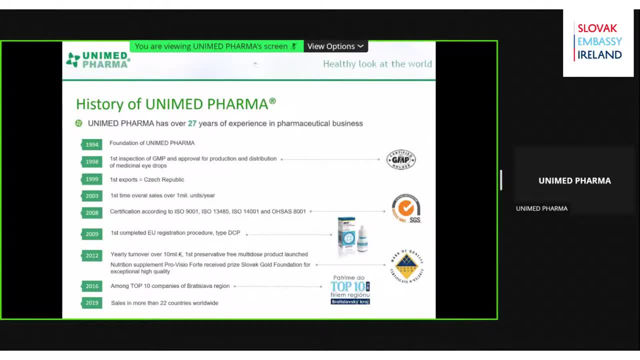 Here you can see a short overview About our achievements during our history. we are on the market more than 27 years so far, and the main achievement was expansion. as I said on other markets, We wait till the original product finishes with the patent and then we manufacture our 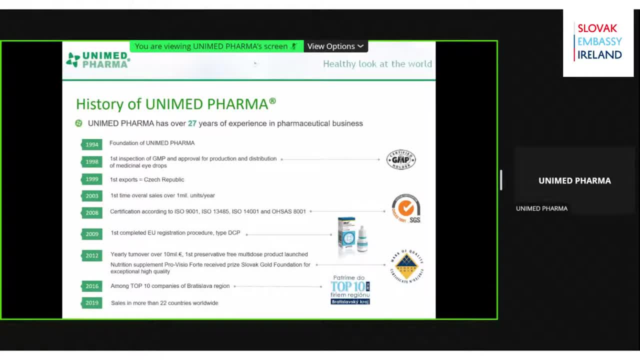 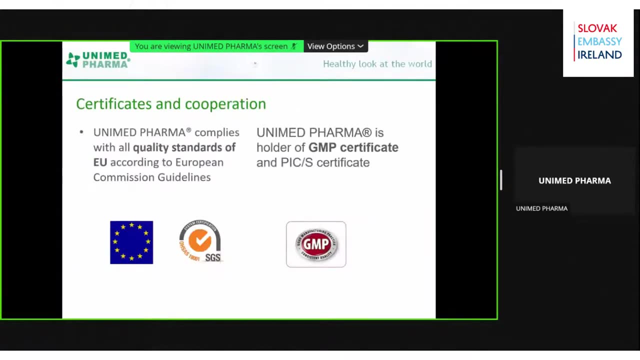 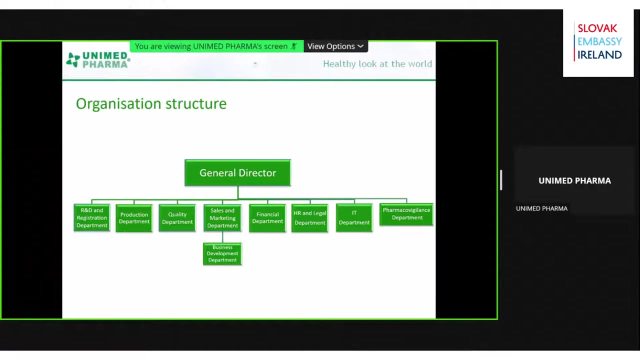 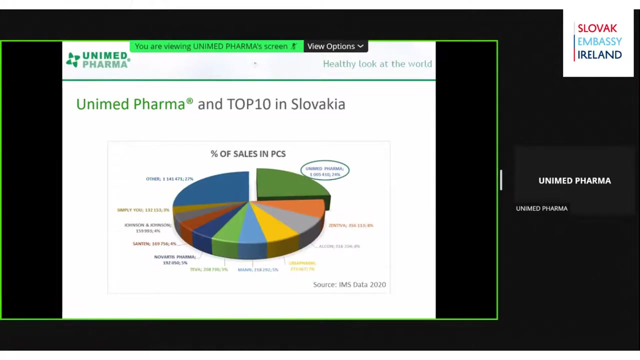 product and register it on the markets where we want to sell. You can see that We also receive the prize for high quality of our nutrition supplement for eye. We emphasize on development and production of innovative products. And to give you an overview how big we are on the domestic market, we are a leader with 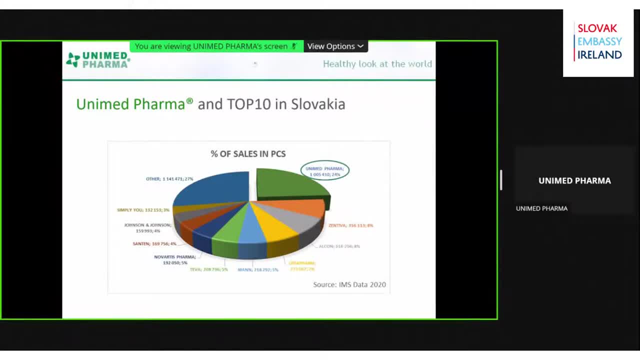 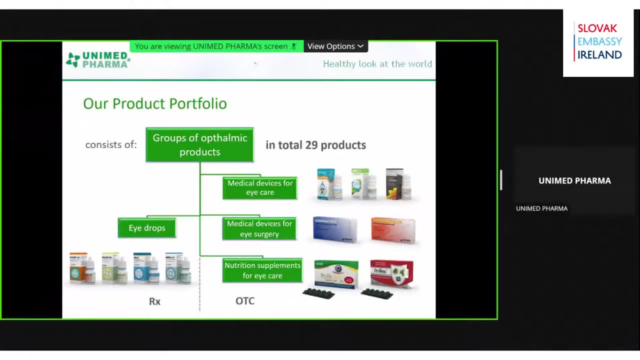 market share of 24%. So we are on the domestic market We are a leader with market share of 24%, So this can give you quite good overview. As I said, we have in the product portfolio new products and we divide it between Rx Products. 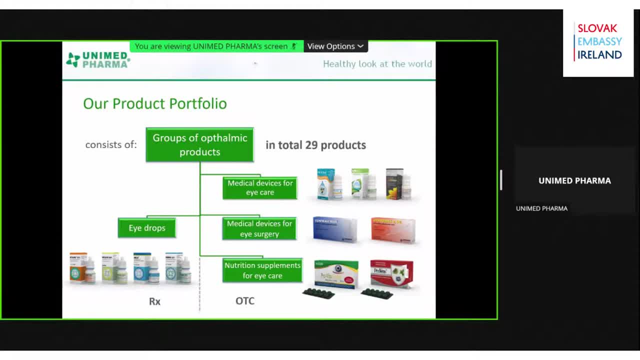 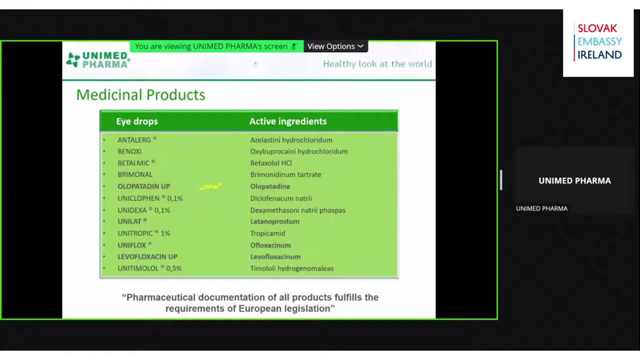 and OTC Products. There are half and half-, I would say- in terms of market share, and we have for each therapy one medicinal eye drop Product. I would emphasize mainly Olopatadine, our first preservative-free medicinal product that we launched this year. 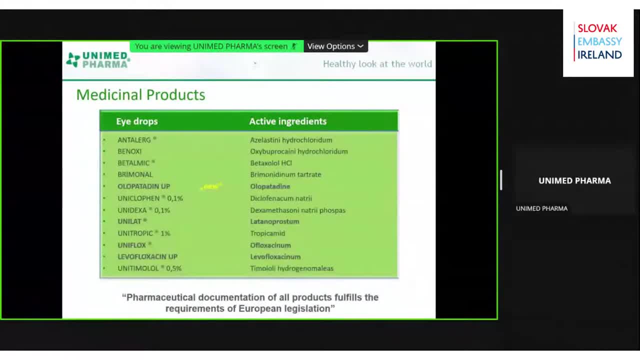 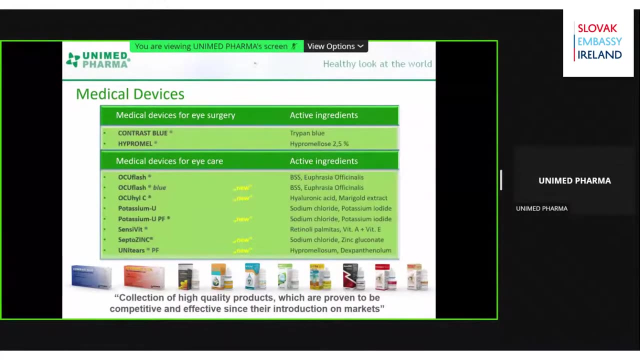 And so we are almost at the same level as top end leaders on the European market. From medical devices that are not prescribed, we have for the eye care and for the eye surgery. Again, the innovation in the market is to have preservative-free eye drops, and all that have a mark new are preservative-free. 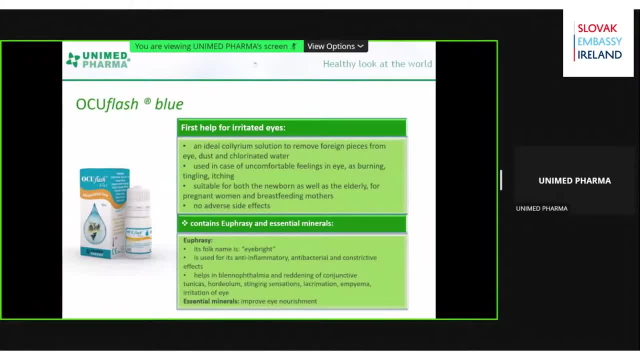 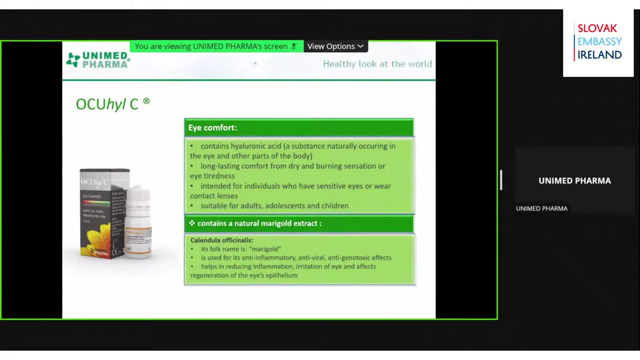 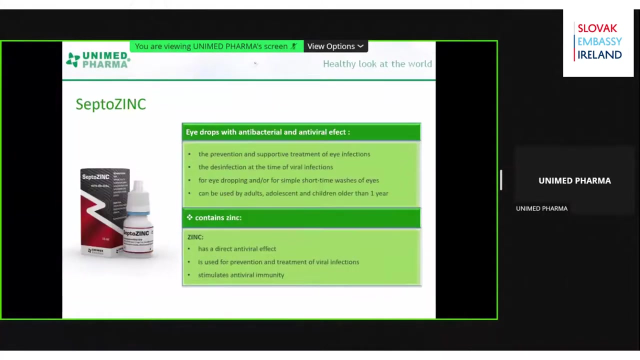 So I would pinpoint mainly OcuFlush. This is a product for newborns with the antigen. The extract from Euphrasia is very popular among patients in the markets where we sell For the dry eyes. we have also a product with hyaluronate acid and calendula extract which is also for top end consumers on the market. 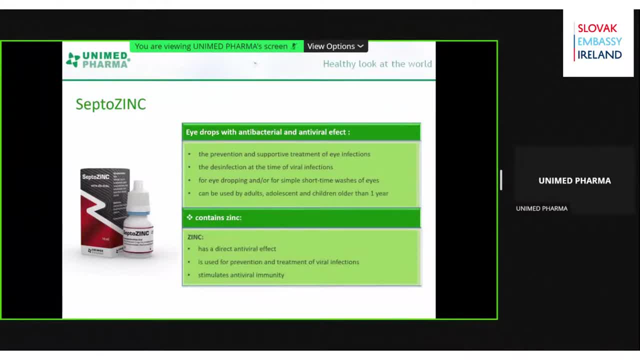 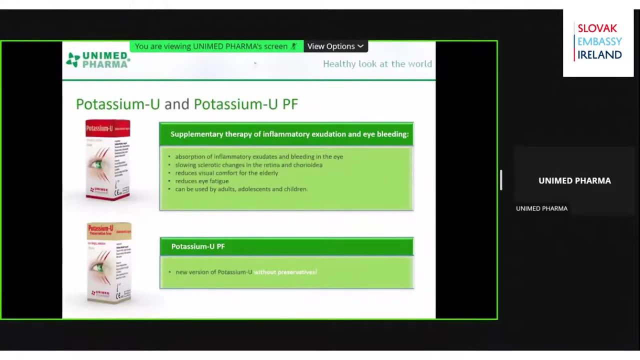 Due to COVID crisis, we developed these new eye drops. This is the product that contains zinc and it acts antiviral in the eye and as a prevention against viral infections. For the red eyes, we have Potassium-U, which is also preservative-free. 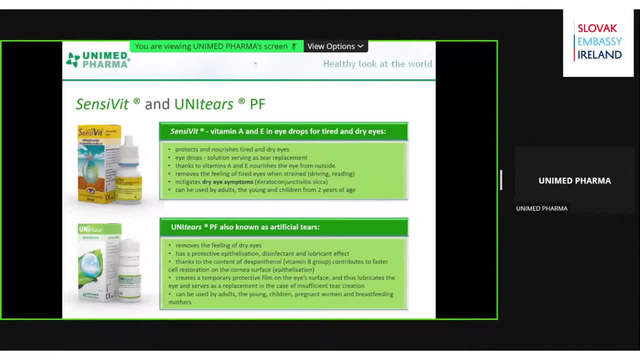 And for dry eyes we have two possibilities with vitamin A and E-Sensivit or uniters with expantanil Impromalol. And for dry eyes we have two possibilities, with vitamin A and E-Sensivit or uniters with expantanil Impromalol. 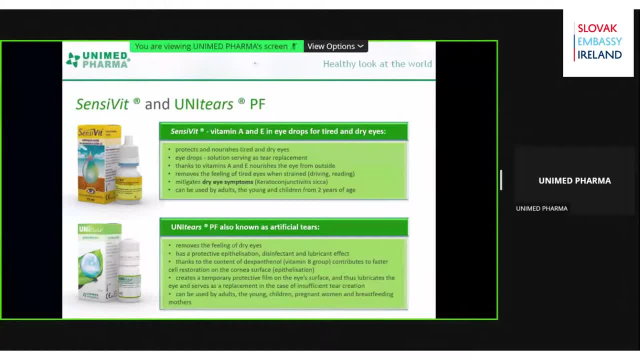 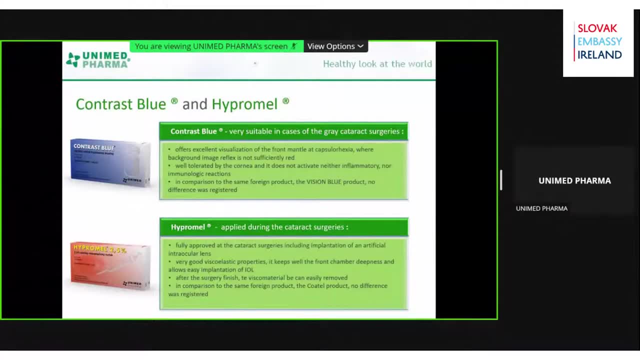 Expantanil E-Promolose, which is a very good option for patients who have first signs of dry eyes. As I mentioned, for eye surgeries we have also products that are used for younger surgeries. It means I mean Ocular Contrast Blue. 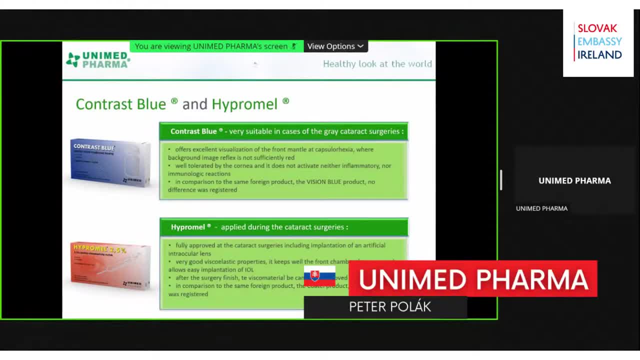 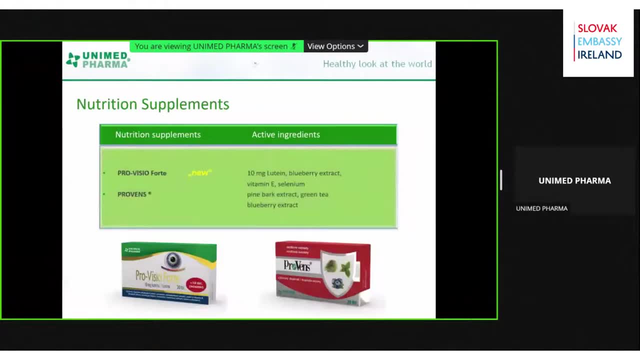 And for eye operations. it's important also to have medical devices like Hypromel, which is of high quality. From Nutrition Supplements. we offer two products: one with lutein for customers who work a lot with a computer, for instance. 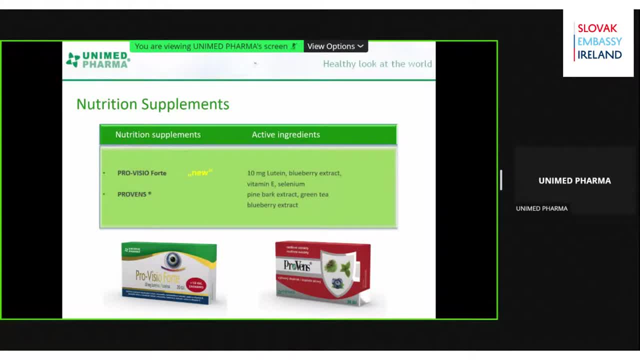 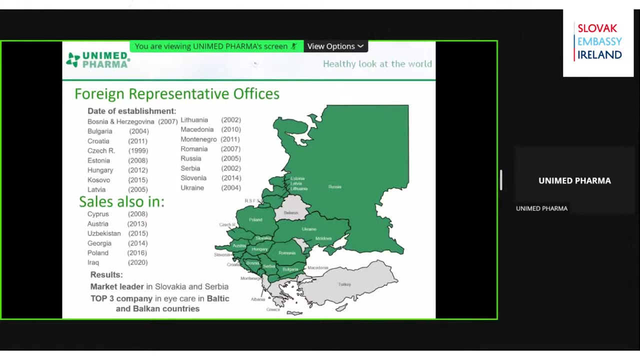 and Provence with the extract from pine bark. Those customers are usually diabetes customers and this product helps them with the nutrition for their eyes. Okay, I'll give you an overview of where we are present. We are mainly in European countries with our representative offices, and also on Asian markets like Uzbekistan, Georgia, or in Asia- Iraq. 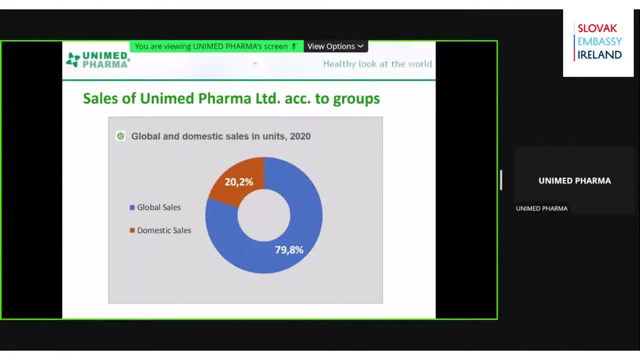 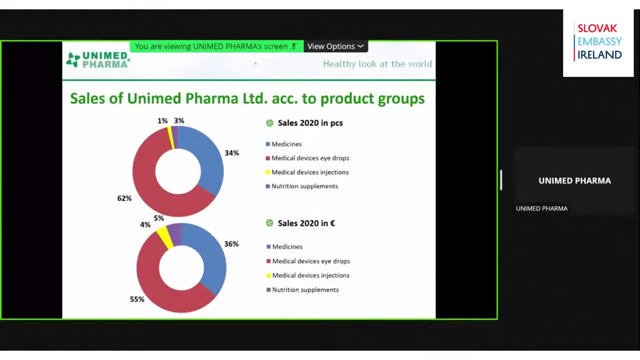 As I mentioned, we are an export-oriented company and you can see that 80% from our sales is export-oriented. So, to give you an overview, how is the share between medicinal products and free products? So it's around 34% to 62%. 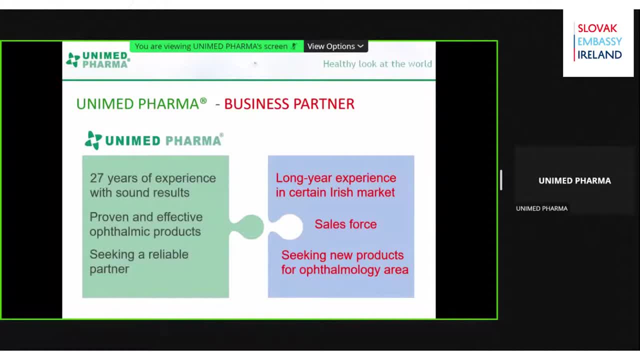 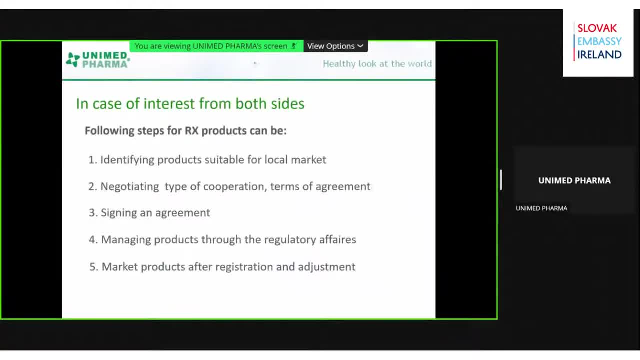 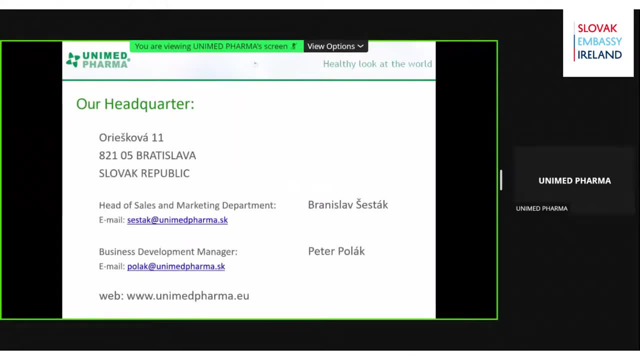 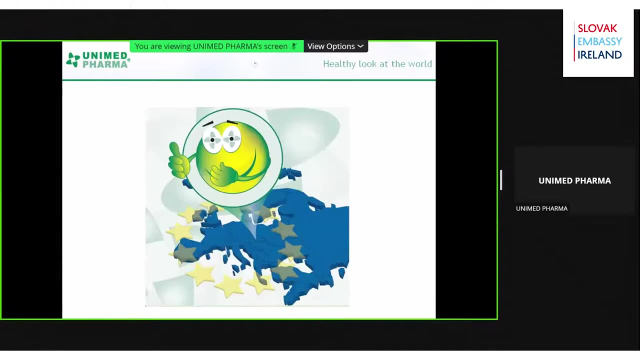 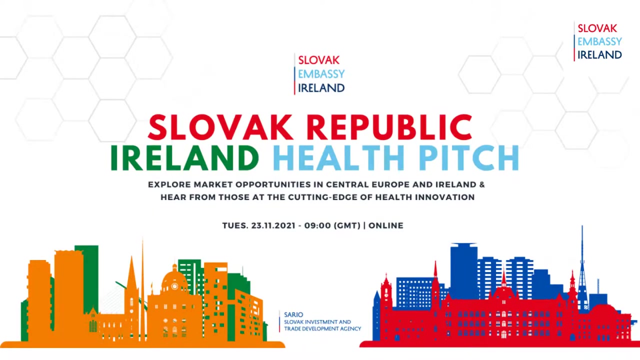 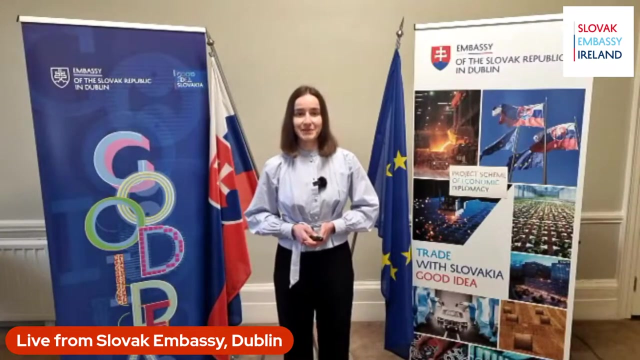 Thank you, Thank you, Thank you. So our 13 presenters is Mr Kieran J McBrien from the Irish company Novareus. Novareus is a kill technology and has been developed here in Ireland by the Novareus team of. 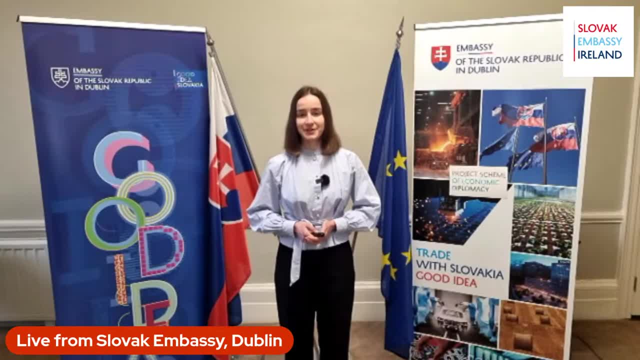 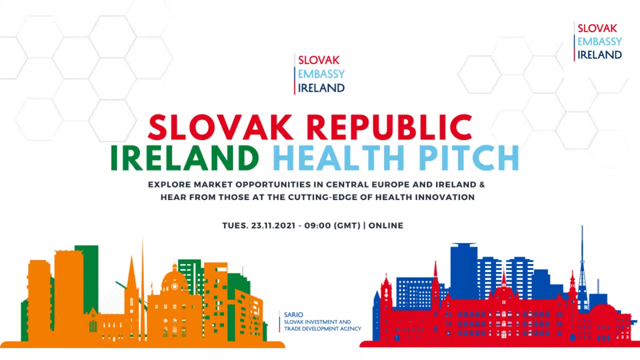 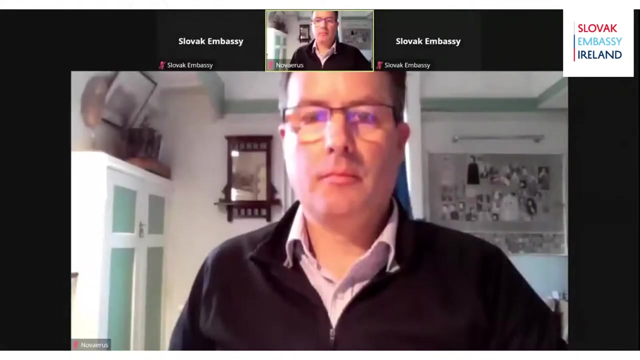 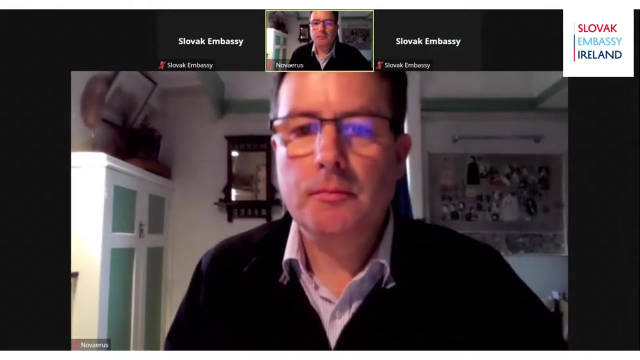 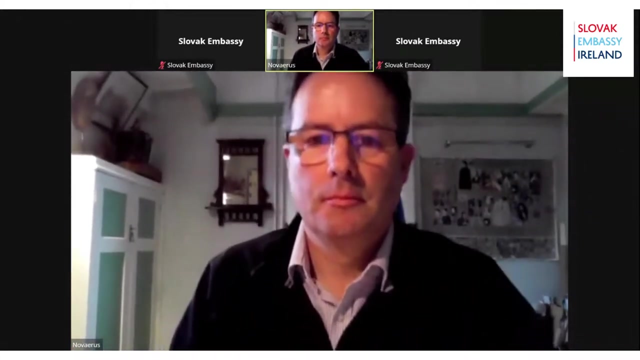 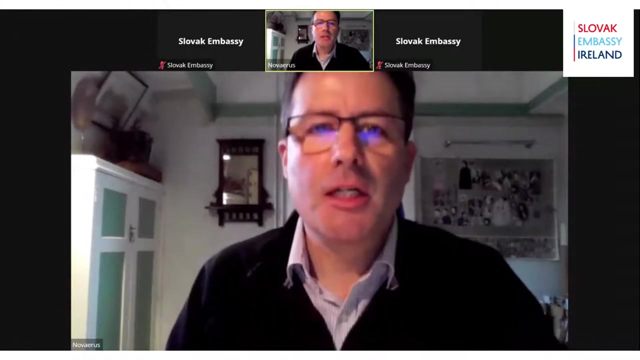 scientists and engineers. It utilizes a nanostrike technology, which is an atmospheric plasma discharge. the same type of discharge found in lightning strikes to deactivate harmful microorganisms. you, Your Excellency, Secretary of State, Minister of State and delegates My name. 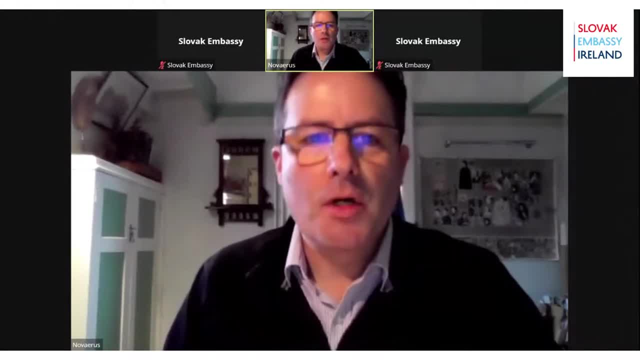 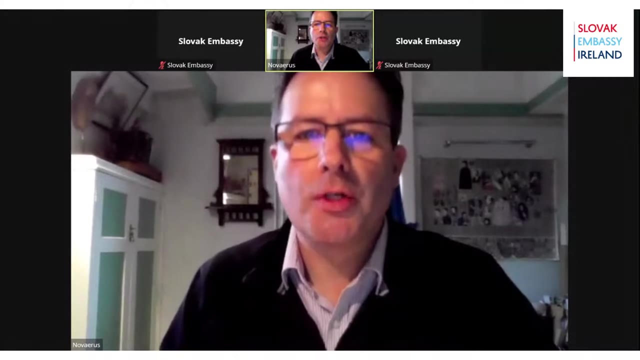 is Simon Bockett, Director of Business Development. Novareus is part of Wellair, a leading provider of infection control solutions headquartered in Dublin, Ireland, and Stamford, USA. Our technology is used worldwide in health care, education, commercial and industrial settings to ensure that airborne 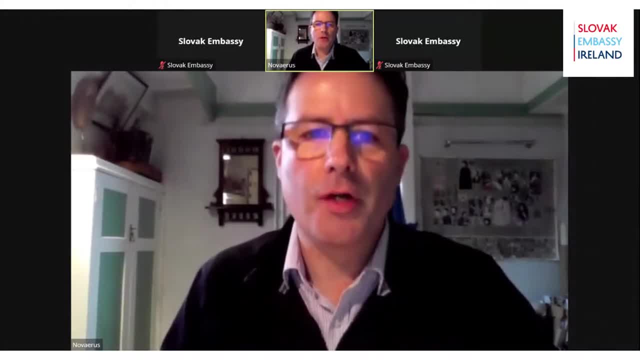 microorganisms are deactivated to no longer pose a threat to human health. Our Today there are over 50,000 Novaris units operating in 60 plus countries, including in European markets. The group operates through its core business brands Novaris, Plasma Air and NuvaWave. 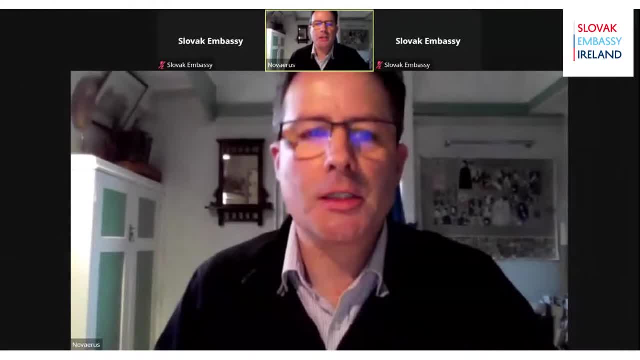 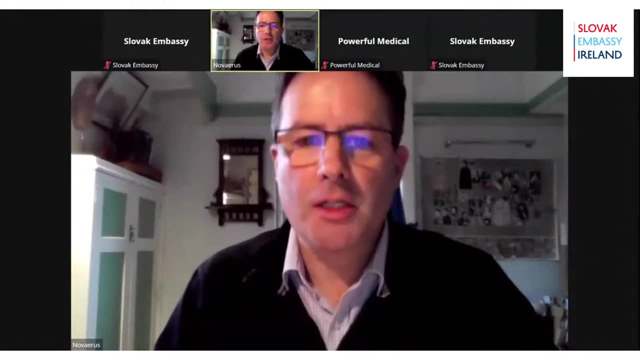 For over a decade, Novaris devices have provided us a medical grade solution that addresses a global problem, namely unhealthy indoor air. Indoor air is the culprit for many virus-based illnesses, bacterial infections, asthma, allergies and a host of other long-term health issues. 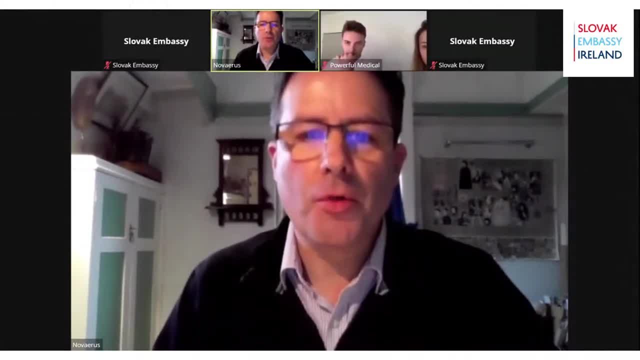 Led by a dedicated team of scientists, we took a fundamentally different approach to air disinfection, which led to the transformational discovery of NanoStrike, the unique patented technology at the core of all Novaris portable air disinfection devices. This nanotechnology inactivates all airborne oxygen. 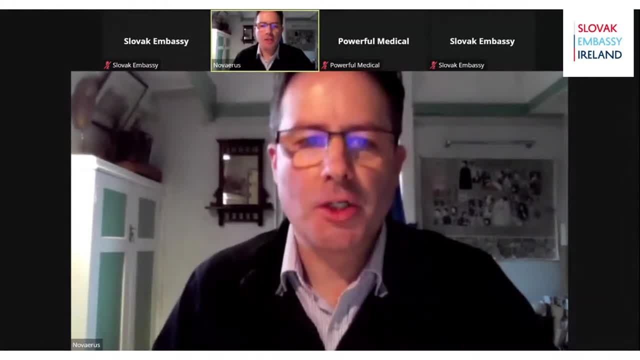 Microorganisms on contact, providing the first line of protection against viruses and bacteria. The technology was invented in 2006 and patented in 2014.. The COVID-19 pandemic has shown us how important air quality is for our health. We believe the EU should make this a priority as we emerge from the pandemic. 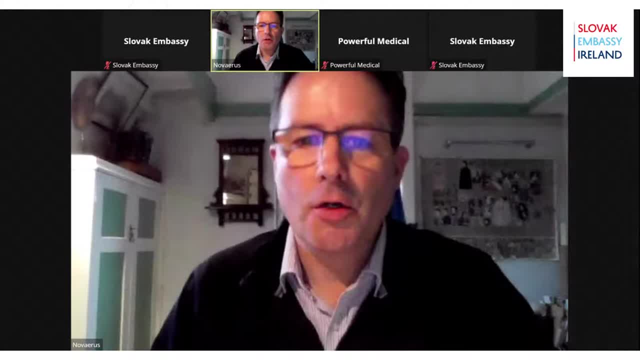 However, some of the important things we know about the COVID-19 pandemic are the following: First, we need to understand the role of airborne transmission With the need for a sustainable air conditioning. the good and bad things about airborne transmission is that a better understanding of airborne transmission is the key to breaking the chain. 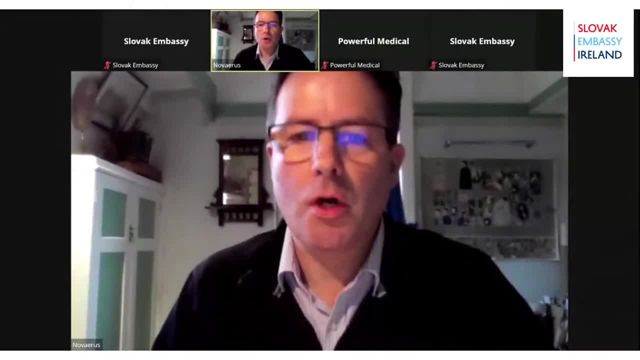 others look to install CO2 monitors or complicated new ventilation systems. However, these measures are applied in a somewhat ad hoc, uneven and inconsistent manner which fails to take account of the actual problem. We wouldn't clean ourselves with dirty water, So why aren't we looking at the air that we breathe? 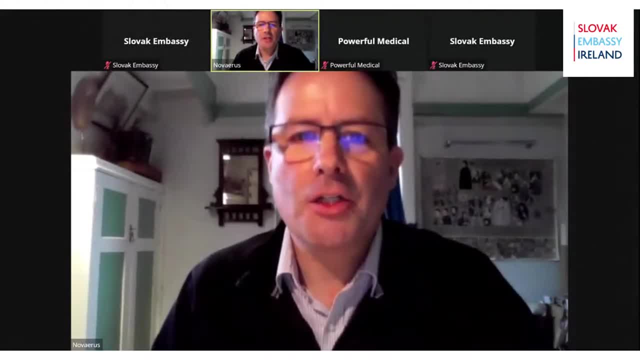 The various air purifiers are an innovative, energy efficient and cost effective solution to reduce the risk of COVID-19 and other viruses spreading indoors. Diseases like COVID-19 have consequences for our health care systems and generate delays in accessing treatment and care Outside of health care. there have been increasing calls for schools to add protections for children against COVID-19,. 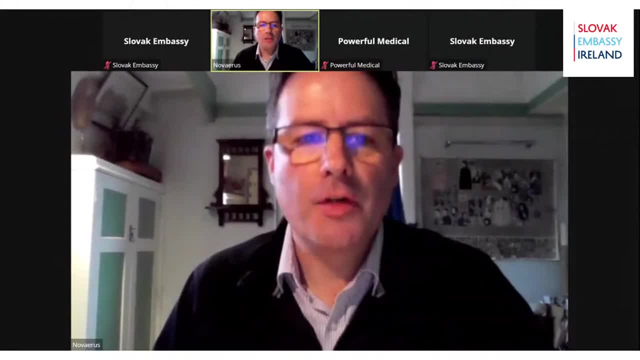 particularly since many of them cannot be vaccinated. Air disinfection is a cost effective way of adding additional protection. How to curb airborne viruses and other pathogens should be considered by European policymakers when looking at the Air Quality Directives, Horizon Europe and the Strategic Framework for Health and Safety, Work 21 to 27.. 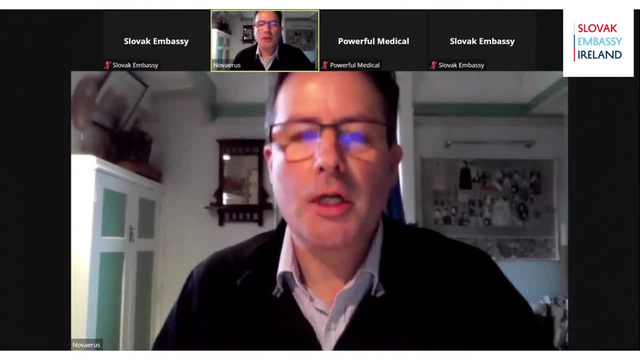 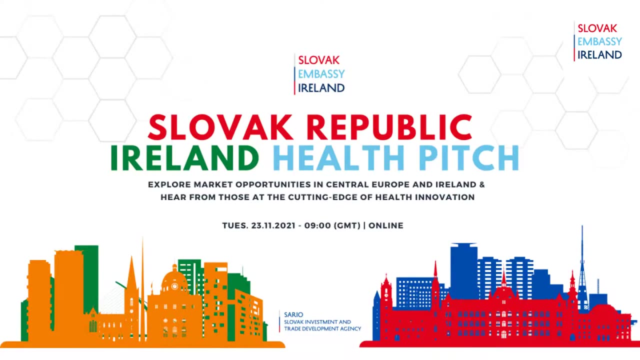 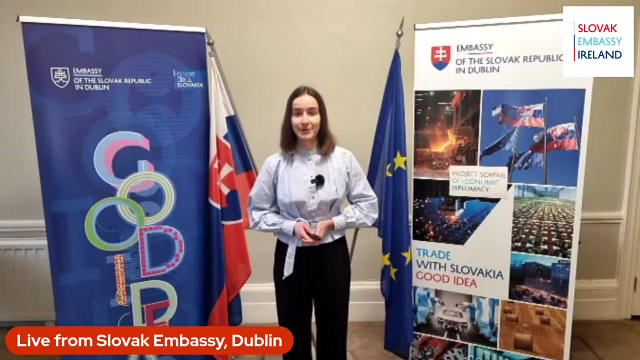 So, in summary, nanostrike technology utilises only physical means to inactivate viruses, bacteria and fungi. We emit only purified, treated air. Thank you, Thank you very much. The next presenter is Mr Michal Haveriš, from the Slovak company Powerful Medical. 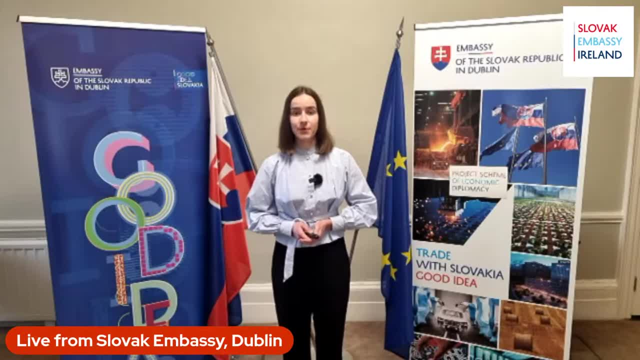 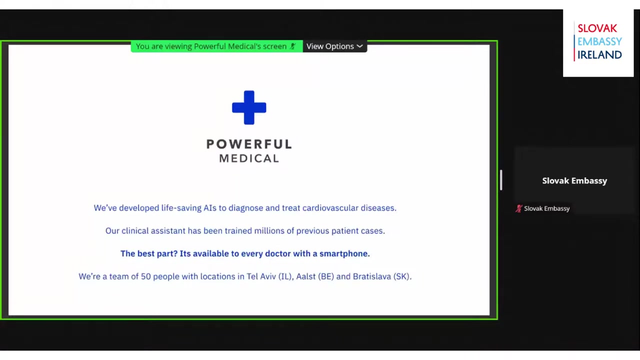 Powerful Medical is a deep tech company tackling the most challenging opportunities of modern medicine and creating a superior patient experience. The company empowers doctors with expertise from millions of previous cases to give patients the most reliable diagnosis and treatment. Hi, my name is Michal Haveriš. 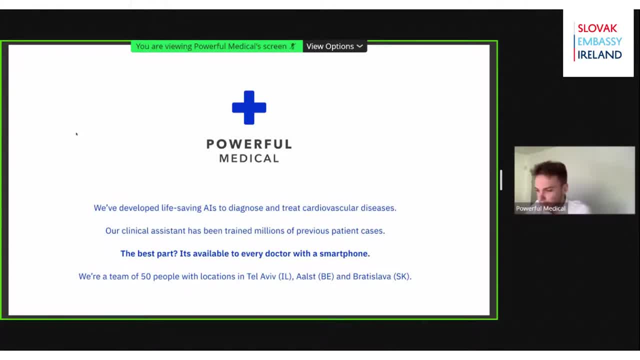 Thank you very much for the floor. I represent Powerful Medical As a company. our mission is to tackle challenges of modern medicine through the application of innovative digital technologies, including AI and big data. We have a big focus on clinical research. However, the other and very equally important part of our work is the integration of these technologies into products that are ready for the real clinical world. 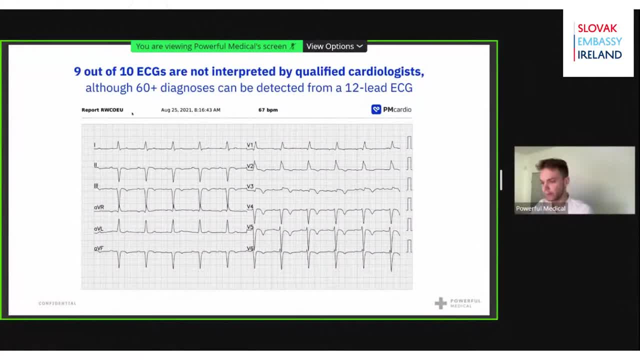 What you see here on the slide is our first on-demand product. Our first undertaking is in the field of cardiovascular diseases, which are the leading cause of death worldwide. What you can see here on the slide is a 12-bit electrocardiogram, or the ECG, or the EKG, from which over 60 cardiac diagnoses can be detected. 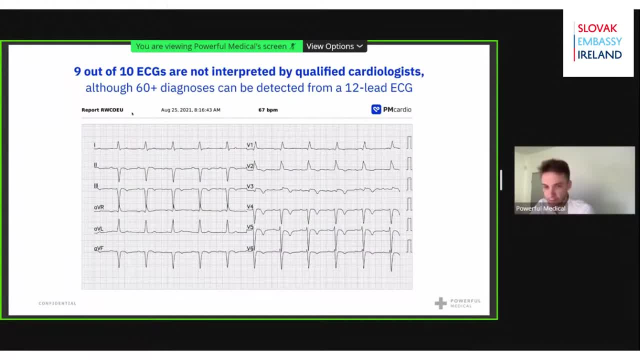 However, a big issue is that 9 out of 10 ECGs are not interpreted by qualified cardiologists, leading to the underdiagnosis of cardiac patients or, on the other hand, the overloading of specialist facilities, preventing the necessary patients from accessing these technologies. 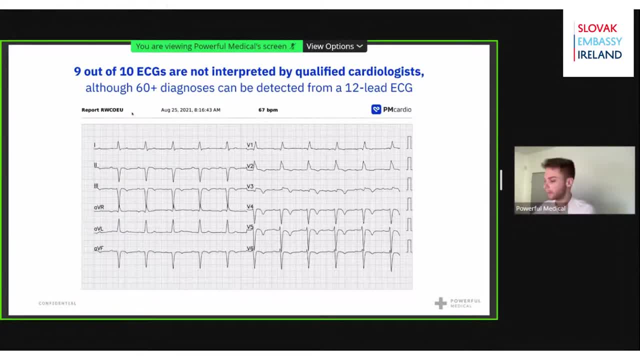 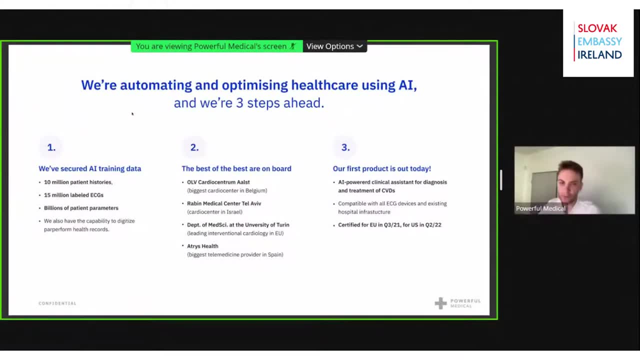 To address this. we also need to make sure that patients are treated, and treated properly, in order to ensure that patients are getting the right care and access in a timely manner. So what we are doing as a technology company to tackle this problem. 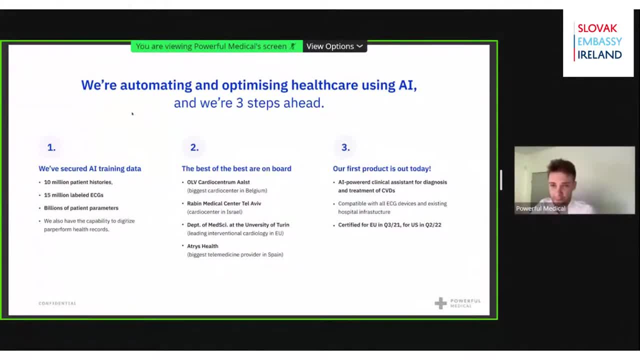 First of all, we have secured a proprietary database of over 10 million patient histories, 15 million labeled ECGs and billions of additional patient parameters to train our artificial intelligence. Our AI is clinically validated by some of the leading partners in Europe and the rest of the world, including the all-week cardio-technology network. 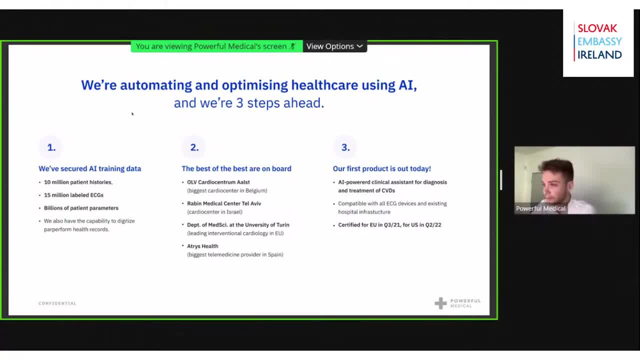 We also have a huge capacity to train: our artificial intelligence Centrum in Aalst Belgium, Rabin Medical Center in Tel Aviv, the University of Turin and Atris Health in Spain. The results of our clinical efforts is our first product, which I'm happy to. 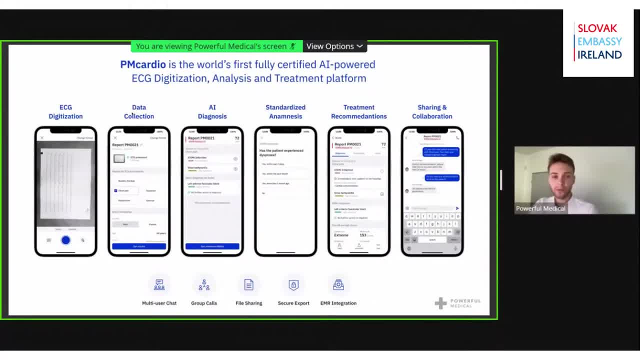 say, is available today. What you see here is PM Cardio, the world's first fully certified AI-powered platform for ECG digitization, analysis and treatment of cardiovascular diseases. It is a certified class 2B medical device under the new EU MDR regulation. How it works is a healthcare. 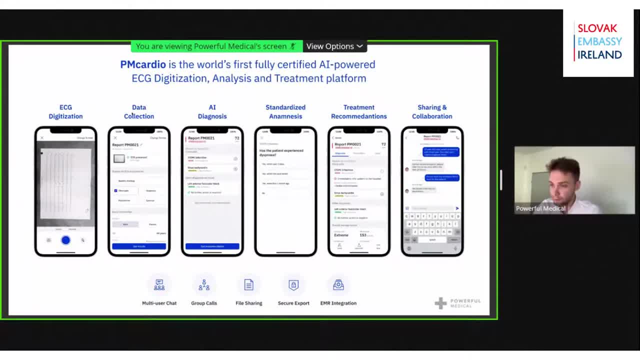 worker is able to digitize any ECG, regardless of its format. These digital signals are interpreted by our AI, together with additional patient parameters that are derived from clinical practice guidelines published by the European Society of Cardiology. The processing of all these parameters together results in a complex report on every patient, including the identified. 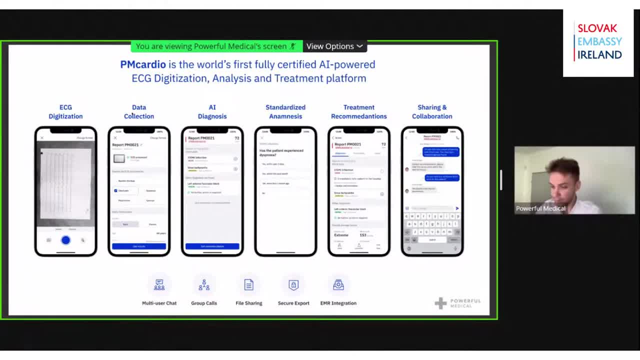 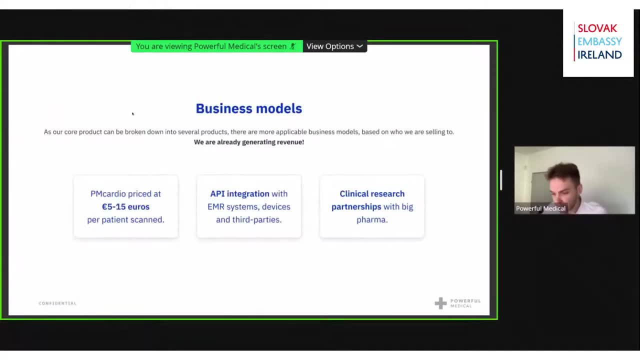 diagnosis, trial and trial. The process of all these parameters together results in a complex triage class and recommendations for next steps In the final stage. these reports can also be seamlessly shared between physicians in each other's networks, enabling instant collaboration on a specific patient. In terms of business models, currently we have three main lines of: 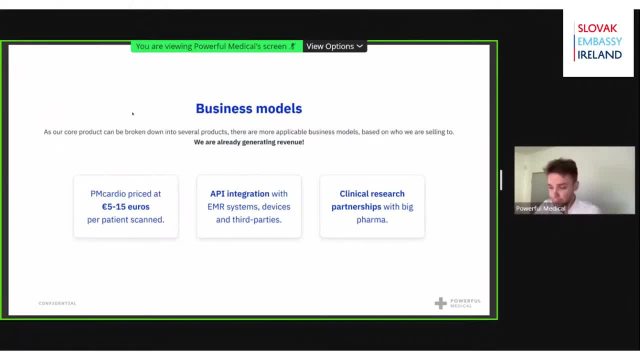 business. Our existing clients include GP clinics, emergency service providers, hospitals, as well as insurance companies, whom we charge 5 to 15 euros, depending on the scenario, per patient scan. We are also able to deploy our technology into existing systems via API. 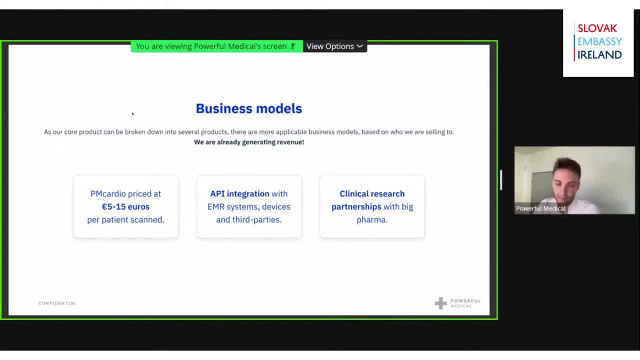 integration, for example, together with telemedicine platforms. Finally, we have several partnerships running with big pharma companies, whom we support in, first of all, running clinical trials, as well as bringing- crucially- their medicines to the right patients using our proprietary software. 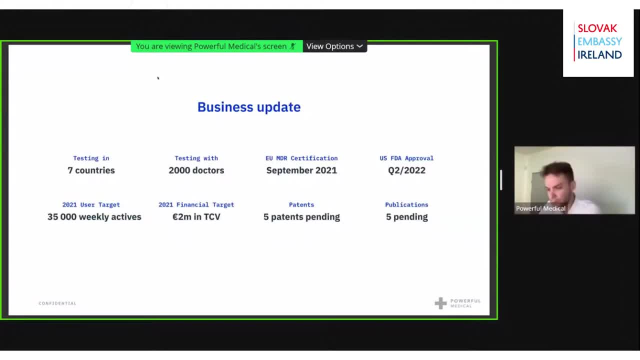 Oh sorry, Maybe a few numbers To close the presentation off with. we currently operate in seven countries. Today, it's over 5,000 doctors whom we cooperate with. actually, As mentioned, we are MDR-certified and we 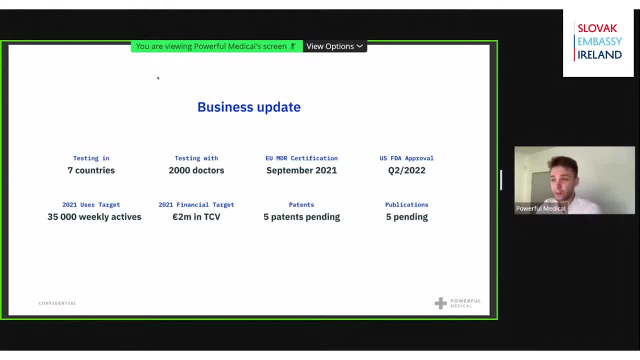 are awaiting FDA approval in mid-2022.. Our targets for 2021 are 35,000 weekly active users, a total contract value of 2 million euros, which we are well on the way of acquiring, and our Our research is covered by five patents that are pending and five pending scientific publications. 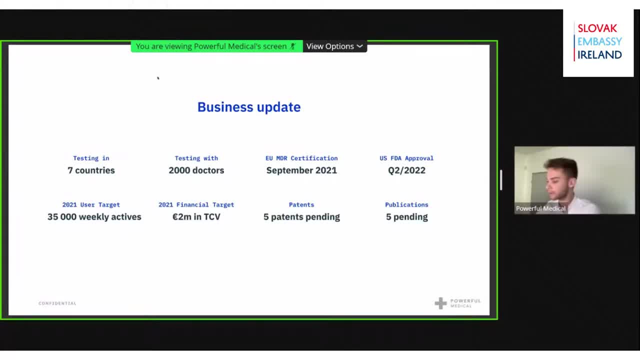 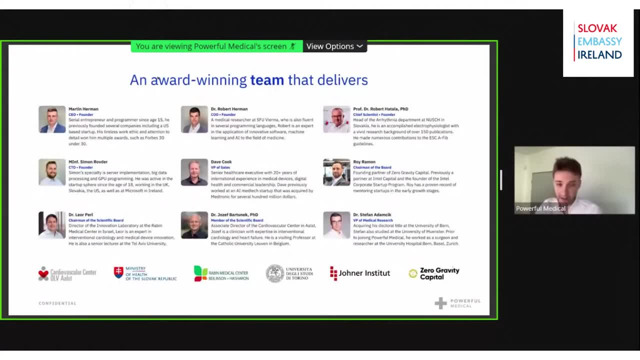 experience that actively contributes to both the day-to-day healthcare work and to establishing and publishing the aforementioned clinical practice guidelines. And we are also supporting of the world's leading investors, for example Roy Ramon, who previously worked at Intel Capital, In this. 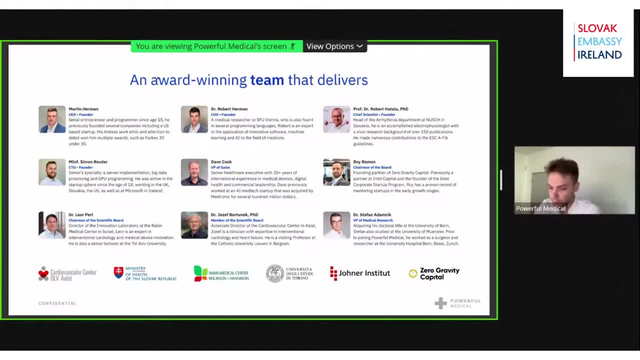 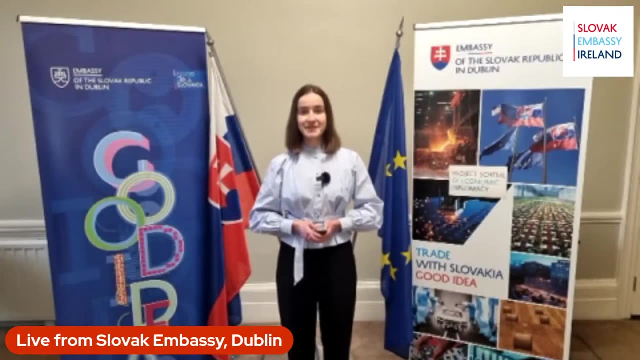 In this context, we are happy to expand our partnership network with relevant institutions in Ireland and we'll be very happy to work with you, So please get in touch. Thank you very much. The 15th presenter is Mrs Veronika Hudzikova from the Slovak company FaceRehab. FaceRehab. 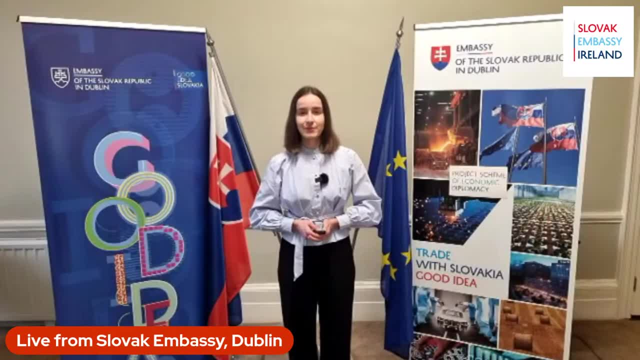 created a mobile application which will allow the users to download their finance software, use the software to process a message that they receive every day from the patient and the University of Slovakia, and implement a mobile application that will help them access the data and access websites and theathacom. So we're looking forward to seeing you. 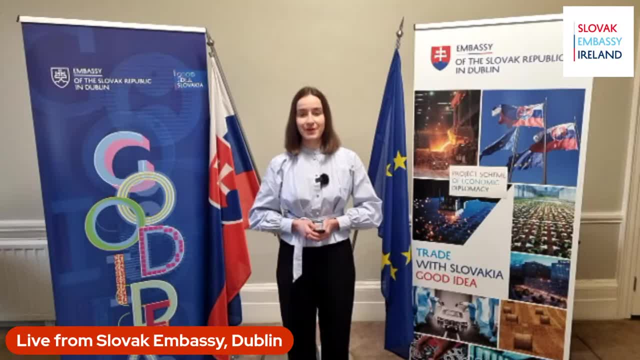 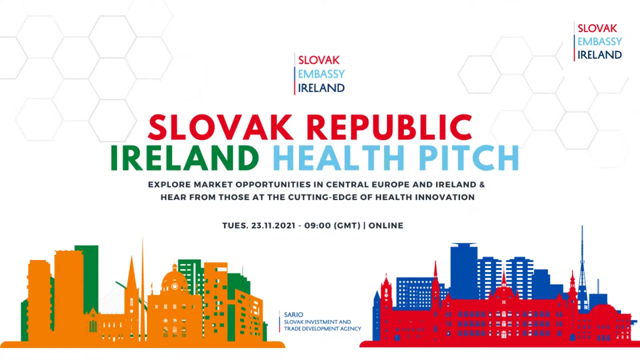 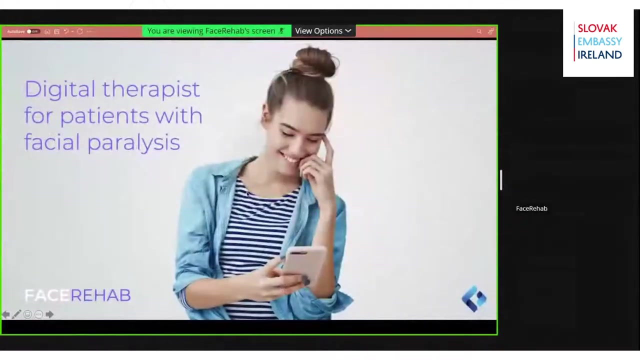 on the show, measure for patient level of facial paralysis and perform muscle movement activity using a depth camera in a smartphone. After initial face diagnosis, the patient can practice recommended exercises or play mini games using a face movement controller in the application. Hi, there, can you hear me? Okay, great, So let me start. Hi, I'm Veronica and let me introduce you. 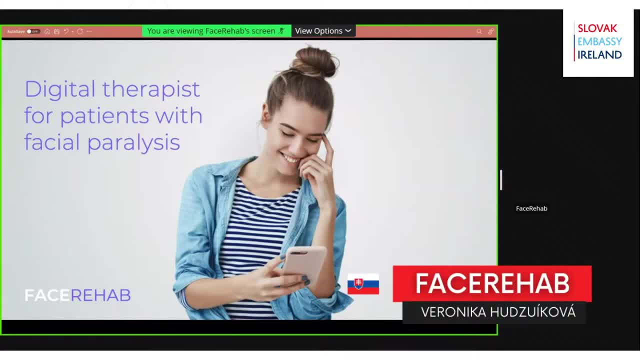 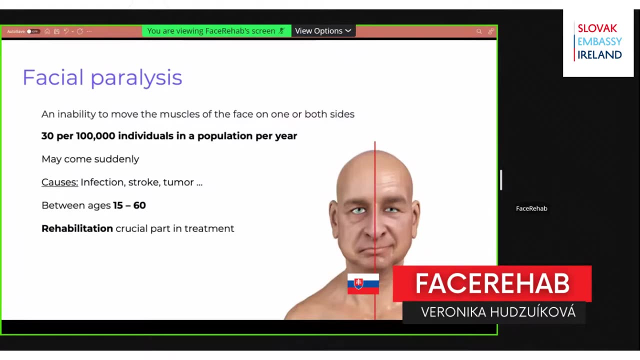 to Facerehab, the digital therapist for patients with facial paralysis. They use mobile application and front camera to track 3D face model of a patient. Facial paralysis is an ability to move the face With the muscles of the face on the one or both sides. It can happen to every one of us. It can. 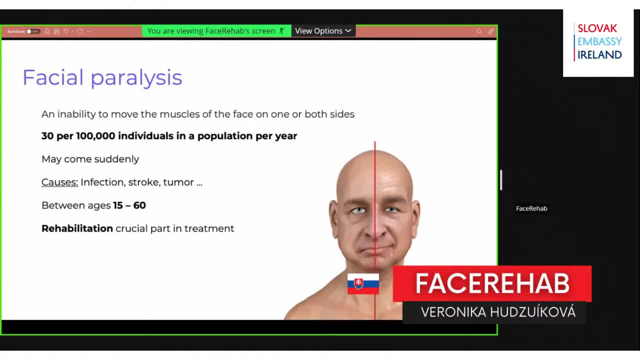 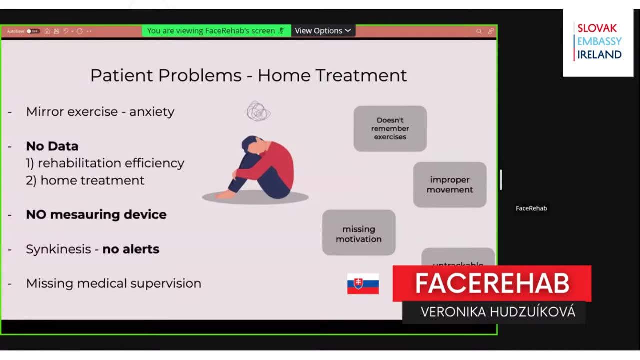 be caused by infection, stroke, tumor, even by the wind, And mostly it's happening between the ages 15 and 60. Rehabilitation is a crucial part in this treatment. This patient who are taking this rehabilitation has many problems And one of them is a home treatment. You should continue these. 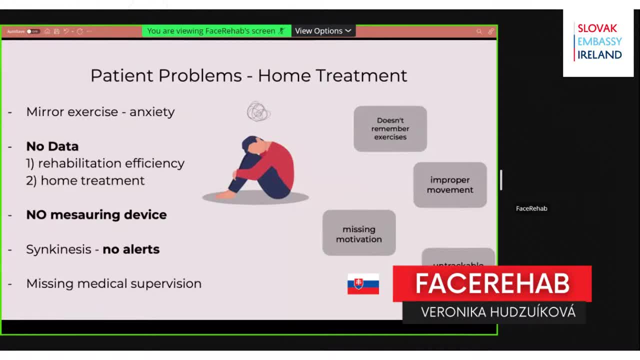 exercises back home, But they are looking at themselves in front of the mirror and this brings them depression or anxiety. We have no data about the home treatment process, If the rehabilitation is efficiency, because we don't have any measuring device that could be available. 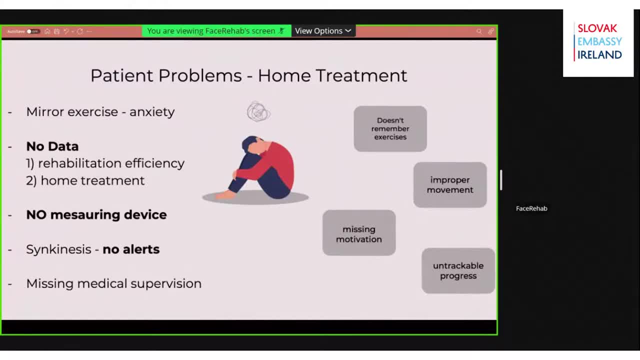 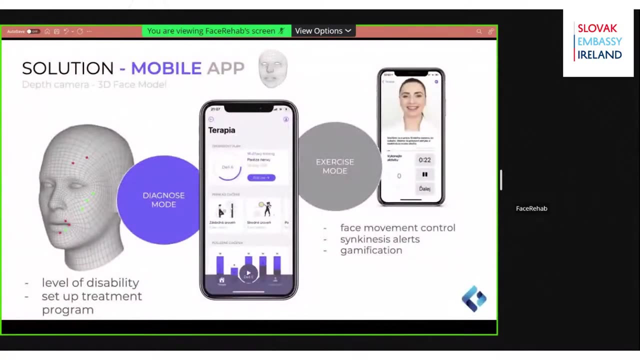 for a patient. If the patient is exercising and remembers some of the exercises, it happens that they are doing these exercises wrongly And this means that synkinesis can occurs and there is no alerts. We can see that there is missing medical supervision And that's why we built medical mobile. 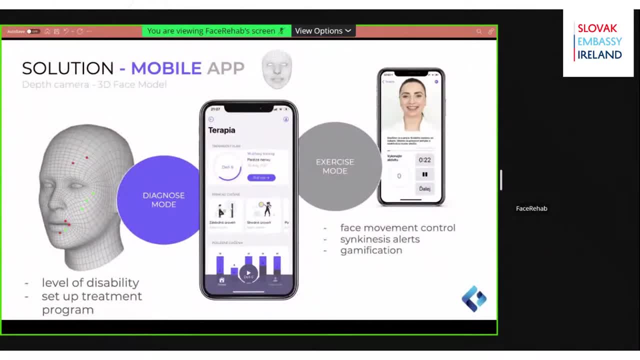 application. It's a therapist in the pocket of a patient. We are using this front camera and providing two modes. The first one is a diagnose mode. Based on the diagnose, we are specifying the level of disability of the patient And based on that we are set up in the treatment program. We also have this exercise mode for a 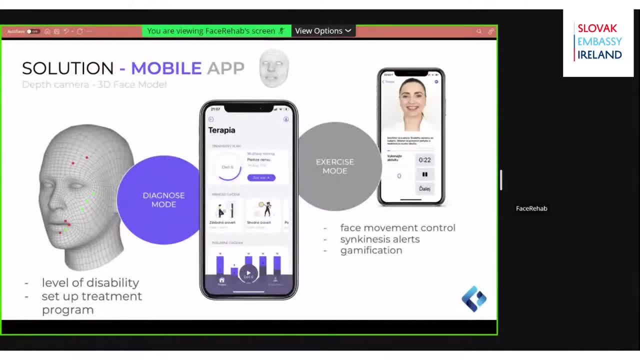 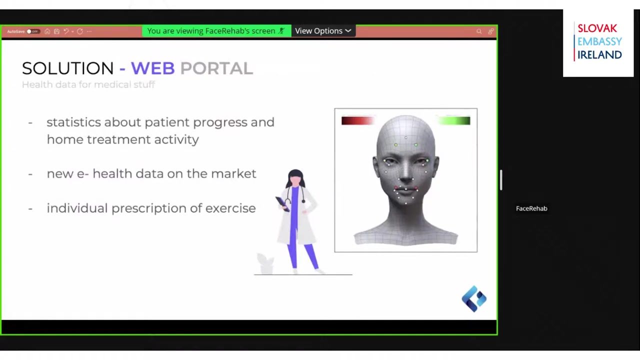 patient. Now can patient practice all these exercises interactively involving these muscles. So exercise cannot be boring but also fun. Also having gamification so patient can play games while controlling them. with this for script facial exercises. Not the only application we have. We have a web portal for medical staff and physiotherapists, neurologists. 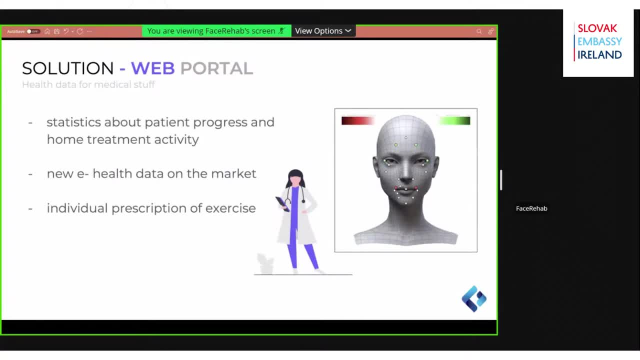 to Iced. All these data are completely new on the market because we didn't have this, So the used center device could measure that the data we have right now are first on the market and be used for other research. patient haircut Number three: an escalator, And this is super simple. A neutralized Rangerswill perform previous. 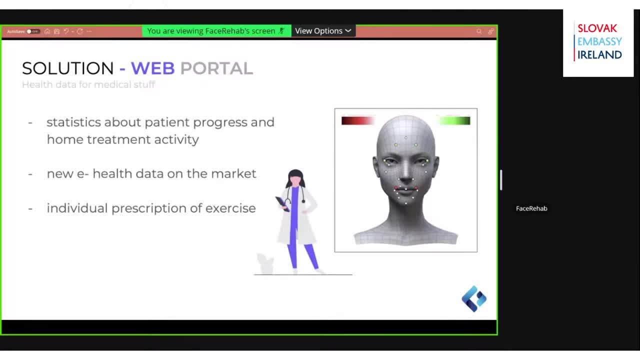 pressure purposes or may change be excessively able to come to one end of the model as well as adjust foot. But also we have put these. we have placed bars on check to prevent adjustedBY. So we're using it for individual prescription of exercise for each patient separately. 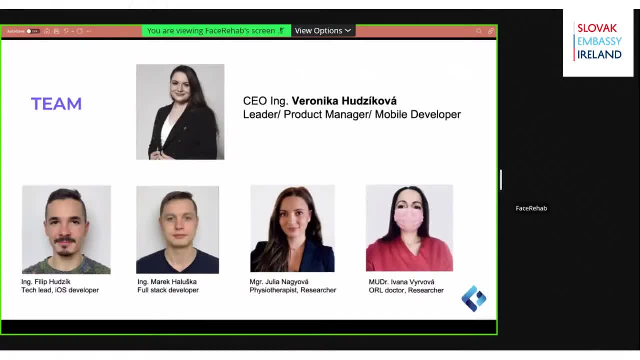 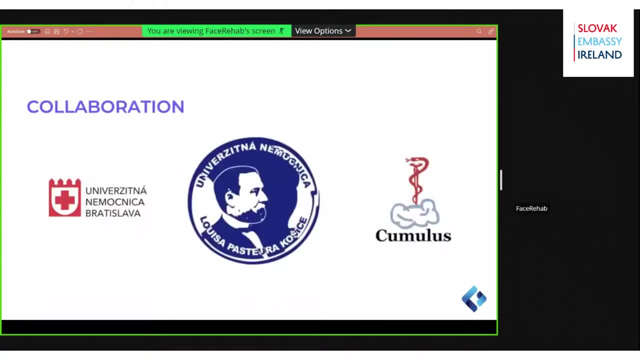 Our team is combining the technical knowledge and medical knowledge on the board. We have a tech guys and we also have a physiotherapist and doctors on the board. We are collaborating with two hospitals- university hospitals in Slovakia and one private hospital- And right now we are testing this solution and making first clinical trials. 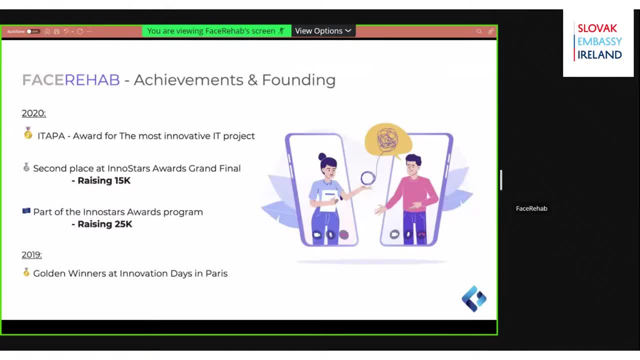 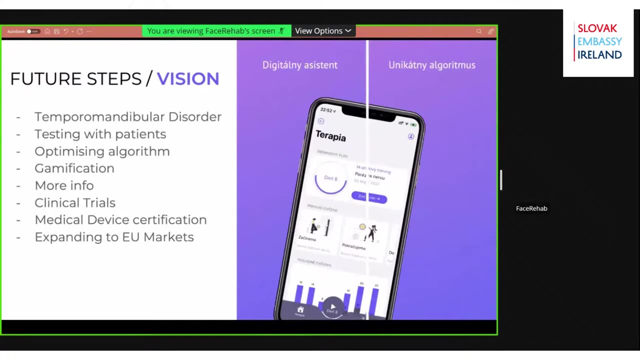 Our achievements are: we were in the part of InnoStars EID health awards. We won their second place, we raised some money And also we were an innovation day in Paris where we were golden winners. So our focus is to implement other solutions, other features into this application. 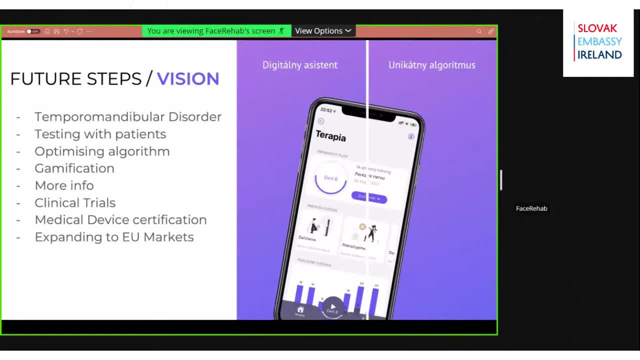 For example, the temporomandibular disorder, to make other features on the phase rehabilitation process And use this application. We were trying to optimize this algorithm to make it more AI and knowing the patient and, based on that, specify the program for them. 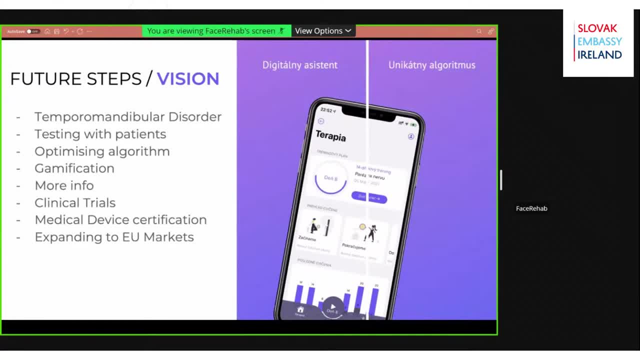 We're applying more gamification, more information for the patients, and we're working on a clinical trials and medical device certification, and we would like to then expand to other markets. So what do we say to our patients that we can bring your smile back? 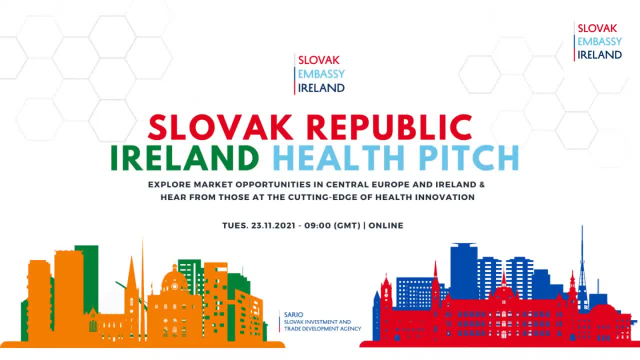 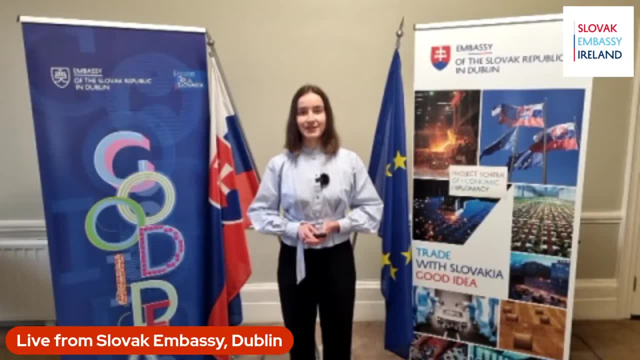 Thank you so much. So our next presenter is Mr Fergal Dagnon from Irish company Paxsana. The company offers a suite of products to help prolong independent living for older people or already offers its services in Ireland and UK. Paxsana uses simple wearable technology to improve care for customers while also facilitating 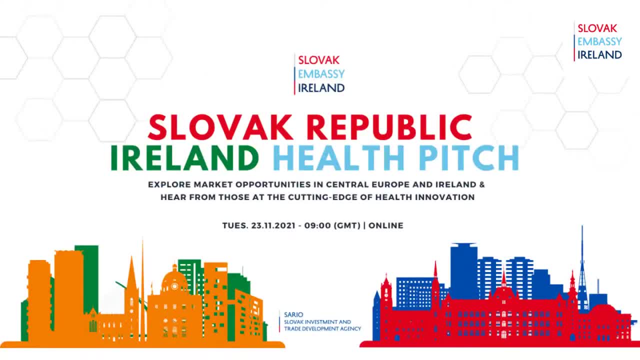 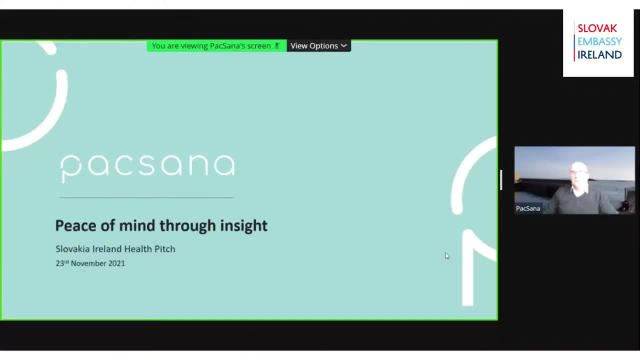 independent living. Thank you very much. Just to double check, Can you see my PowerPoint presentation? I hope so. Okay, Good morning folks. Thank you very much for your time this morning and thank you to the Slovak Embassy in Ireland for arranging this session. 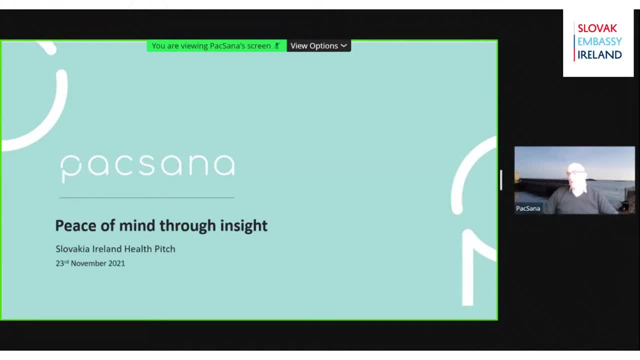 My name is Fergal Dagnon. I'm the CEO of Paxsana, and at Paxsana we use technology to improve how care is delivered in the community. Sorry, Let me skip through this. Care is a human business. It's a business. 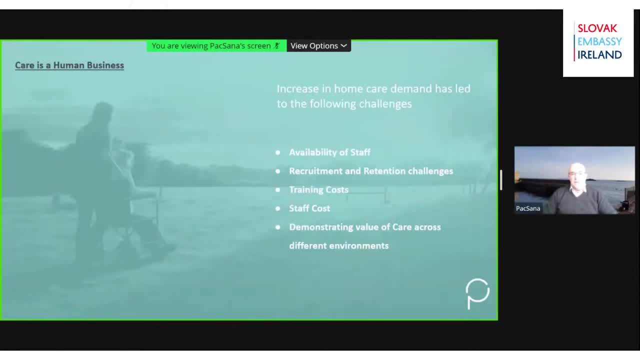 It's a business. We've seen over the last number of years, particularly after COVID, a massive spike in the needs of providing care in the home. Outcomes are dramatically improved for people as they live in their own home, But what we need is more caregivers. 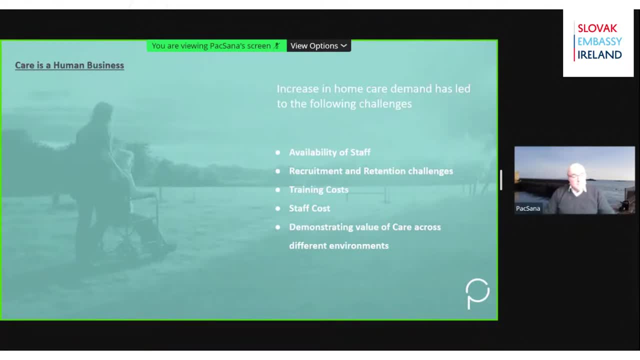 There's a dramatic shortage in caregivers, So what we need- the problem that Paxsana want to solve- is that of enhancing how we use technology to provide better care With the absence of caregivers. Really, Technology is something we can use much better and we need to focus on how we can do that. 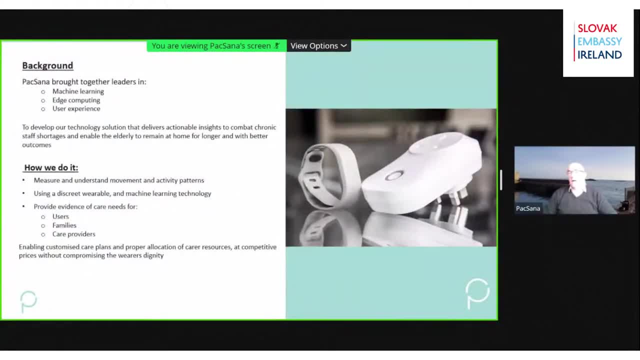 The background for Paxsana is: we set up over three years ago and we brought together leaders in machine learning, edge computer, edge computing and user experience to understand how people engage with technology and how they use it, And what we wanted to do was bring the user to the center of the conversation. 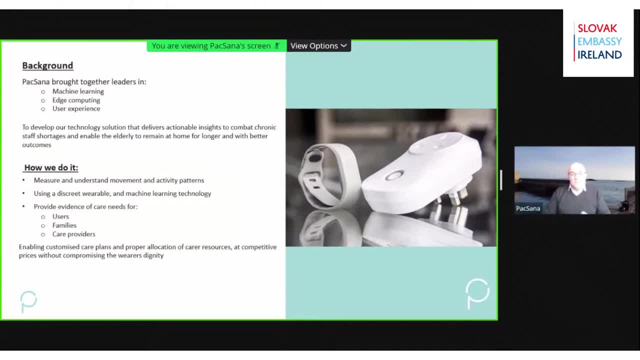 In doing so, we built a solution, Yeah, That is focused on the outcomes that are going to enhance the life of the client, which is at the center of it, And we do that by supporting caregiving organizations with technology to interpret data that can. 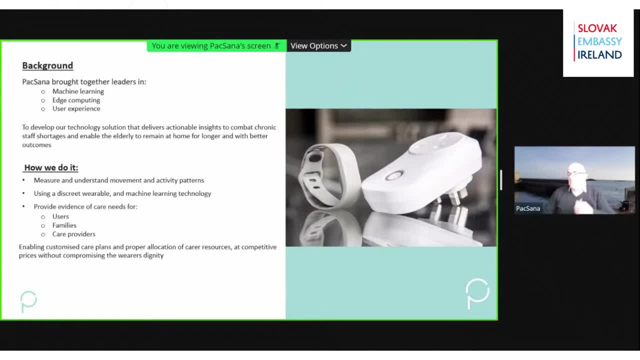 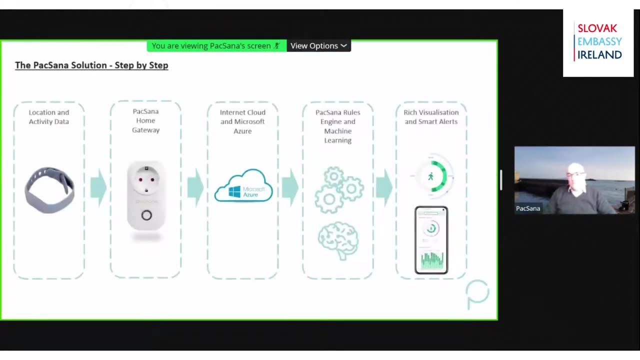 help and govern how care plans are delivered. We measure and understand movement activity in the home, and we do so using our wearable technology, and we share that data with families and their care providers. Our solution is a very simple cloud-based solution. We have a wearable that holds a sensor. 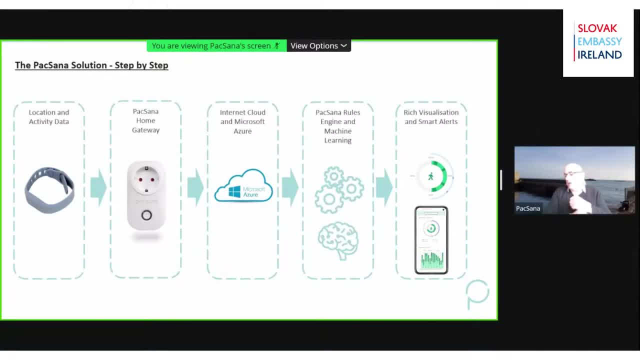 It's very simple and light wearable. It's very high compliance rates with our clients- over 90% in terms of adherence to wearing the wearable 24-7.. We connect that to a gateway And we're a Microsoft Azure partner where we model the wearable 24-7.. 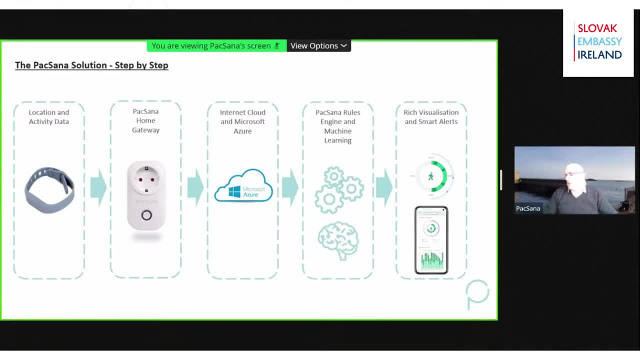 And we connect that to a gateway And we're a Microsoft Azure partner where we model the wearable 24-7. And we're a Microsoft Azure partner where we model the wearable 24-7. And we balance that data with bendable and visualize data that we present to our clients. 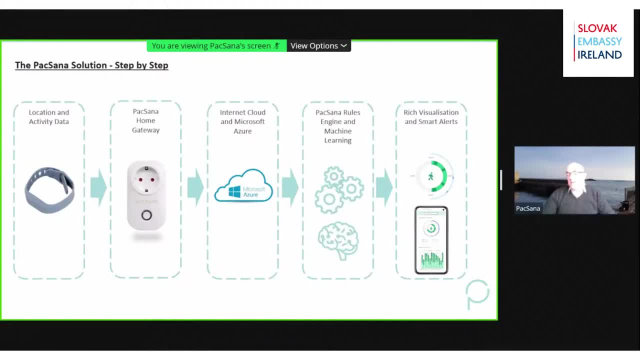 One of the reasons we've focus on gateway and wearable solution is to make sure that we remove the platform as far as possible away from the client so we have longer battery lightolo, a six month battery life- dolly life by pushing the technology upstream, if you. 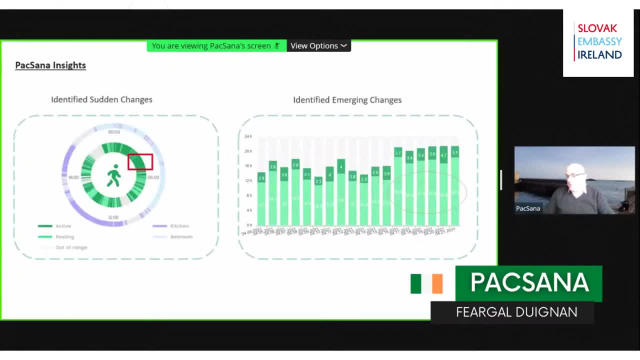 like. This is some of the data sets that we 초ize for our clients As we're getting data stream of data. this, or the granularity and the insights become more meaningful over time. but you can see here on the left-hand side and that's a 24-hour clock. the external circle is 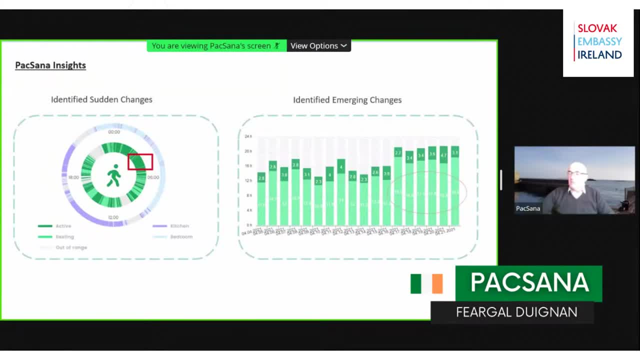 the location of the user. the internal circle represents their activity levels and mobility, and and what we we see here is um is it's sudden changes in that activity and and so that can identify a wandering event, movement in the um, excess of movement or an absence of movement. 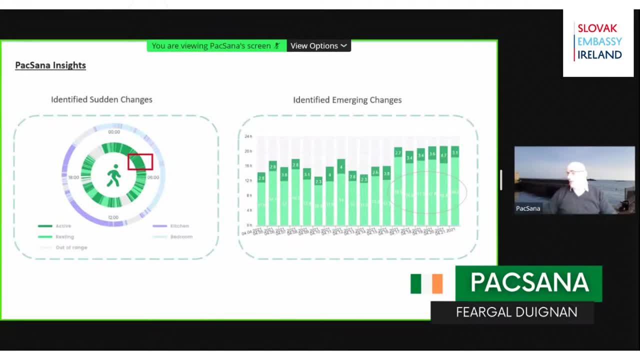 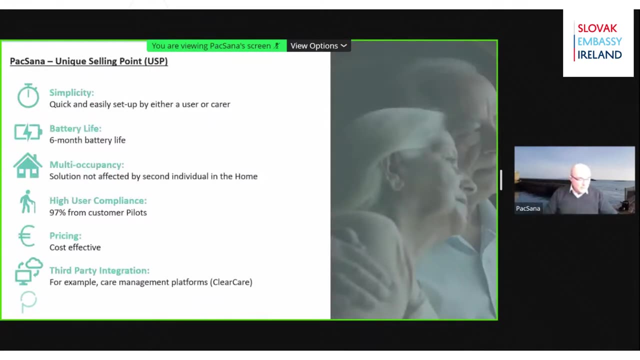 in the home and, and equally on the right-hand side, we can see emerging trends, changes in in specific pattern and changes in blocks of sleep, or indeed absences of sleep and movement around the home at night, and so on, the the reason why we have such a good traction in the market at 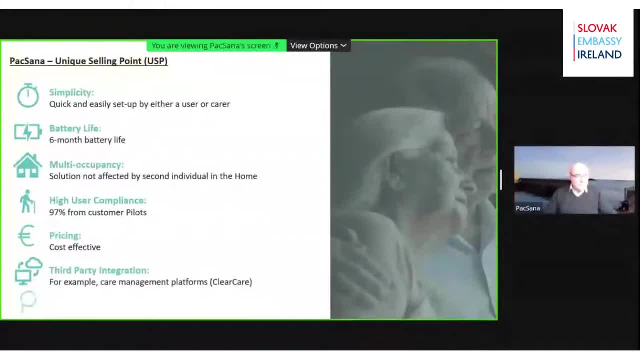 the moment is this simplicity: we have a deployment of a simple wearable and a number of gateways in the home and deployed typically in under four minutes- and the simplicity of the solution itself also allows for a six-month battery life for the wearable that's worn- 24 7. 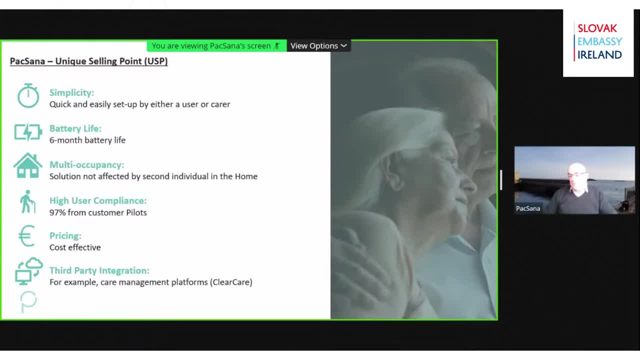 waterproof in and in and out of the home and we support multi-occupancy dwelling many technology solutions in the home and get confused by and by. if there's animals or other adults or children in the home, the compliance rate is really high. for for clients, they love, they love the build up, the 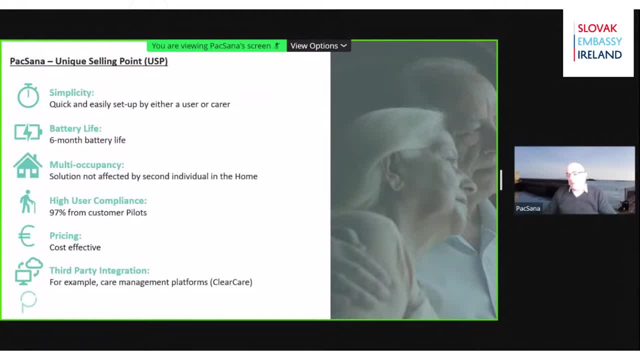 product. they feel very comfortable with it and they it's kind of a set and forget model and we have a very cost-effective approach to the product and we have a very cost-effective approach to the product and we have a very cost-effective approach to the product and we have a very cost-effective 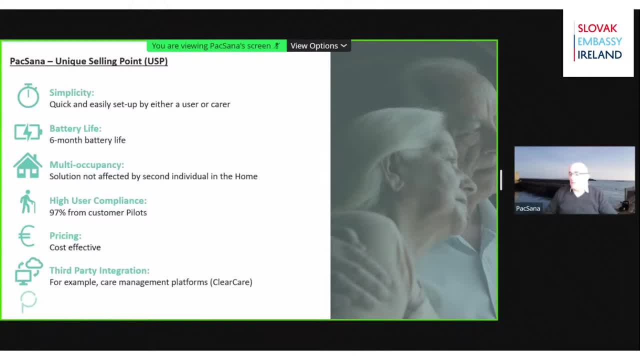 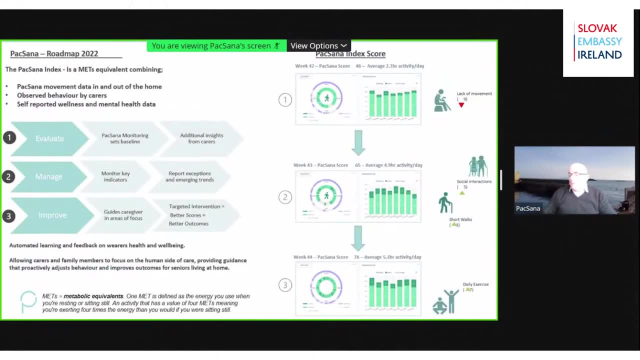 model for this, and it in terms of it's under a dollar a day, in terms of our us customers, and and we're an open platform that integrates and eat readily with others. and for 2022, i want to share this roadmap with you and we- we currently um- are in a position to assess and evaluate how 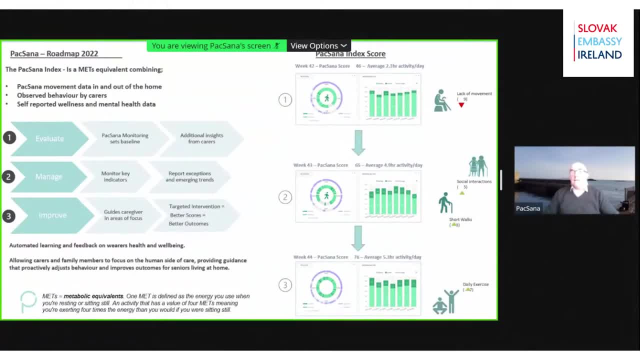 our how our clients are doing and set a baseline for them, and then, through our monitoring and process, we can and we can help manage and, and, and you know, ensure that people are safe and and. but what we are moving to is a process of improvement where we give guidance to caregivers. 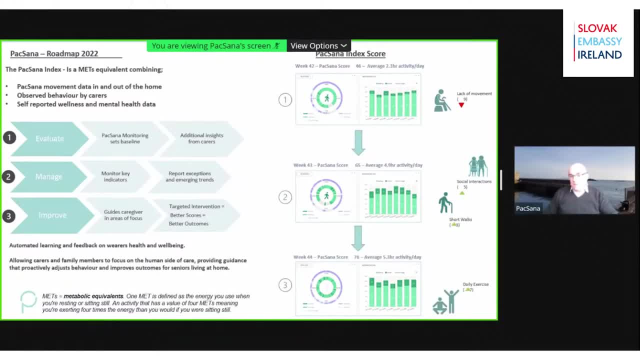 and using the insights that we've gathered, that you know, observational data, paxana data and um, and self-reported data from clients who are able to engage- to build a paxana index that allows us to to guide the care and to move from survive to thrive, which is where we want to see our, our 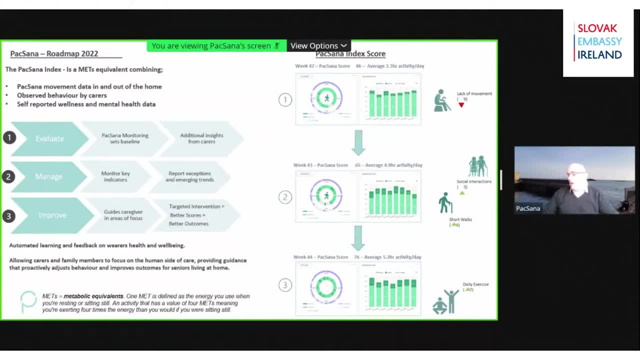 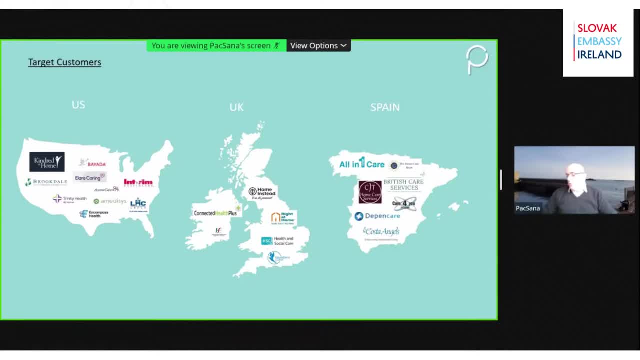 we operate in in the us, the uk, and we're looking at european markets at the moment, and the companies that we work with particularly in the us are private home care companies and a lot of franchises and independents. some of them would be state funded, but in the uk and 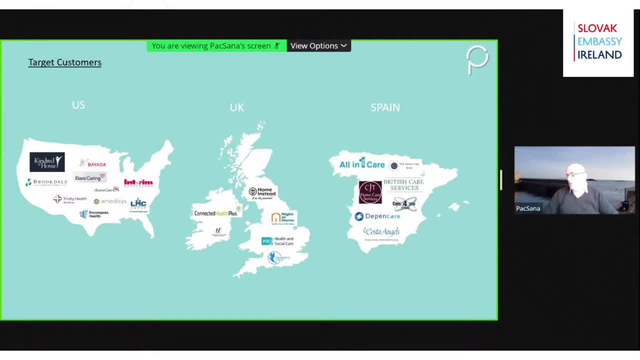 ireland, for instance, we've- uh, we've- worked with connected health in belfast for a number of years and we've done, we've done some projects for home instead in the uk. but we're really kicking on to a kind of a global launch in q1 of next year and and so, with that in mind, we're very interested. 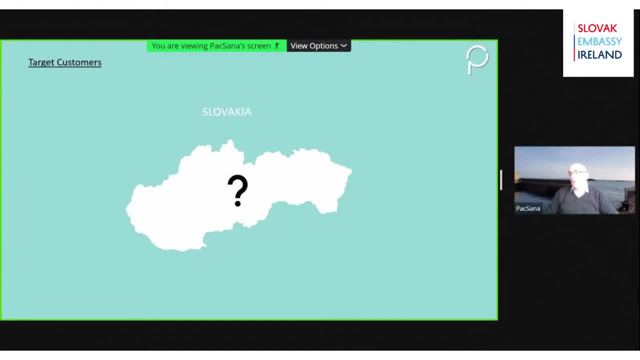 to see it what partnerships and local and relationships we can build and with the slovakian embassy and and partners in the field. so, and again, my name is fardo deignan. thank you very much for your time. really appreciate it. please contact me with any questions, okay, thank you. 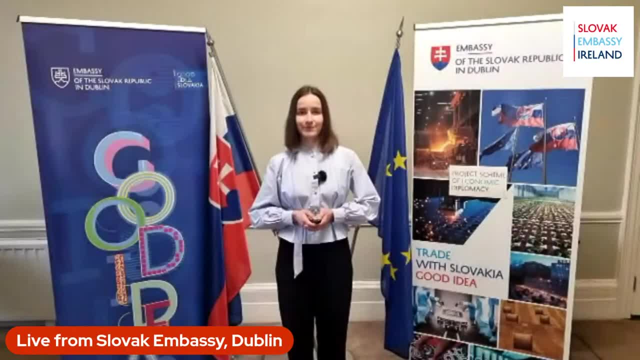 and the last presenter for today is mr yura yakubik from the slovak company natures. natura specialize in the development, research and production of natural polysaccharide and fungal beta glucan. natures is the market leader in the czech and slovak republic beta. 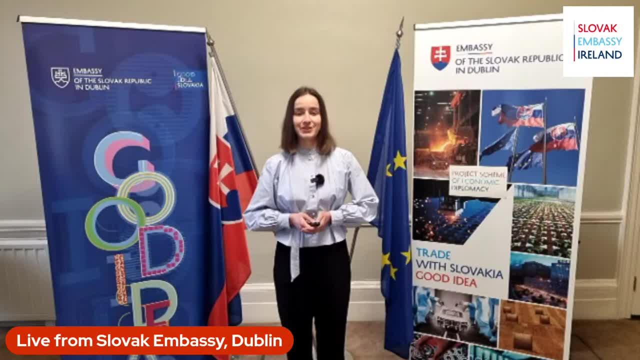 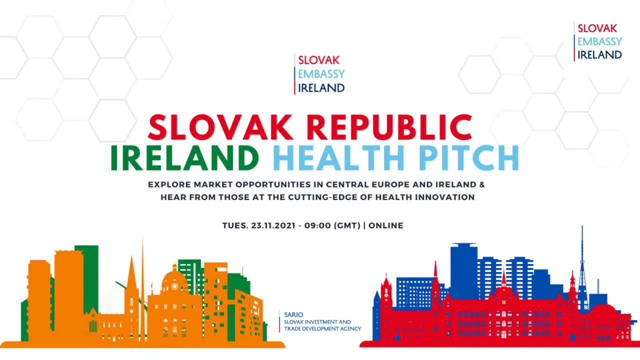 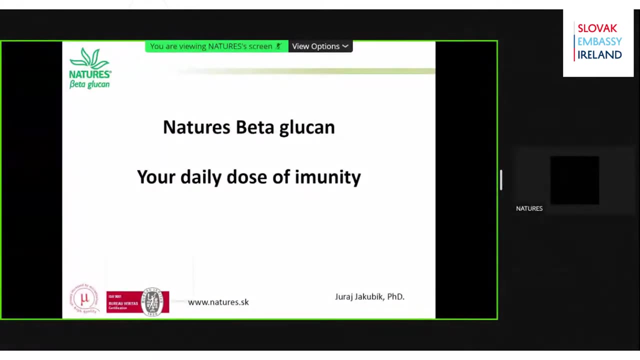 glucan. support to the immune system is ensured by a change in the activity of immune cells. thanks everybody, hope you can hear me and see. see my view and my screen. my name is yura yakubik, work for company natures and our main business is beta glucan and supporting the immune system. 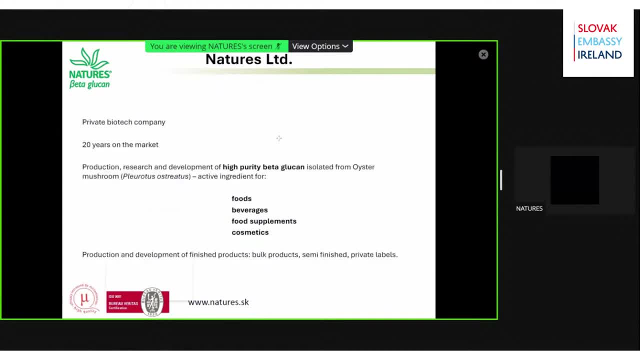 company natures has been on the market or for 20 years. we have celebrated 20 years this year. it's a small, private, family-owned company and our main main product is a high purity beta glucan isolated from oyster mushroom, and we concentrate on the production, research and development of the product as an 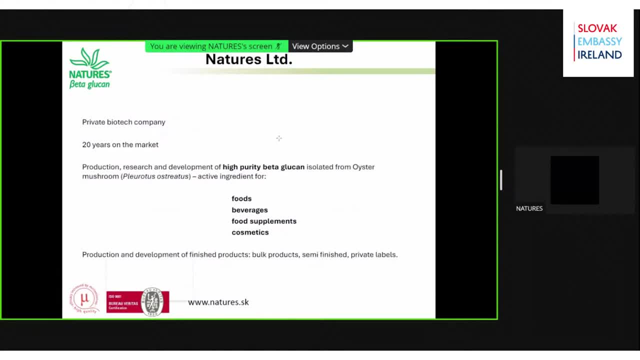 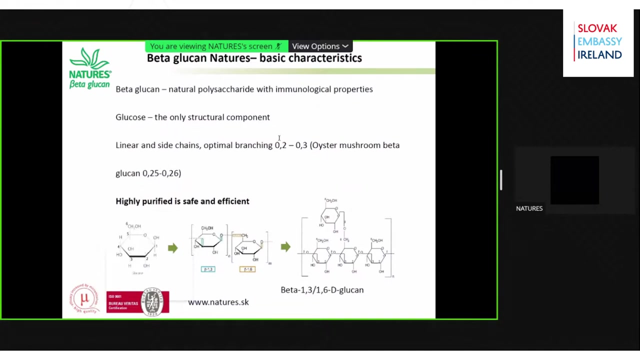 active ingredient for nutraceuticals, food supplements, cosmetics, foods, beverages and so on, and we also produce- and we help our partners to develop- finished product, either as a bulk product, semi-finished products or finished products ready for market. beta glucan is a natural polysaccharide with immunological properties with only structural 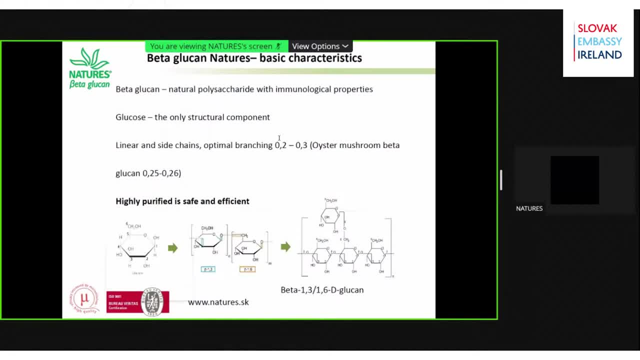 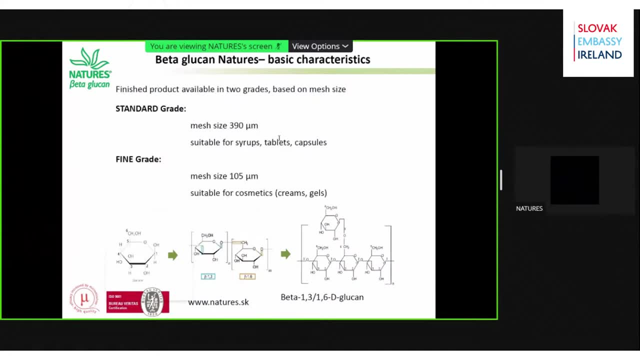 component glucose. it's a safe and non-toxic product. if highly purified, it's very efficient. the active ingredient, the beta glucan, we can offer in two grades: on the mesh size and based on the on the intended use of the of the customer standard grade is: 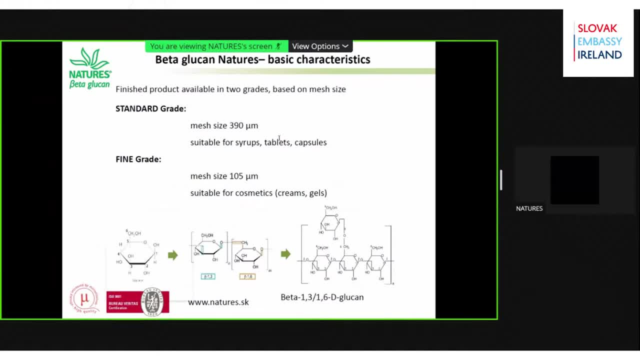 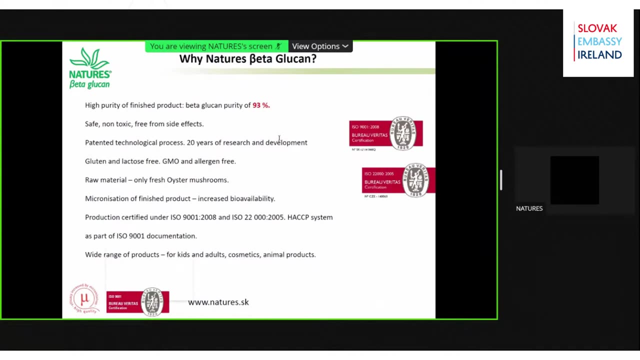 mainly for for syrups, tablets and capsules, and fine grade, which is very, very fine powder, is suitable for cosmetics, either creams, gels and so on. our main description, or my main characteristics of the product is that our beta glucan is very pure- we achieve purity of 93 percent, is safe, non-toxic. it has no side effects as far as 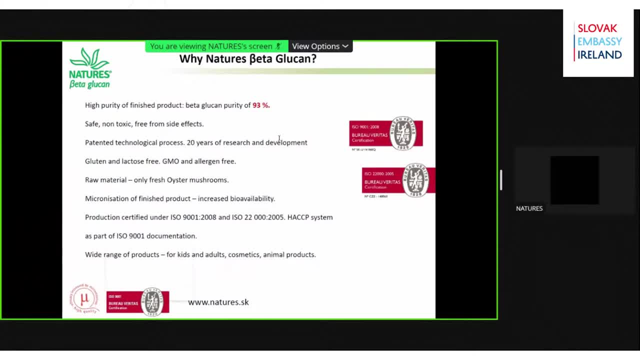 our 20 years of experience has proven. the raw material we use is fresh oyster mushroom and the whole production we have here in syrups and capsules is very, very good. the product range in slovakia is certified under iso 9001 and iso 22 000 with the hasap system. 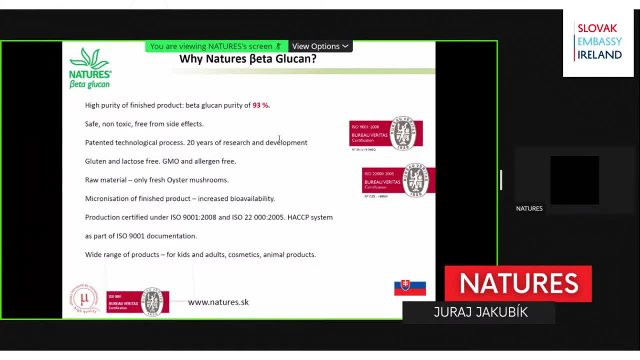 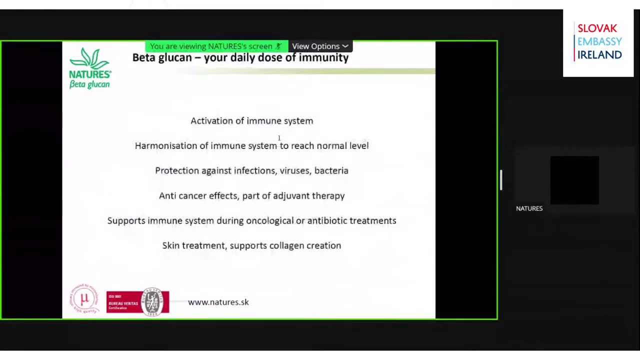 incorporated into into these two documentations. uh. the product ranges from from kids tablets for kids, syrups, uh tablets for adults, or cause or capsules for adults. we have cosmetic products, animal products and so on. the main reason we we work with the beta glucan is to activate. 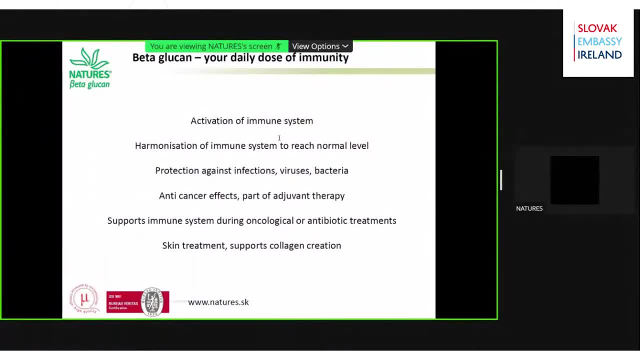 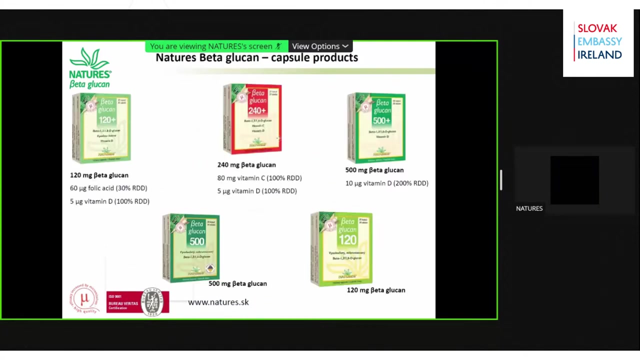 the immune system to promote the health to patients. beta glucan protects against infections, viruses, bacteria or any any health problem. it has proven anti-cancer effects and, in japanese, part of an adjuvant therapy in oncological patients. and, as i mentioned earlier, the the products are either a hard product. 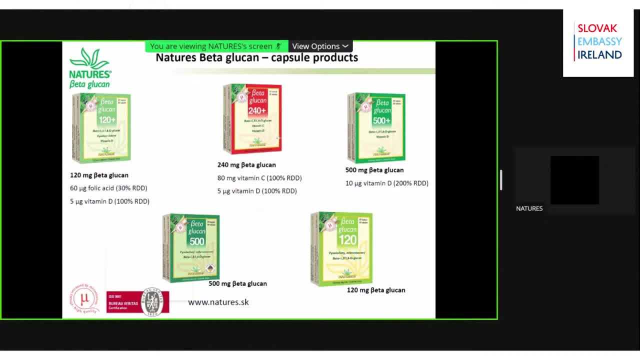 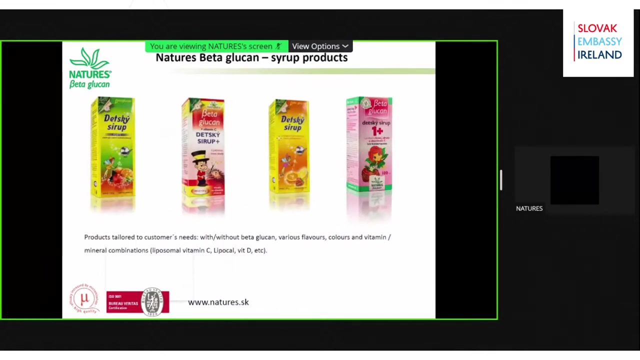 or for oral use, either capsules or tablets, with the various dosage of beta glucan and a combination of vitamins, depending on what the customer wants or what the customer needs. and there are several products, uh, orientated for kids or for small patients, which are syrups. uh, the picture shows. 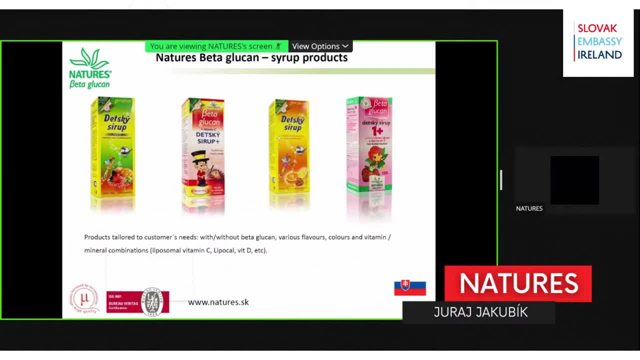 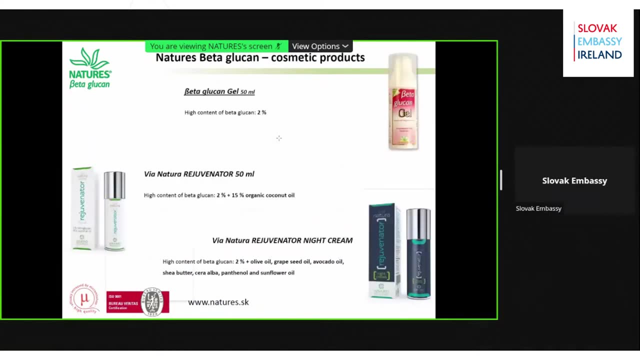 only four products, but at the moment we have over 20 different syrup products for kids with various dosage of beta group and various combinations of vitamins or minerals. and the last group of our finished products is a cosmetic, and all the cosmetics contain beta glucan in concentration of two percent. 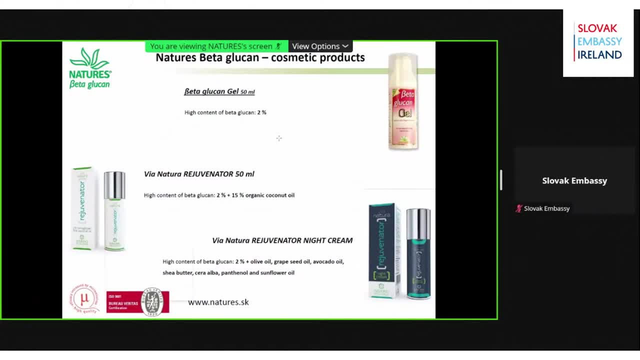 and there are several products we have with different combinations of natural oils, either coconut oil or the latest product which we have developed and put on the market this year, which is night queen. it has a combination of olive oil, grapeseed oil, avocado oil, shea butter, pantanol and. 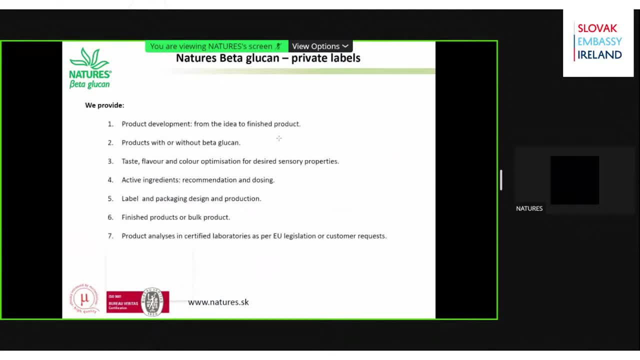 sunflower oil. uh, the products we can offer, all the services we can offer to our customers and partners is from from the basic idea of the food supplement or the cosmetic to product development. we can provide the finished products. we can provide a active ingredient, we can provide the whole. 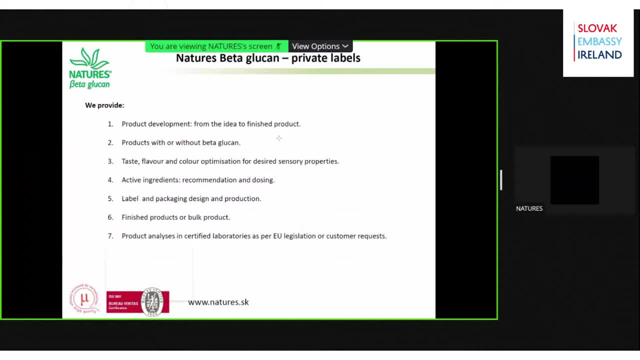 development process where we can fine-tune the taste, flavor and color of the products. we can recommend various combination of active ingredients, either being a beta glucan or combination of vitamins and minerals. all products are finally certified in laboratories. analysis are performed on on every batch, on every product, as per the either eu. 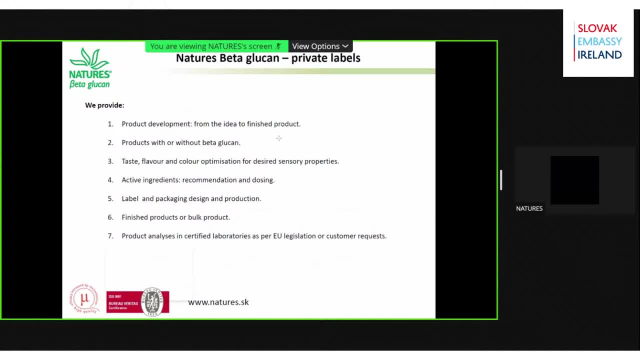 legislation or, in case of customers from outside the eu, as per the local authorities. we have partners from basically all around the world, or we have big partner in kazakhstan, azerbaijan, latvia, norway, sweden, jordan kingdom, qatar. we are starting a cooperation in in vietnam. so